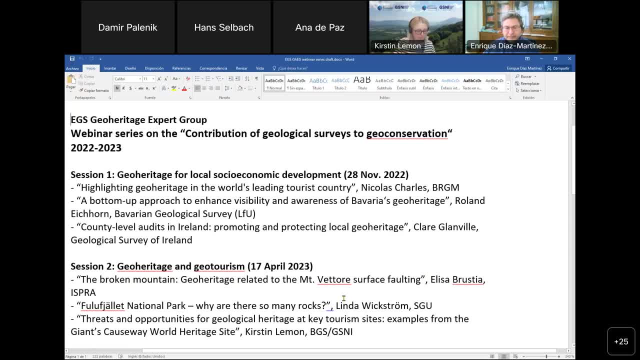 Surface 14,. then we will listen to Linda about the national park. Why are there so many rocks there? She's from the Swedish geological survey And the uh. for the last 1, we will be Kirsten lemon from the British geological survey, the geological survey of Northern Ireland. 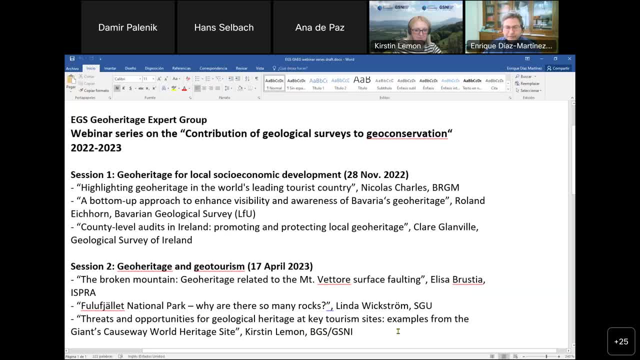 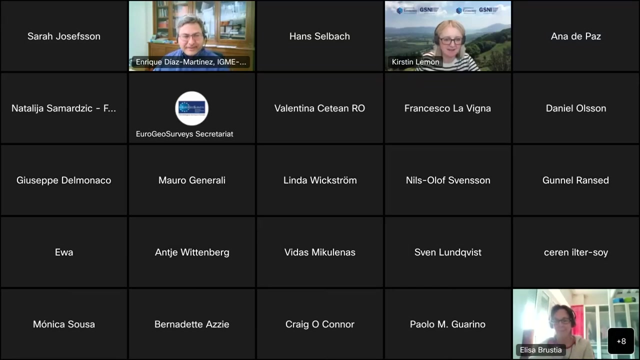 Who will be talking about the threats and opportunities for geological heritage at key tourism sites. examples from the giant causeway World heritage site. so let me, How do we go back? I don't know how to. I have to stop sharing. Okay, so everybody has seen the, the program and we will 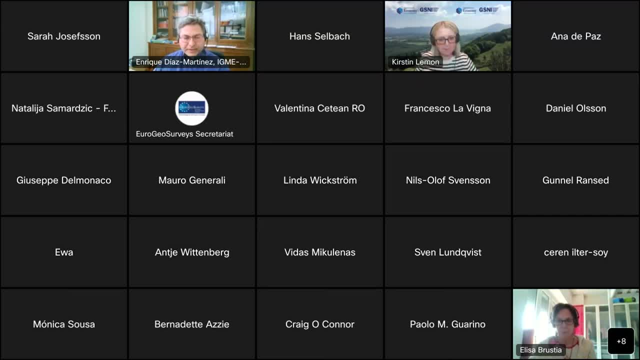 Start right away, maybe one uh, Vegas is already asking for: Is there a problem? can you hear me? I think it was just a accident. Okay, so then we will start right away, So we can uh Optimize it. 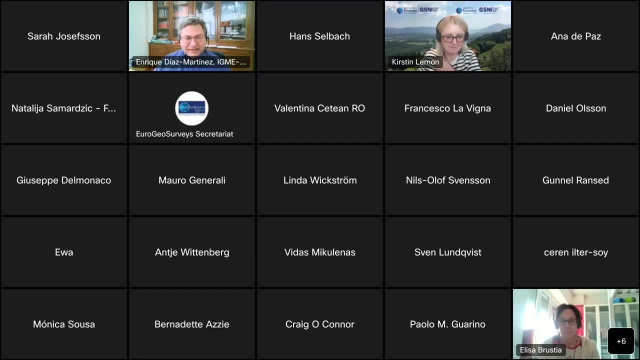 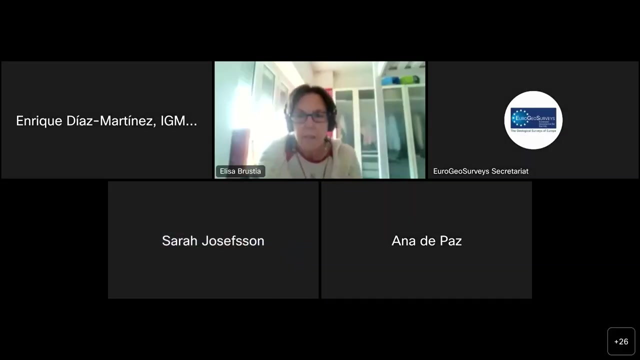 So 1st will be Elisa talking about the broken mountain related to this surface for thing. You can go ahead, Elisa, and I share my screen. Please can you see my screen? It's coming. okay, now we can see it. 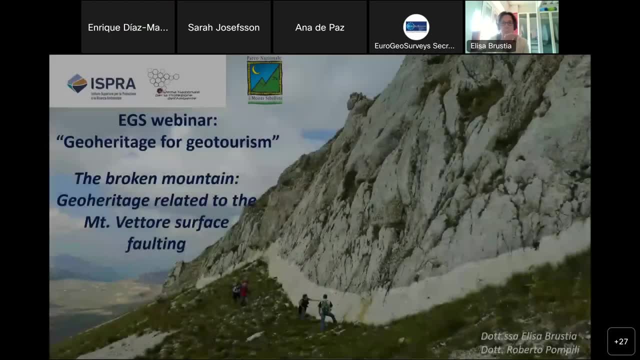 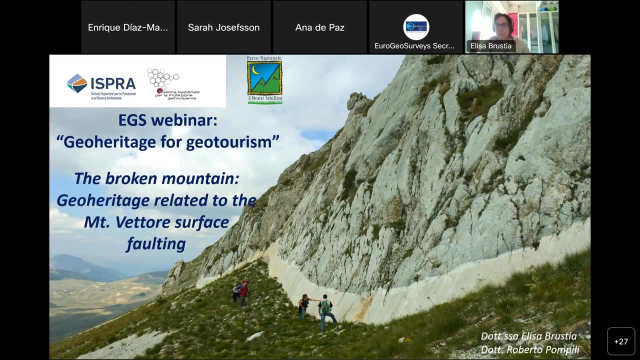 you will have to start the presentation. yes, okay, okay, there we are, thank you, um, i am elisa brustia, from ispra geological service of italy, and i'm going to introduce a project focused on the 2016 central italy earthquakes of phase 14 and concern enhancement and protection along the montevettore. 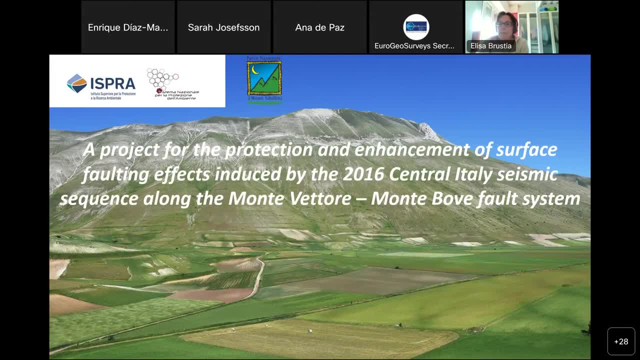 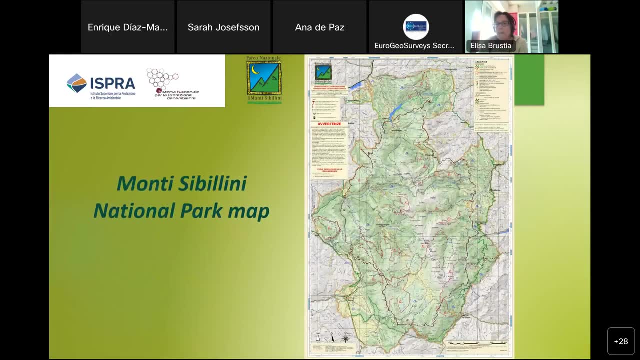 multiple food system. it is a joint project realized by ispra and montesibilini national park. montesibilini national park is a wonderful place in central up and nines, visited and and appreciated by by many tourists. there it is possible to choose several types of tourism. 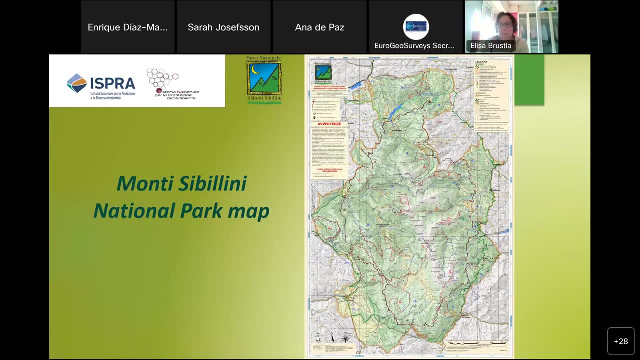 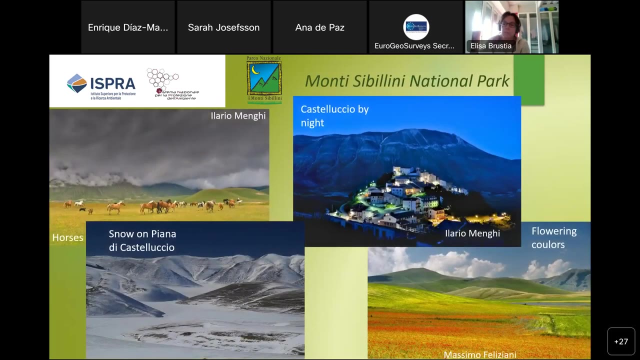 food and beverage for its ancient tradition. environmental, sports, tourism for trekking, mountain bike, riding ski, also religious and cultural. in these photos are shown some sibillini's landscapes. as you know, starting on 24th august 2016, a wide sector of central italy including including sibillini. sibillini's. area was hit by a sequence of earthquakes that started with the magnitude 6.0 event with epicenter in a coolie culminate and culminated with the magnitude 5- 6.5 event with epicenter in norcia. several magnitudes more than 5.0 shocks characterized the sequence until january 2017.. 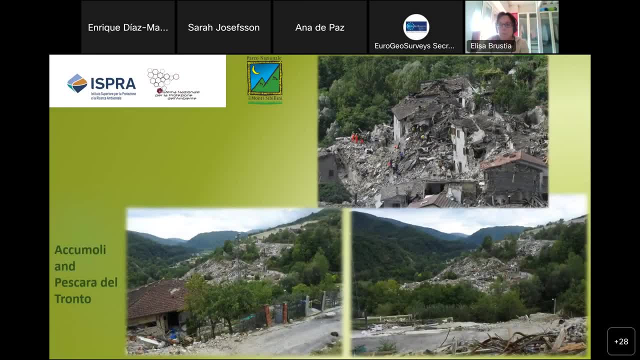 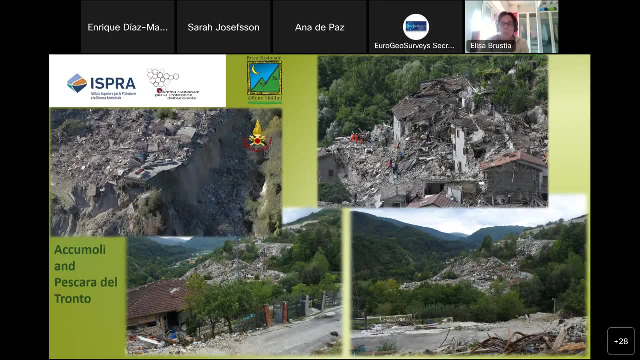 during the first shock in august, about 300 people died, mainly in the territory of amatrice and arcuata del tronto, where most buildings have been destroyed in the areas of viso usita and castle sant angelo sul nera. the highest impact was due to the 26th and 30 october event main shocks. 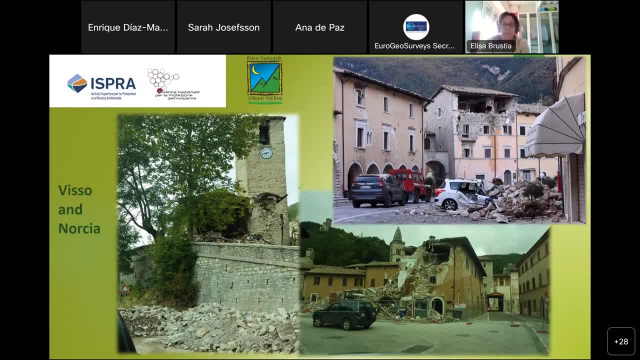 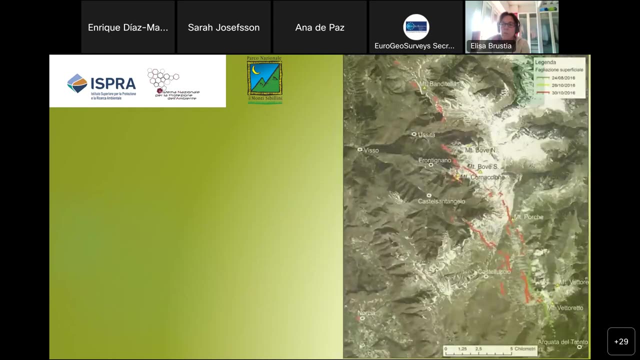 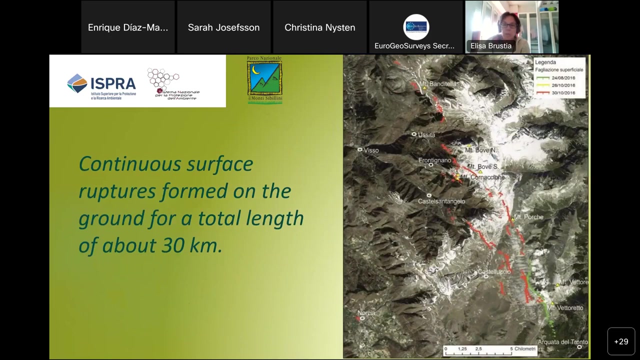 did not cause extravaganza, but destroyed a lot of buildings located in the Marche region and in some areas of Umbria, changing in a few seconds the life of many peoples. During the earthquakes, continuous surface breaking formed on the ground for a total length of about 30 km. 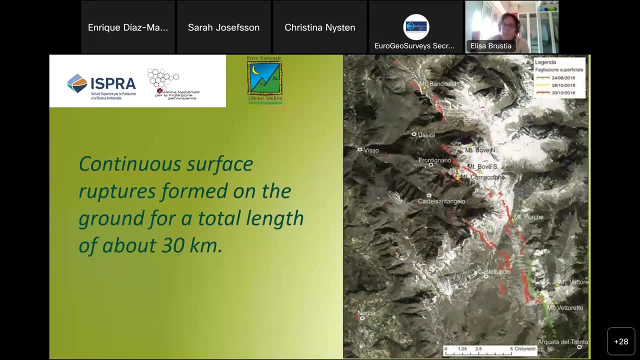 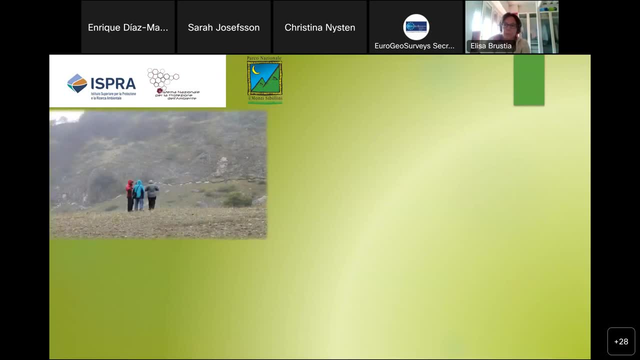 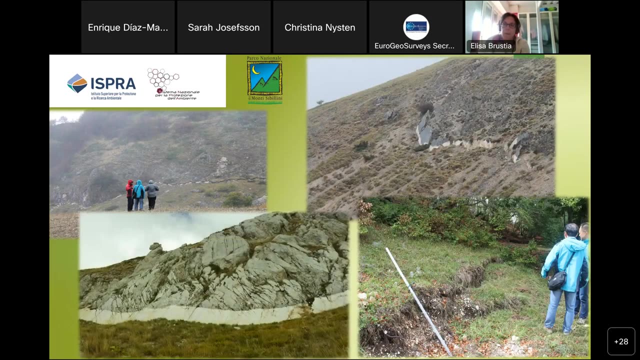 Geologists interpreted these ruptures as the seismogenetic fault. In the photos are documented some breaking interpreted as evidence of earthquake. These seismic ruptures along Montevettore-Montebove fault system represent the largest and most documented surface faulting example in Italy. 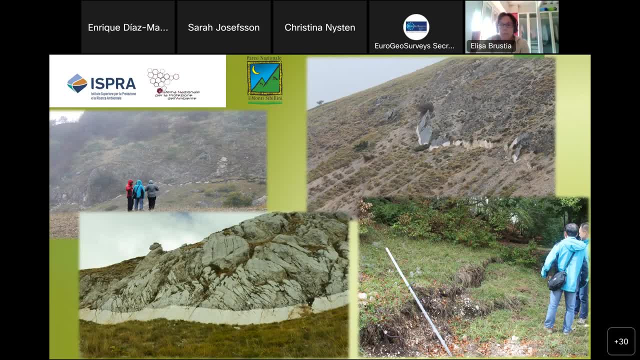 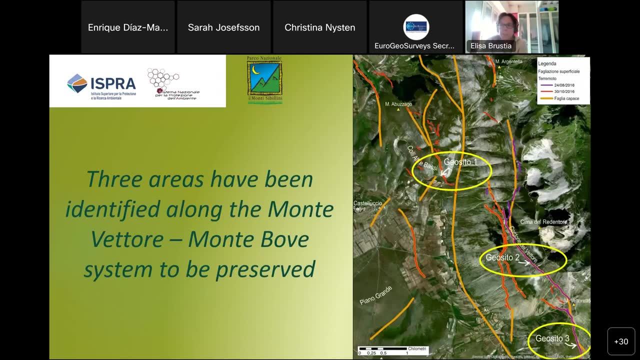 Three areas have been identified along the fault system to be preserved and to be pointed out with the aim of showing and describing this geological evidence, also at a non-specialist audience. These areas are also identified as a national geo heritage and part of national inventory of geosites. 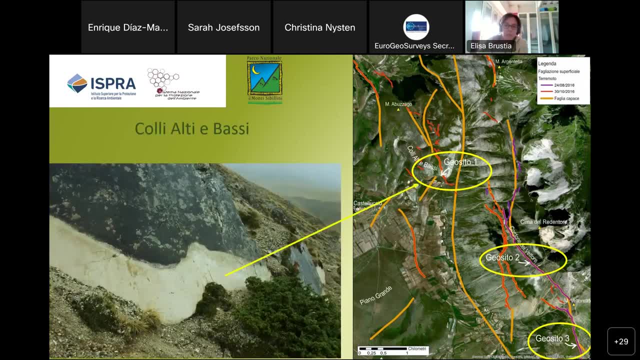 The first one is Colli Altie Bassi where Colli Altie Bassi, where the recent co-seismic rupture is marked by a white stripe at the base of the fault plane, allowing to estimate the amount of displacement in about 60 cm. 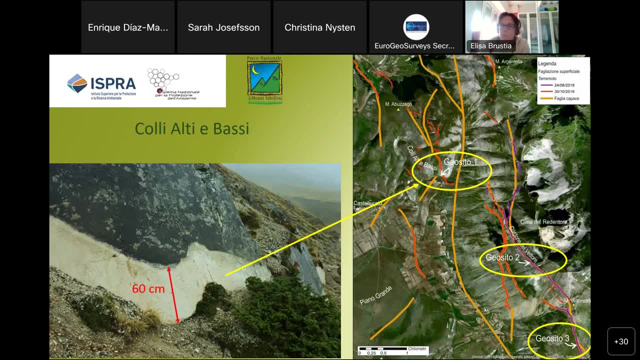 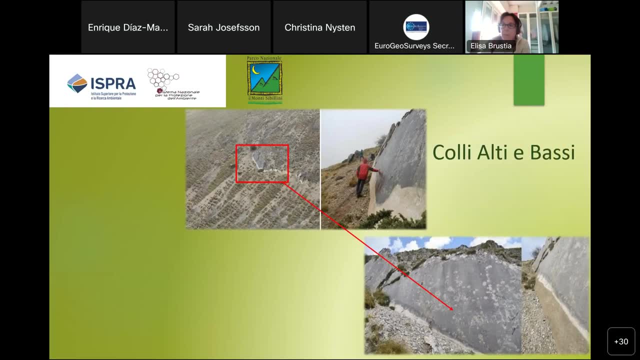 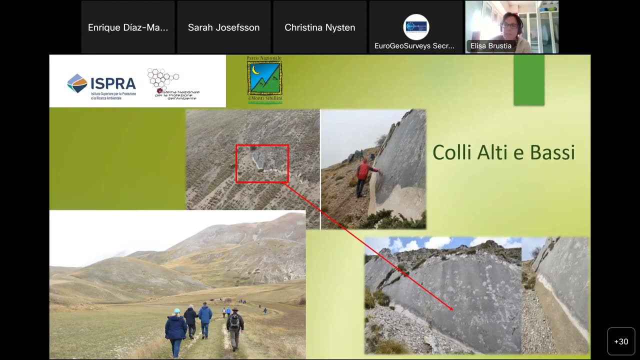 The breaking interests: mesozoic limestone and displacement. It was induced by the 30 October shock. To reach geosite it is needed to walk along a large white street for a few hundred meters from the parking near the driveway. The access is very easy. 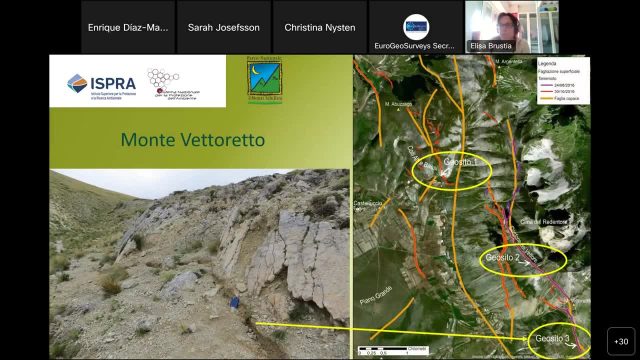 The second one- the southern one is Montevettoretto- is along an erosional gully in the southern slope of the mount. It shows a total displacement of about 70 cm. The rift interests mesozoic limestone, but his hinging wall is characterized by debris due to the presence of the little valley. 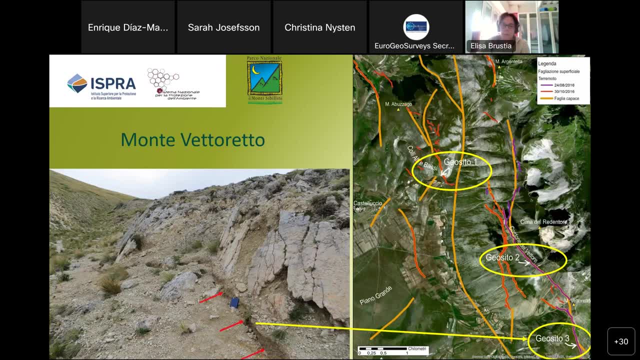 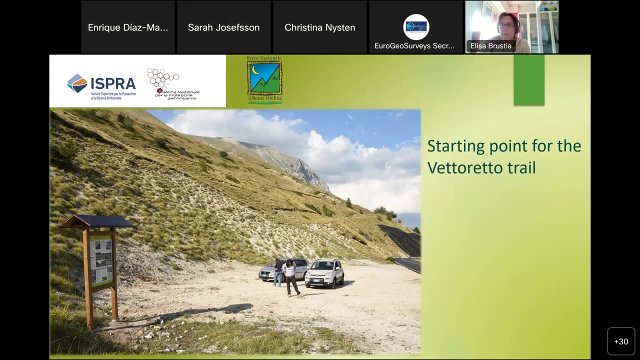 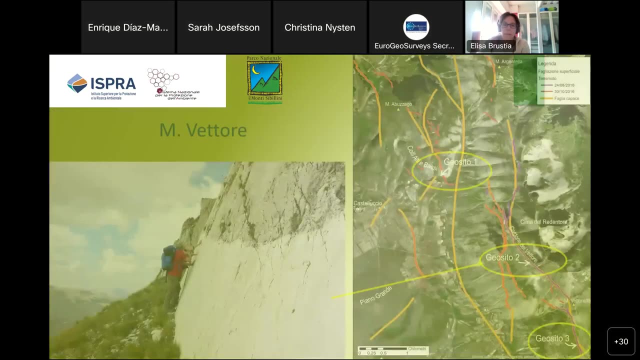 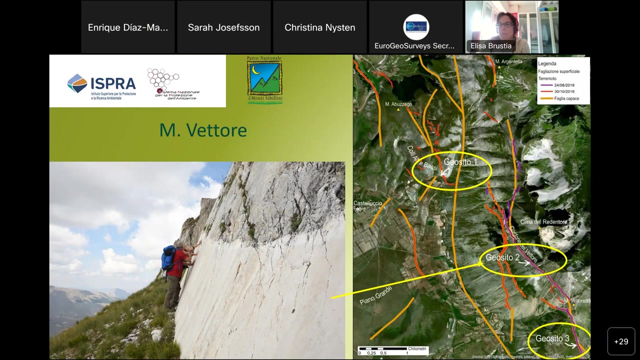 The access is easy. There is a small path indicated by a panel located along the principal driveway. The last one, and the most important, is Cordone del Vettore fault scar, where it is possible to observe a total amount of displacement of about 2 meters high. 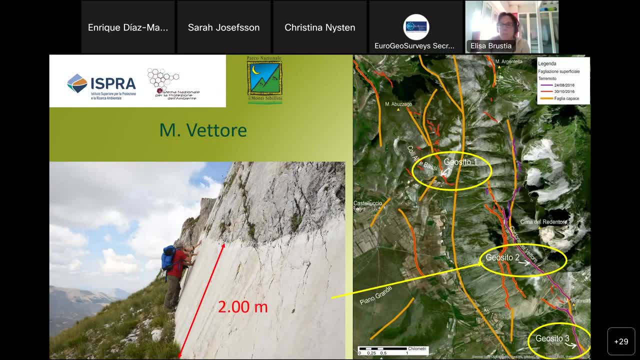 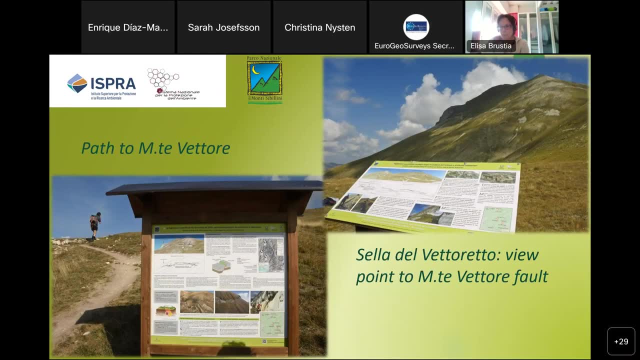 The fault breaks mesozoic limestone. A panel at the beginning of the path indicates the access, but in one and a half to two hours it is possible to arrive at the site. The path to arrive at Sella del Vettore. 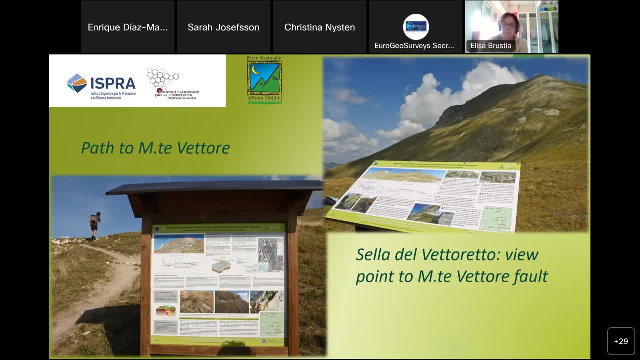 where it is possible to observe the Monte del Vettore big displacement described and represented in a panel. The path to arrive, to reach the surface faulting, is unofficial, It is long and dangerous and it is not recommended to go. The goals of the project are two. 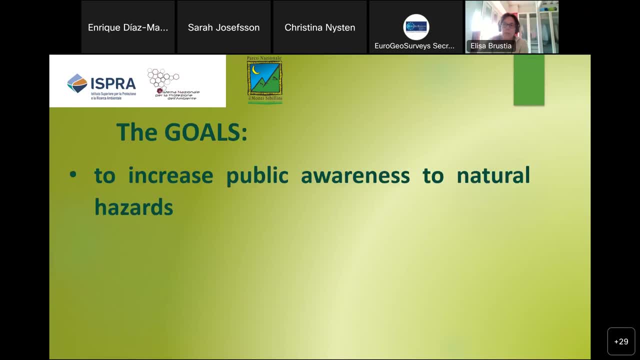 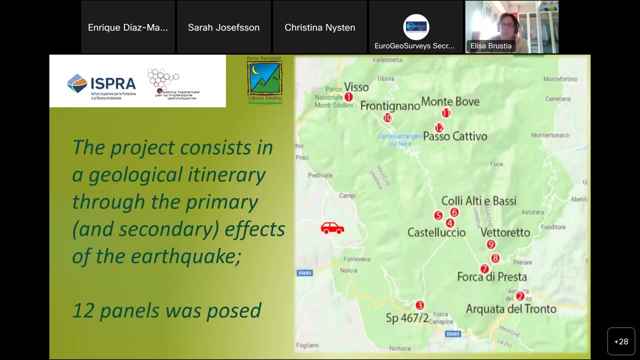 First, to increase public hours and second, to reduce the risk of natural hazards. and third, to keep the memory of the event through the announcement of the identified sites. The project consists of a geological itinerary marked by 12 spots where information boards illustrate surface faulting phenomena. 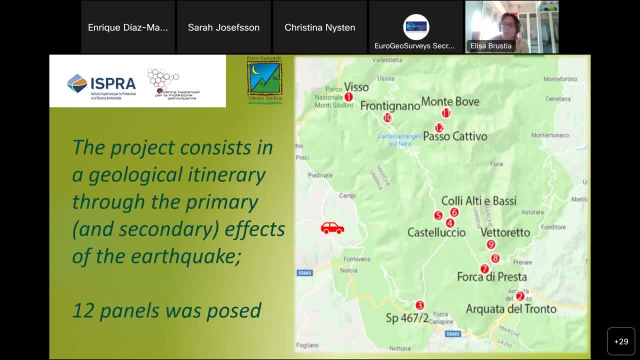 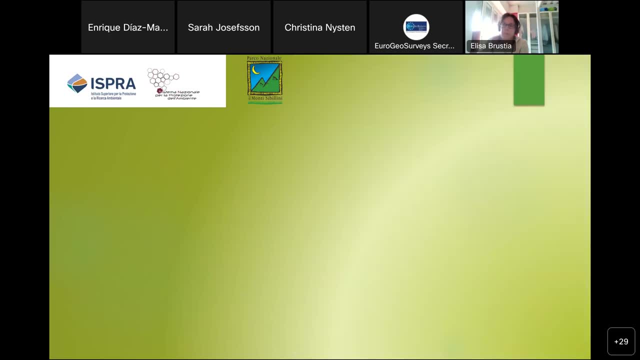 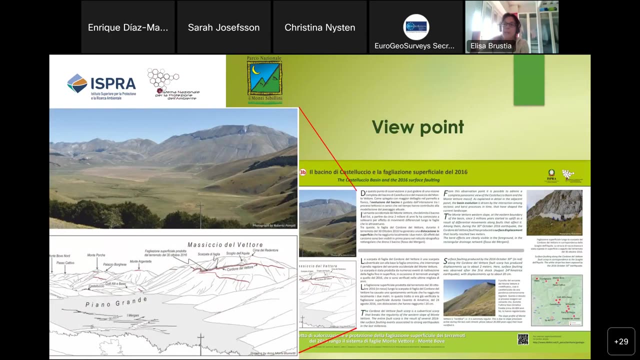 and other ground effects induced by the 2016 earthquake. The panels are in viewpoints where it is possible to observe the geological context, helped by line drawing and scheme. Other panels are located in parking areas near roads to indicate the pedestrian path to reach the geosites. 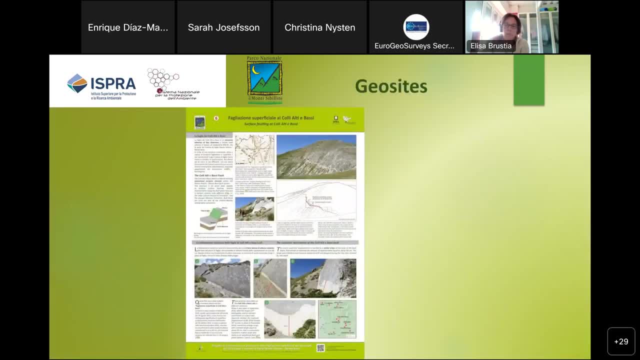 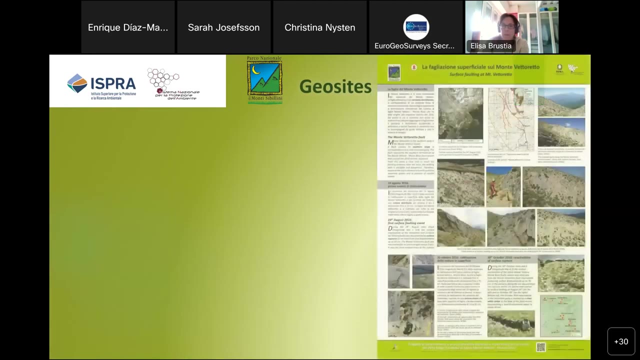 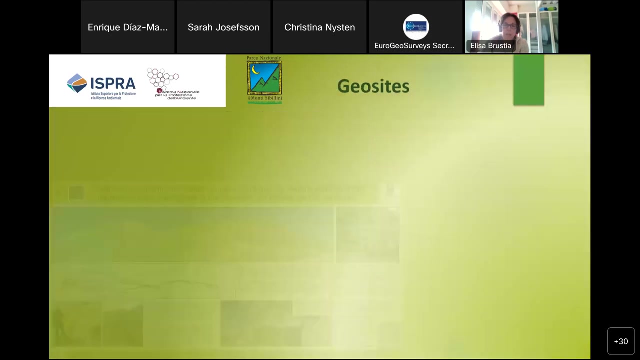 Others are just close to geosites we have yet seen, For example, Colli Altiebassi, with more information about reactivation and tectonic elements. This is Monte Vettoretto and the big one, Cordone del Vettore. 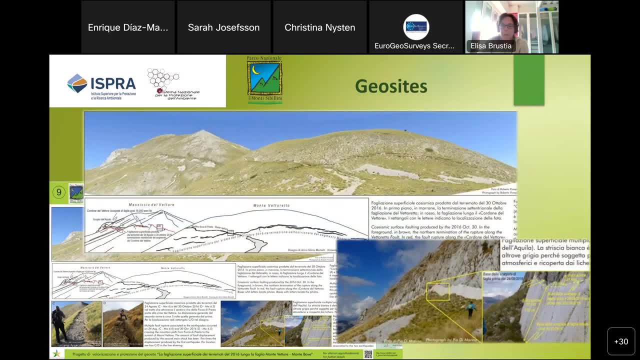 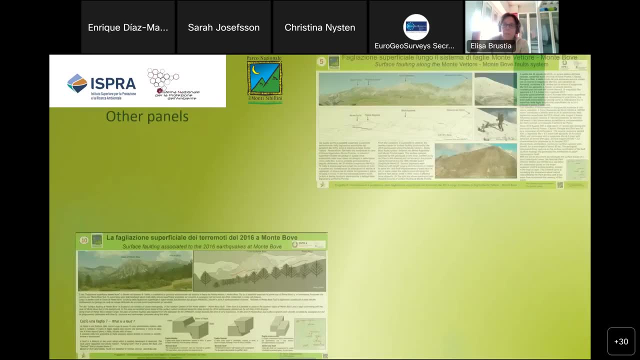 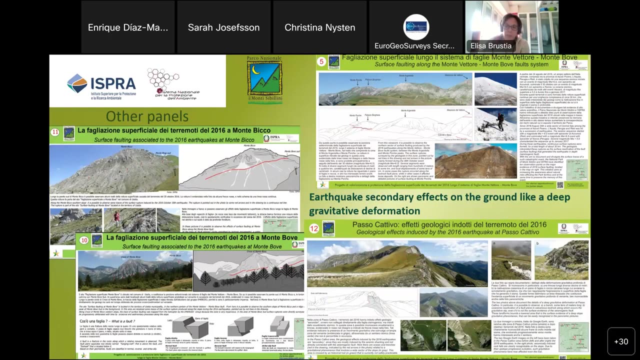 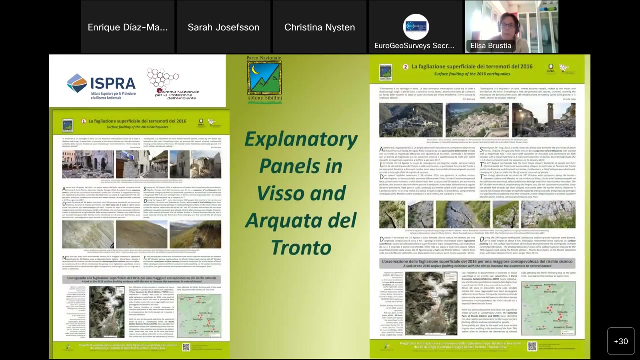 with line drawing and details. Other sites represented earthquakes with secondary effects on the ground like a deep gravitative deformation. for example, in Passo Cattivo, as the bottom right, Two introductive panels in Visso and in Arquata del Tronto. 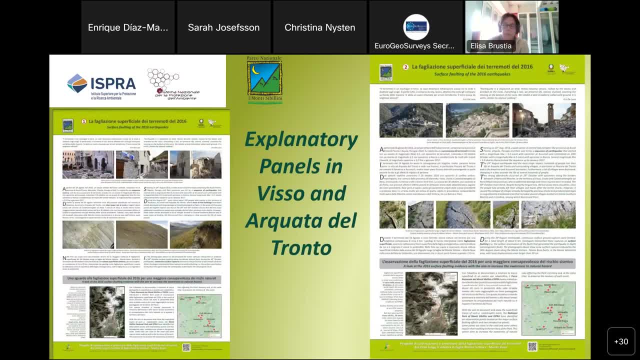 at the gates of the park commemorating the victims of the tragedy and introduce the visitors to join the geological itinerary. The people interested in learning more about the 2016 earthquake will be able to access directly from their smartphone to further multimedia web resources. 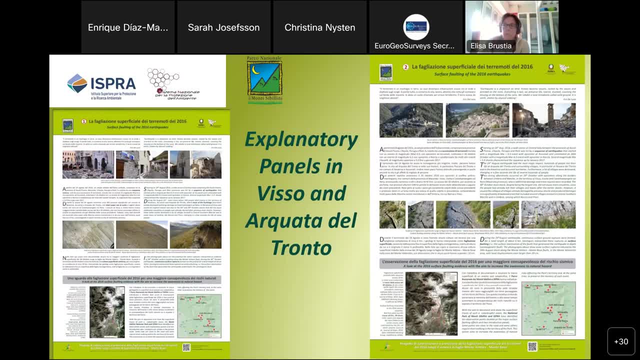 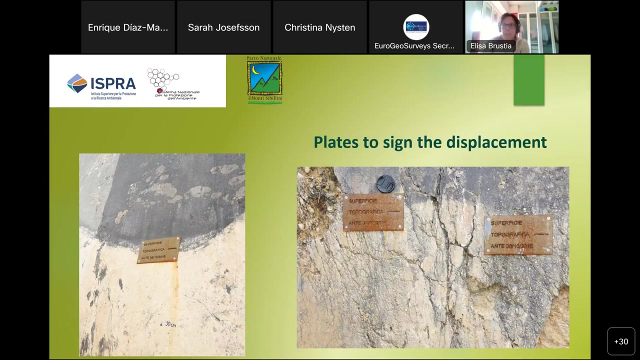 like video and papers through a QR code in every panel. The project also includes some protection works against weathering on default mirrors with special protective resins. furthermore, metal plates were posed to indicate the entity of displacement In order to complete the project. 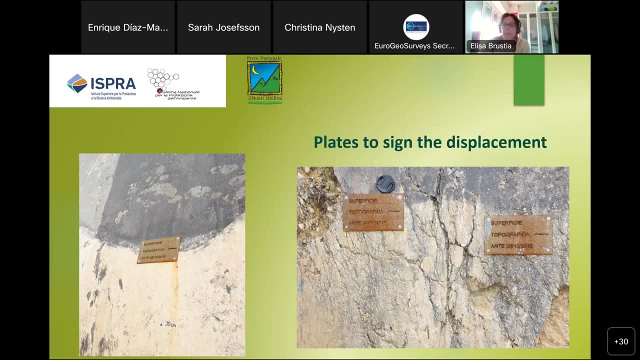 a training course for park guides was organized by ISPRA and his specialists. The course was about the geological itinerary, geoheritage and seismic hazard In November 2021, when the technical activities finished and the difficulties associated with the pandemic period improved. 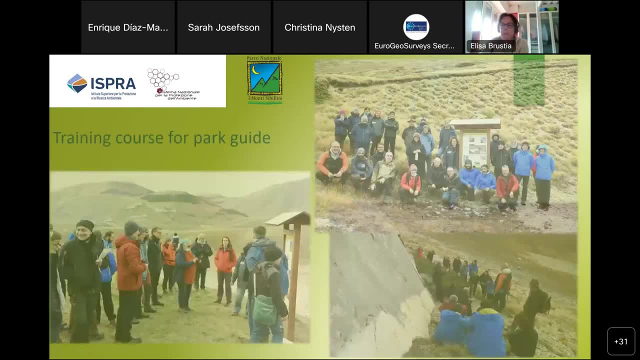 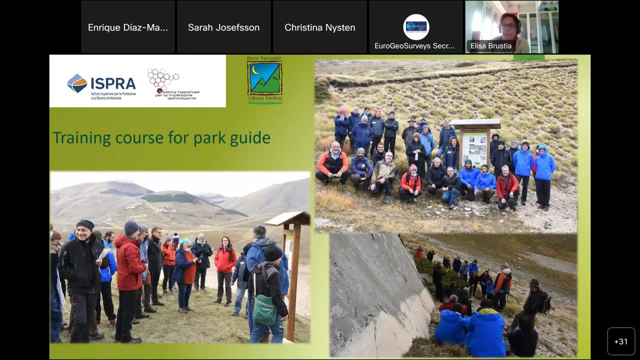 today's course was organized. On the first day, the lessons were held online and the next day, a field trip. lessons were done. 2016-17. Central Italy. earthquakes, as well as causing many death and destruction, represents a deep and painful wound. 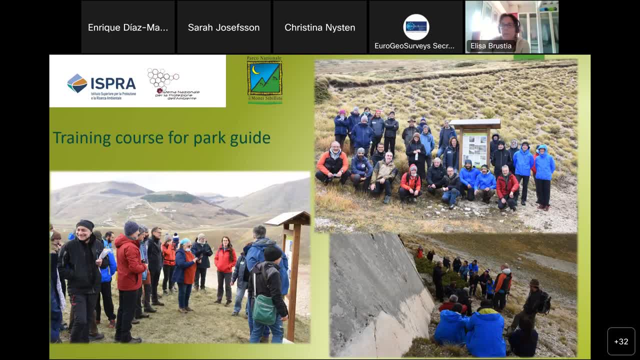 Close to technical activities. the project expects some meetings with local people to inform them about the project activities and to raise their interest in Vettore geosites, an asset they own, In this case, the relationship between the geosites. 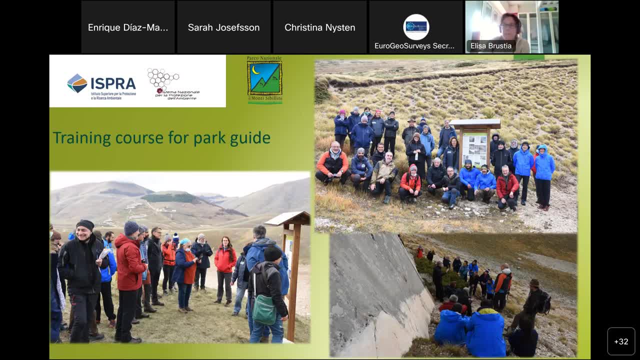 and the recent tragedy is still too much felt. so to respect for their sensibility was good, to get on carefully. Also, the difficulties created by the pandemic changed the times of activities and in this moment we still haven't done a meeting. 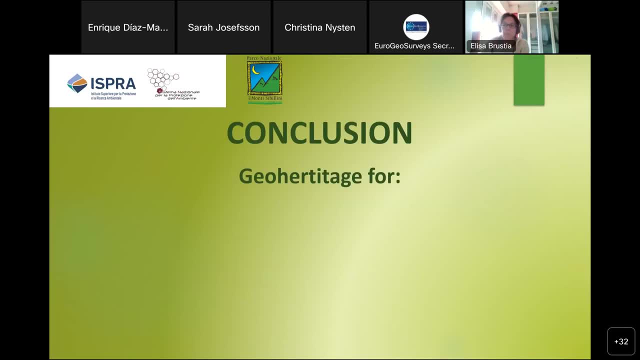 In conclusion, the local people trust in tourism, important to recover from disaster and the recent COVID period. We think geo-heritage is a richness every day more known and appreciated, not only for scientific reasons but also for cultural tourism, whose pillars are: 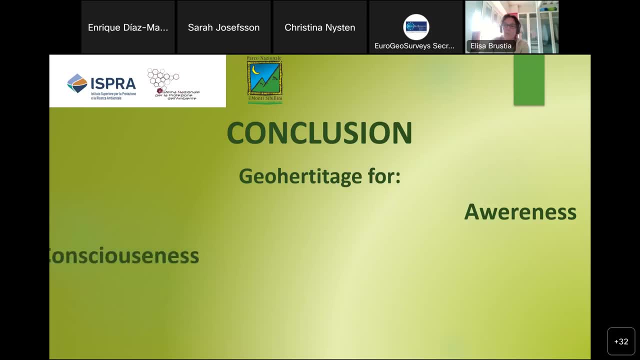 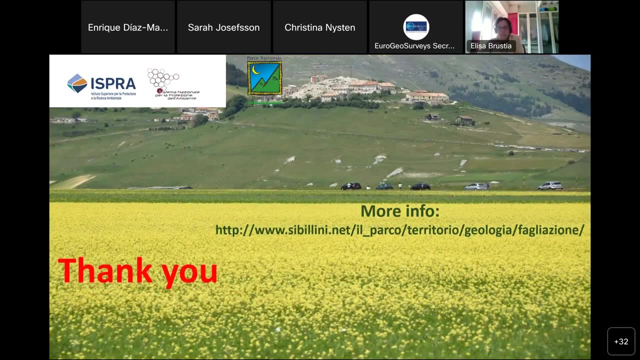 awareness in natural processes, consciousness and respect. Thanks all thanks for the attention. Other info: you can see the site of Sibillini of Monte Sibillini. Thank you very much, Elisa. I think the best will be. 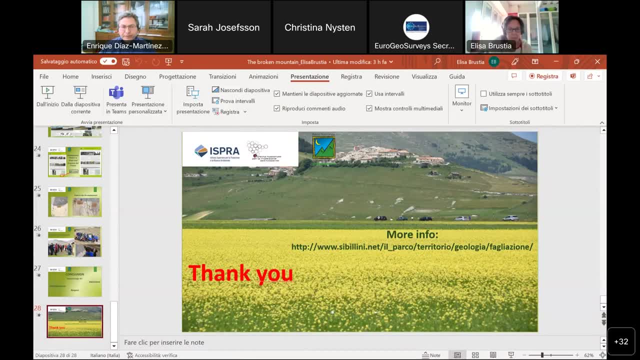 if we continue with all three. Thank you for keeping to the time and then we will get the questions or in general. I hope that is okay. We already have 37 participants. Thank you all for attending our webinar and we will go now into the next presentation. 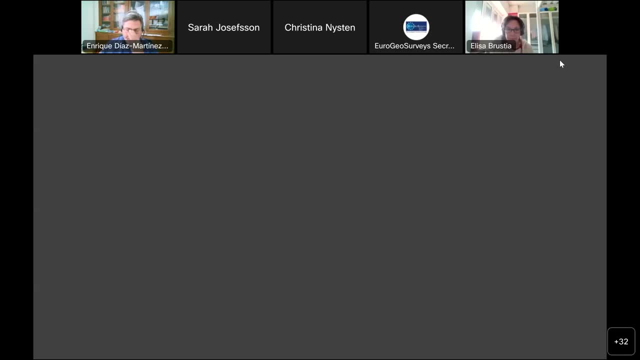 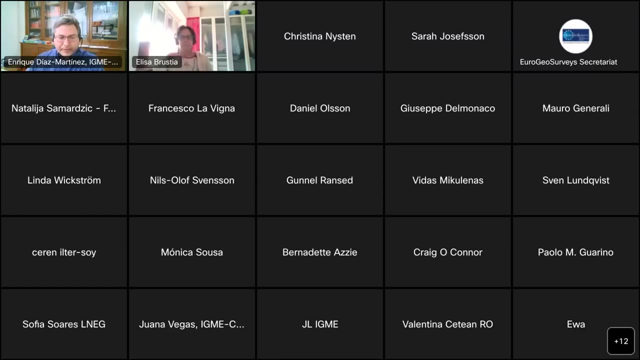 That is Linda Wikström from the Swedish Geological Survey. We'll talk about the Fulufjallet National Park. and why are there so many rocks? Thank you, Linda. Linda, She's attempting to share. Okay, Now we are seeing it. 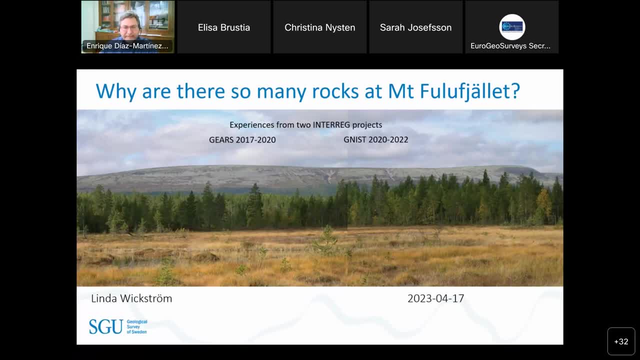 Good, Thank you. You have your microphone. We don't hear you. Oh, We don't hear you yet. Hello, Do you hear me now? Okay, Yes, Linda, Okay Good, It was the headset this time, Okay. 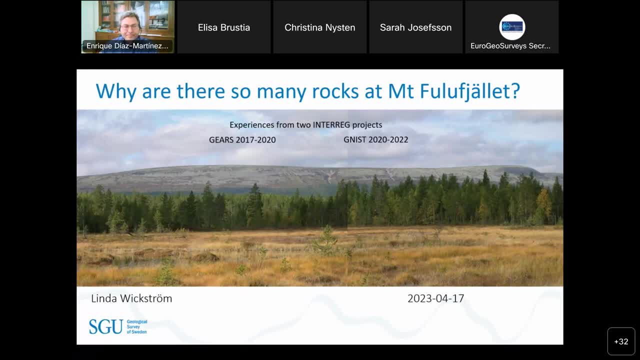 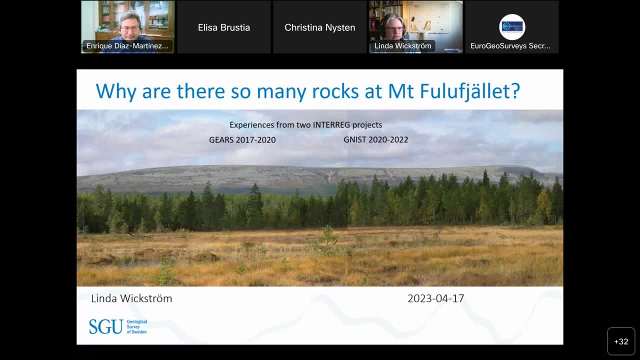 and I'm a geologist at the Geological Survey of Sweden and have been working with Geoheritage and Geotourism for like 20 years now, I think, And I'm going to talk about some experiences that we've had during two interreg projects. 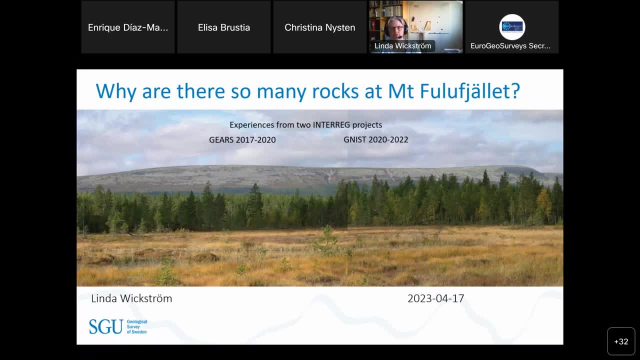 we've had, together with the Norwegian, the norwegian geological survey, um. so the title of this, of this talk, is: why are there so many rocks at mount hulu fjellet? because that is what the visitors wants to know. why- and these interact projects. they lasted between gears, which is the first one lasted between 2017. 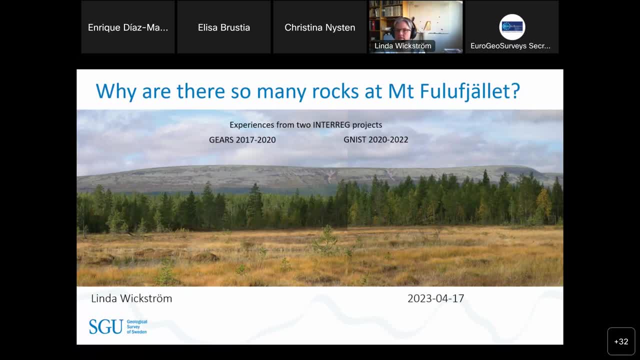 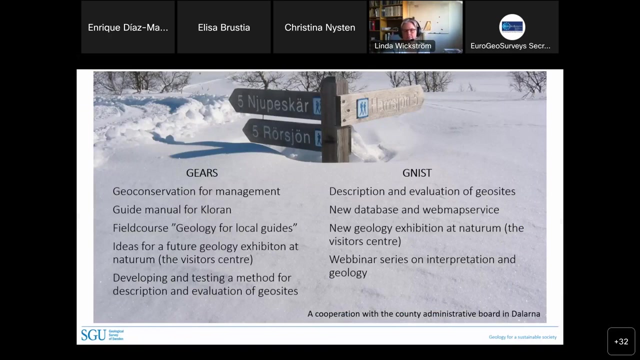 and 2020 and gnissed between 2020 and finished last year. oops, i'm just trying to get to the next slide. there we go in gears. we had some activities where we would about your conservation for management people, the people working with the nature, protection and management of protected areas. 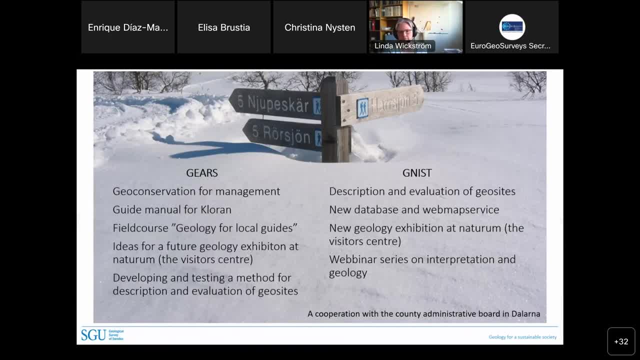 in sweden mostly. we also produced a guide manual, a geological guide manual for the national park for one of their gorges which is called cloran. we also had a small field course for the local national park which was very popular, and some of the things i will talk about in this talk is how we 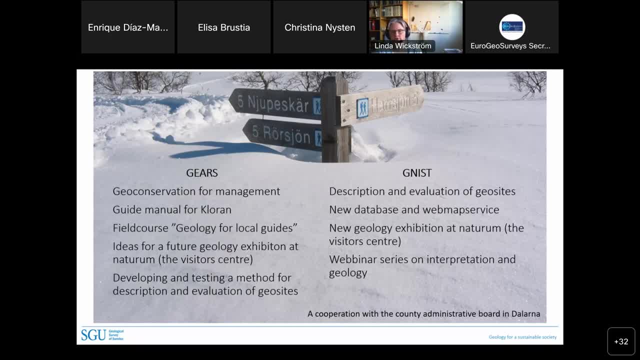 presented it to them. we also had a cooperation with the county administrative board in dalan, which was one of the partners where we helped them with ideas for their future geology exhibition at the visitor centers of the national park, and in the project we also developed and tested a method. 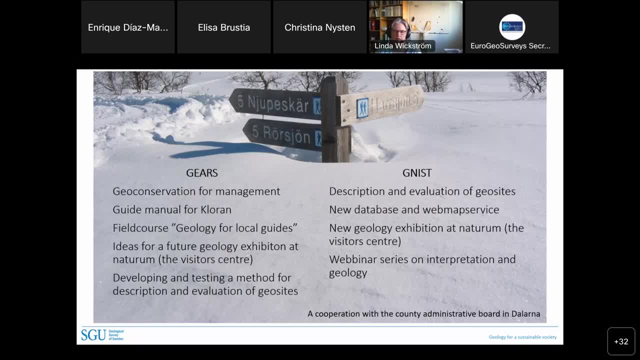 for description and evaluation of geocites together with nina and the norwegian geological survey, and it was a very successful project with many good opportunities to talk about your heritage and tourism, and all that to geologists and also non geologists in gnis. we could take this further on. 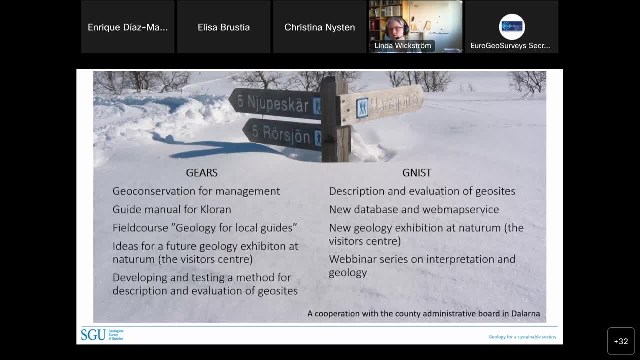 and and described and described our efforts in the geological survey which we have brought to the and evaluated a number of geosites in the area and in the surrounding area as well, And we developed actually a new database of geosites and a web map service. 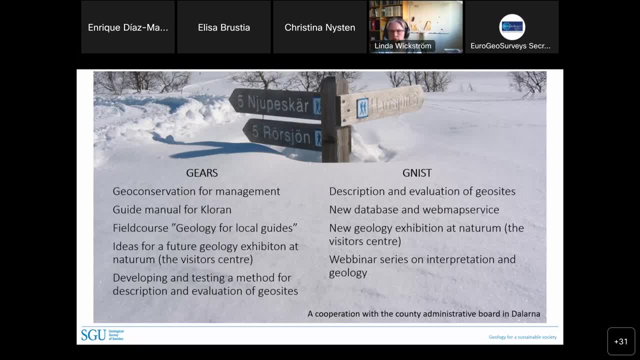 that we have together with the Norwegian Geological Survey, So you can actually see sites in both countries at the same time, And the Visitor Center at Fuglefjället also have a new geology exhibition thanks to the project, And in the project we also held a webinar series on interpretation and geology. 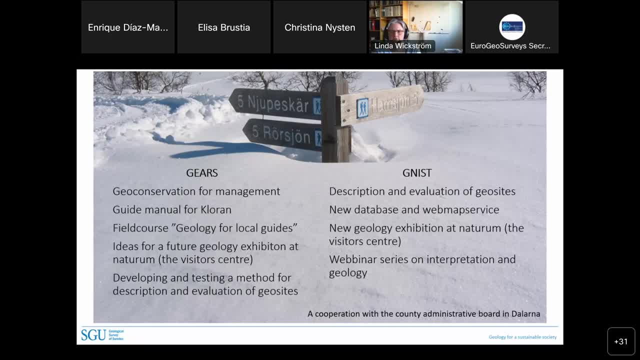 Remember that Gnist was actually a project running in the middle of COVID, So we had problems with meeting each other and seeing the tourism industry. So we had problems with meeting each other and seeing the tourism industry. We had problems with meeting each other and seeing the tourism industry. 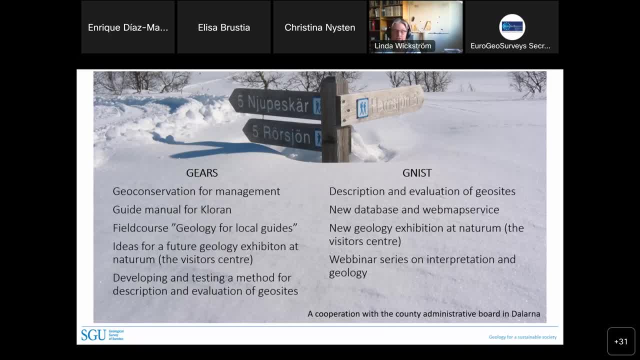 So we had a webinar series instead and it was very popular. We had about 110 people attending the seminar series in total. We had about 110 people attending the seminar series in total And people enrolled for it In general. there were like 50 people doing each occasion. 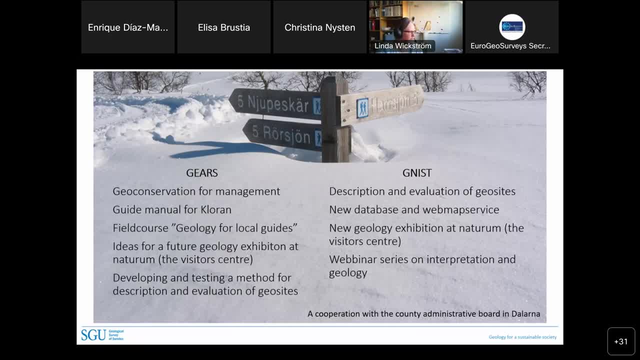 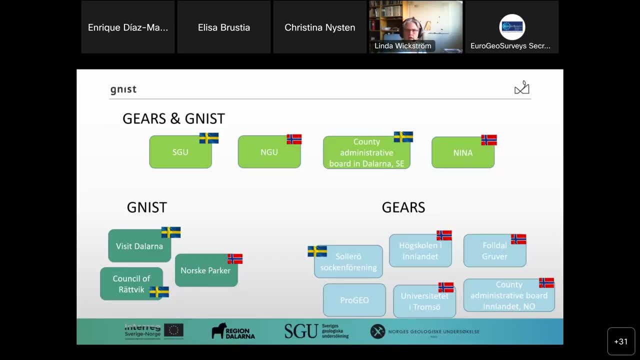 Which I have to say it was a very good number of participants. number of participants and this is just to tell you about who were in in the projects: many the green ones are the one the the organizations that that were the same in both projects. in Gnist we had some other organizations as well. Visit Dalarna, which is the 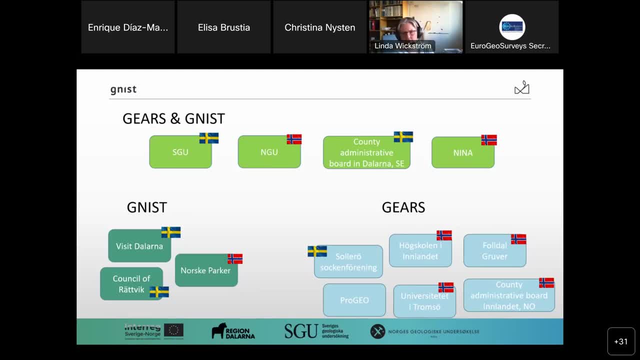 the tourism organization in Dalarna. we also had a council and an organization in Norway called Norske Parker and in Gears. we also had a few more universities: Foldal Gruver in Norway, which is a visiting mine, and the county administrative board in inlanded in Norway and a few more. 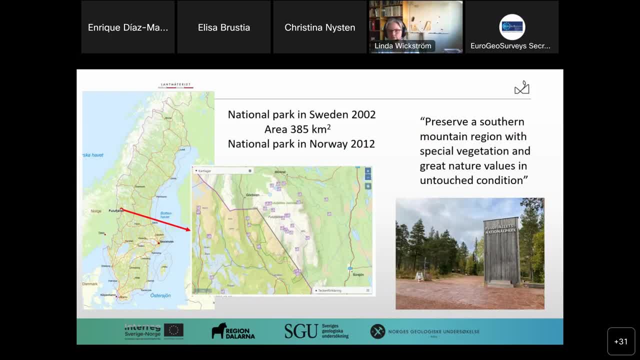 so I'm sure that most of you actually have no clue where that is and you can see on the on the map there's a red dot, which is where it is. it's in the central of Sweden, not very far north and very close to the Norwegian border, so you can actually the mountain itself is actually. 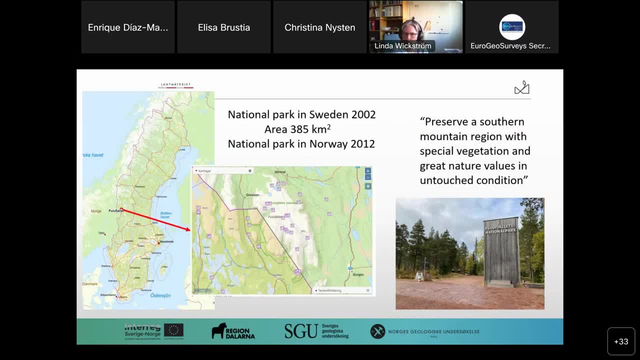 split between Sweden and Norway, so um, and it's been a national park in Sweden since 2002 and in 2012 it also became a national park in Norway. so it's it's a it's a good area for a uh, combined National Park interest. so, and it was. 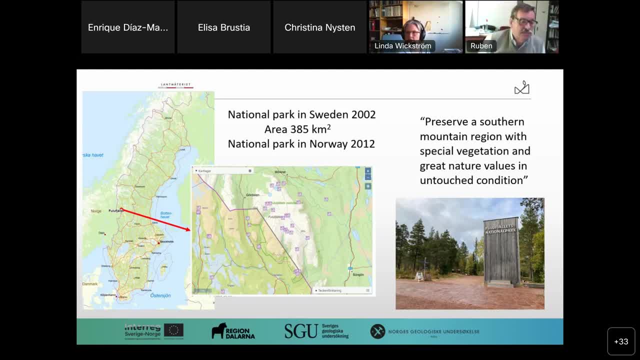 it was named a national park to preserve a southern mountain region with special vegetation and great nature values in untouched conditions. So that's the the reasons why Tullufjället became a national park on the Swedish side. So why do people go here? 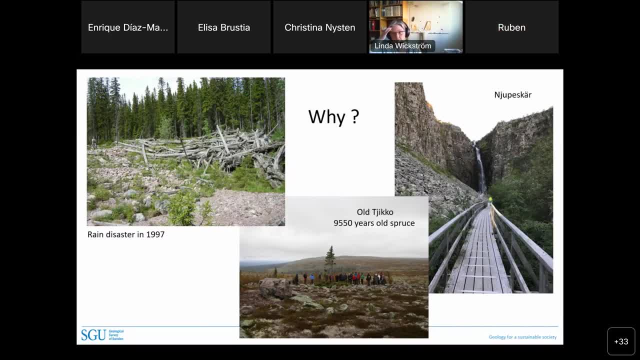 There are- it's mainly three reasons why people go to this place. First, they want to see the, the tall waterfall Njupesjär. it's 70 meters tall and is among the tallest in Sweden and quite impressive to look at. 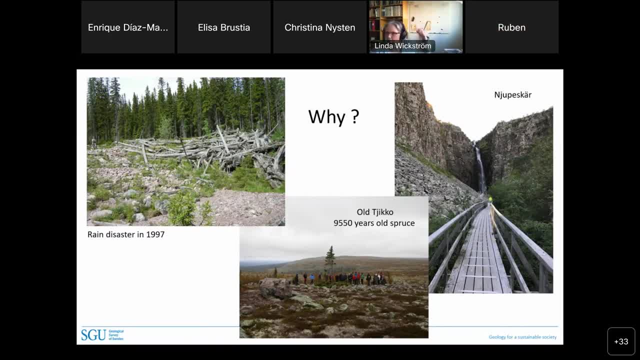 And then another reason is to see Old Ticko, which is a spruce that's 9,550 years old. So it's not the tree itself, It's the root system which is that old, So that is the oldest tree in Sweden. 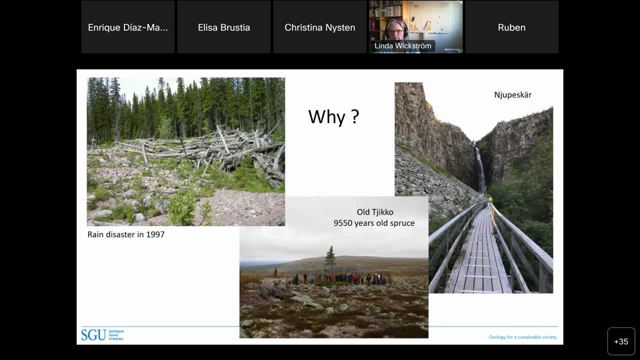 And I think it's the oldest tree in Europe or something like that. So that's what people go and look at, And they also look at the remnants of the rain disaster that happened in 1997, when 400 millimeters of rain fell during two days in a very specific spot. 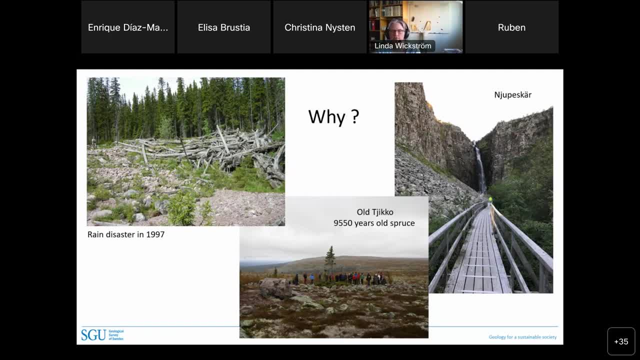 And it was a lot of water coming off the mountain- And you can see in this picture it's my- actually my colleague Gunnel- which is to the left of the of the trees, So you can get some kind of scale there- And these trees were actually standing up further up and they were all pushed down along with the water masses. 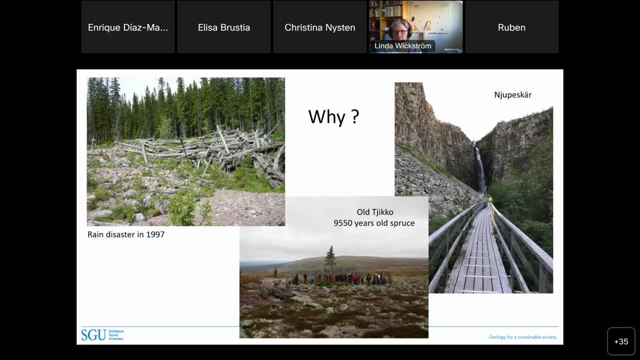 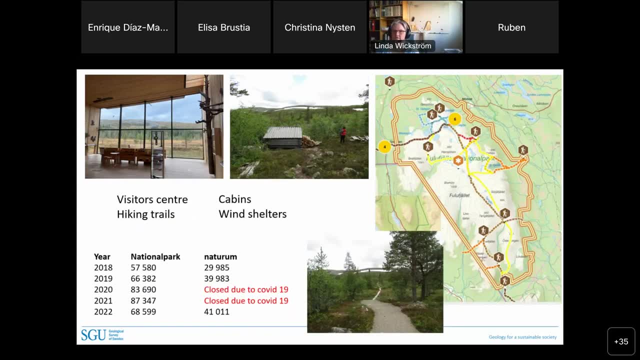 So this is mainly why people go here, mainly why people go to this part of Sweden And in the national park you have a visitor center, you have a lot of hiking trails, you have cabins where you can stay overnight, you have wind shelters where you can also stay. 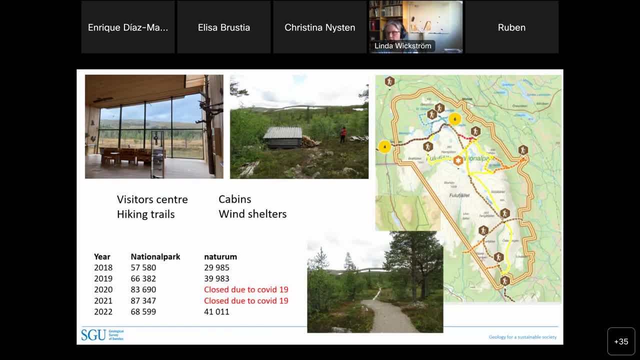 overnight that are prepared with wood so you can make a fire and take care of yourself. It's not allowed to go by bike on the mountain because then the trails and tracks will all get ruined. And I have a few numbers of visitors. During the pandemic there were 83,690 visitors and 87,300 in. 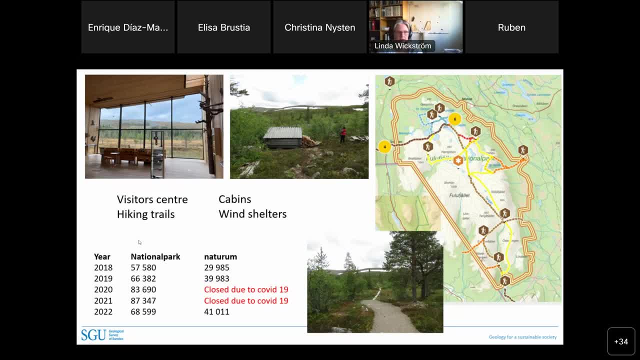 2018.. Which is really, really good, and you could see that people, when they couldn't be inside, people were actually going outside, outdoors instead, And last year the visitor numbers were down to 68,000. but it's still very, very good and 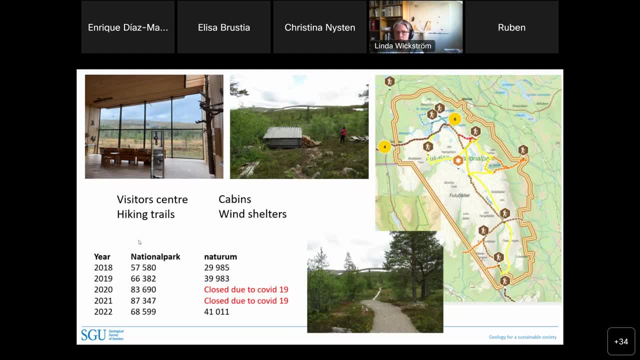 far better than the years before. And Naturum, that is the visitor center, so they have different counters, But the number of visitors have increased a lot and they have had to do some increasing the parking spaces and things like that to be able to welcome everyone that wants to go there. 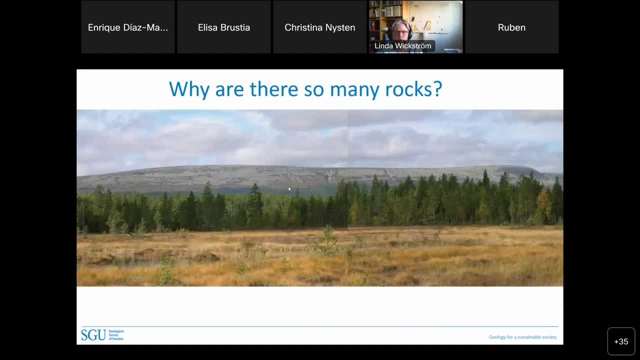 So why this question? Why are there so many rocks? That's what Sofia, which is the woman who works there. she gets this question every day from people that spin up On the mountain. Why is it so rocky? Why is it so difficult to walk and 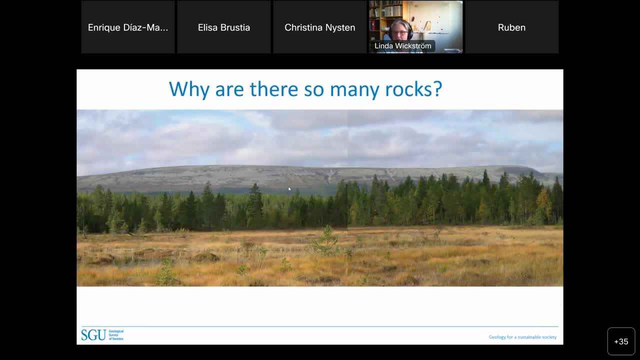 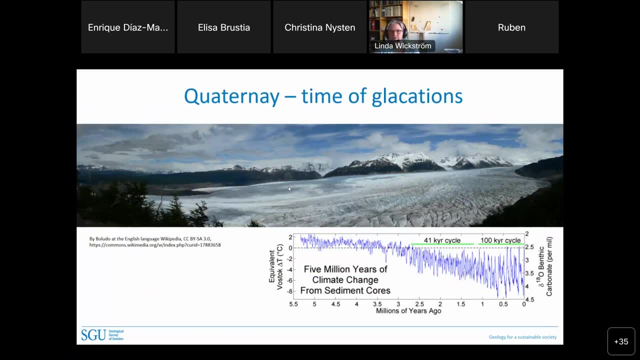 climb and so forth. So that's what we tried to help her with, And so we went back to the Quaternary and then talked about the Quaternary, which is the most recent history, And it's a time of glaciations and time of 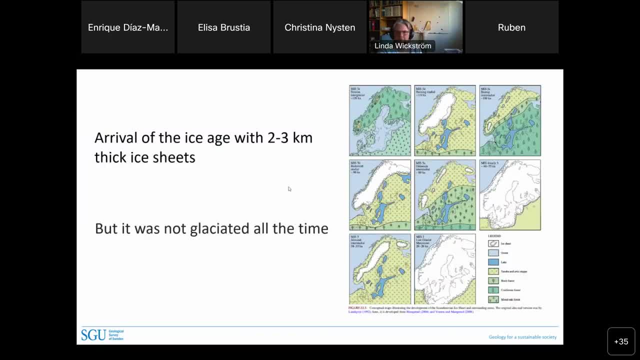 changes in climate. So you have arrival of the ice age and you have two to three kilometers thick ice sheets in this area. But most people think that the ice were there all the time. but it wasn't, as most geologists know. So there were time. 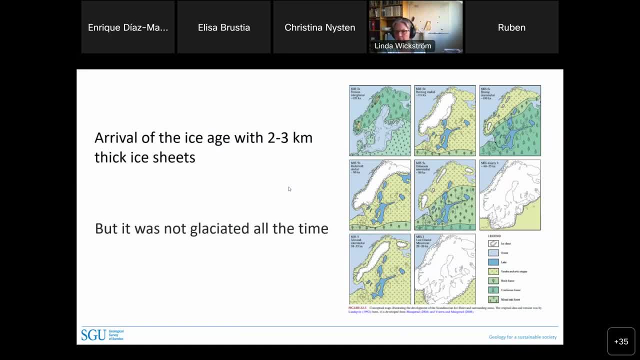 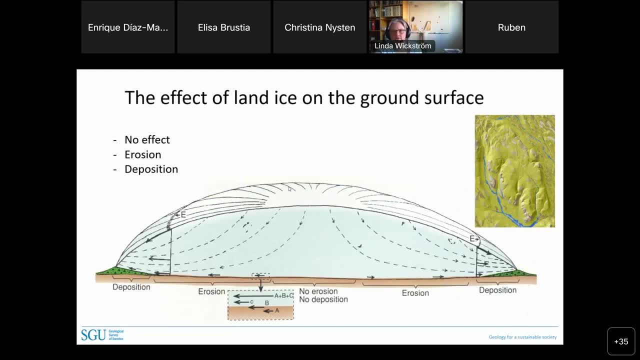 periods with no ice And the ice a big land. ice affects the ground surface in different ways. You have areas with no effect at all. you have erosion and you have deposition, And we can see all this on Furufjället and that's why. 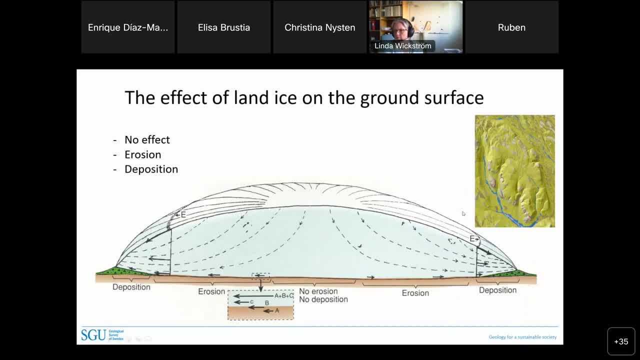 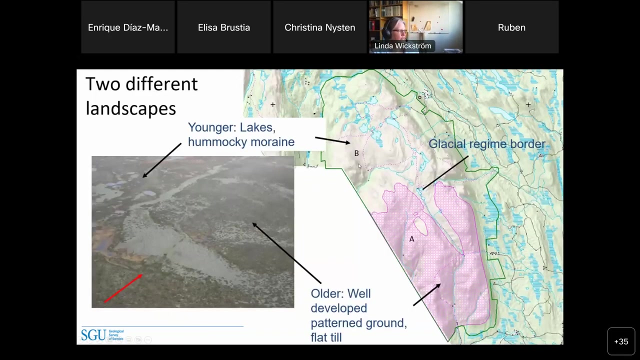 it is so rocky. And this soil map to the left here, which is where you can see the blue, which is that deposited material, and the much in in the some of the yellowish, a lot is erosion On Furufjället. you have two different landscapes and as a geologist I think this is very fascinating. 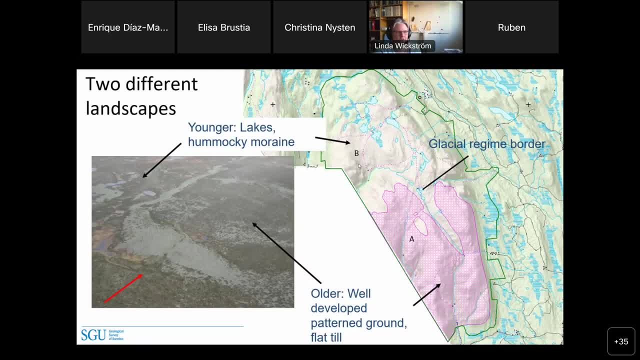 As an A normal person, you just don't see it. You just see the tumble of rocks and you just wonder why, why So? so on the, On the northern parts of the mountain, you have a younger landscape with lakes, lakes and murrain. 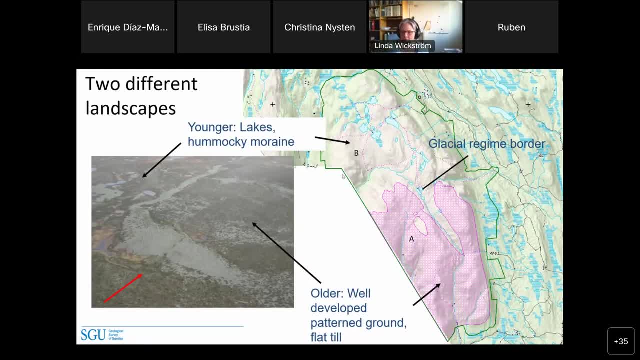 And in the south you have a well developed, patterned ground and flat till On. in the photograph you can see the red arrow- That's the direction of the eyes, So you can see how the ice has actually moved the rocks forward. 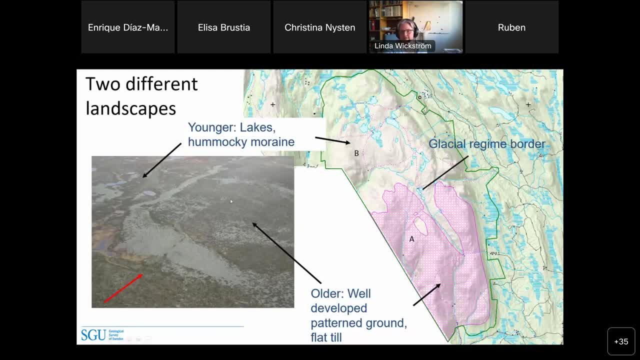 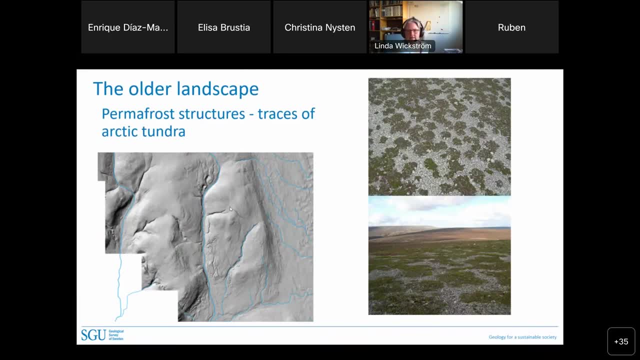 And after that left, uh, left this lake Landscape and the all the landscape you can in in in lighter. you can see that it's a very flat surface And if you go closer and take Photograph, you can see, uh, perma, perma, frost structures and traces of Arctic tundra. Uh, and that's a lens, That's. 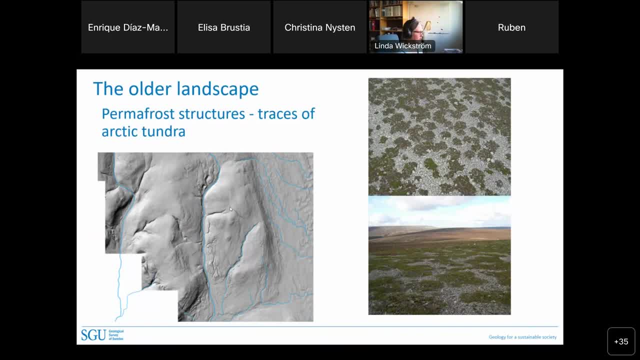 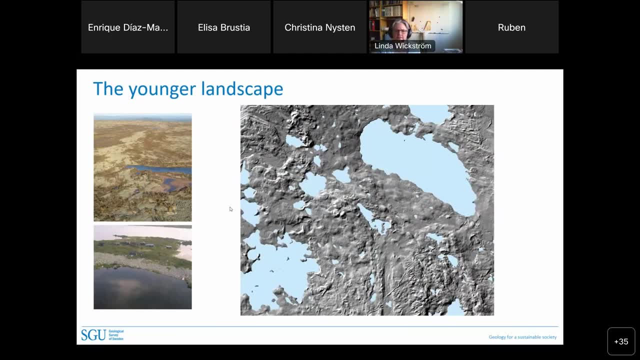 Climate conditions that aren't uh developing Today. uh, and these are very old. And then the younger landscape. you have a lot of lakes and uh and it's more uh boulders Everywhere. so you can also see a difference in in. 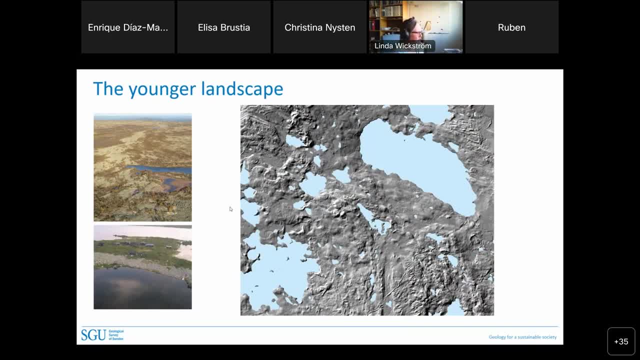 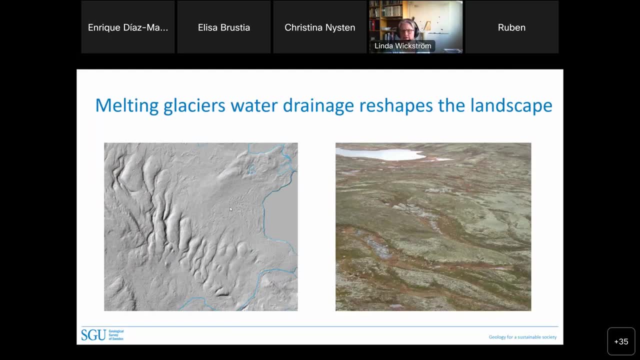 Uh, when you look at LIDAR, for instance, And then also the melting water, uh has reshaped the landscape and and uh transported the, the uh, The blocks and gravels uh to other places, which is also very clearly seen, and that's also when you walk up and down. 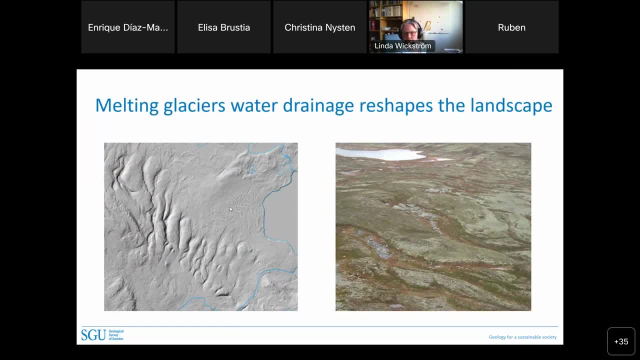 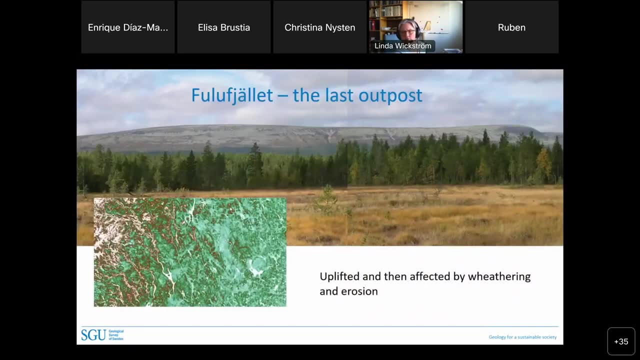 That's very often drainage, uh channels of different kinds. So that's the uh and, But the rocks in itself. um, what are they? That's also, But people ask: and how did get its uh shape? Uh, I used to call it the last outpost because it's on the border to Norway and it's like from the Swedish point of view it's. it's a very solitude sort of kind of mountain. 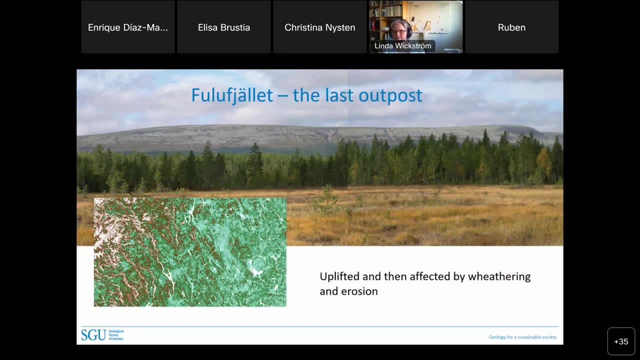 Whereas in Norway you have a more hilly landscape. Um, so If you go for Norway, it's the end, if you go from Sweden, it's the beginning. So this part of of uh the world has been uplifted and then affected by weathering. 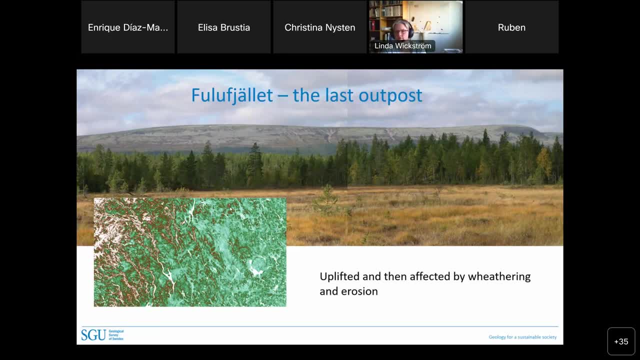 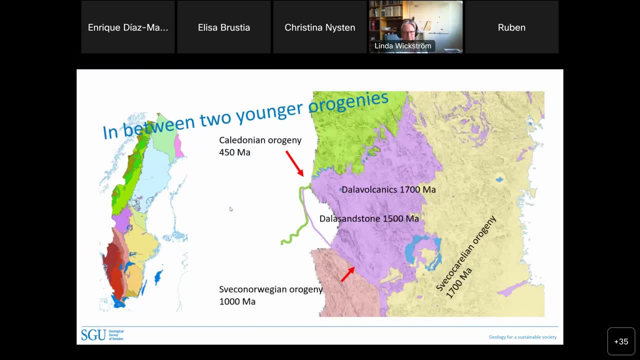 And erosion, and it's the weathering and erosion that has actually uh shaped uh the mountain, because Um area it's, It is um uh in the middle of this uh of the. I don't know if you can see my point. uh, you probably can't. 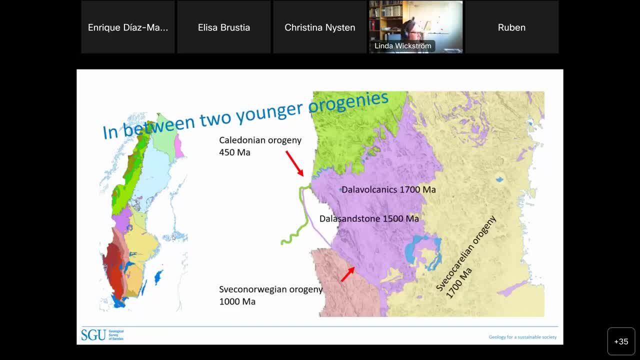 It's actually where the you see the name dollar Sunstone, It's just uh. above Above that, uh, it's, it's uh, squeezed between 2 younger. So this part of the world has um a Sunstone, that's uh. 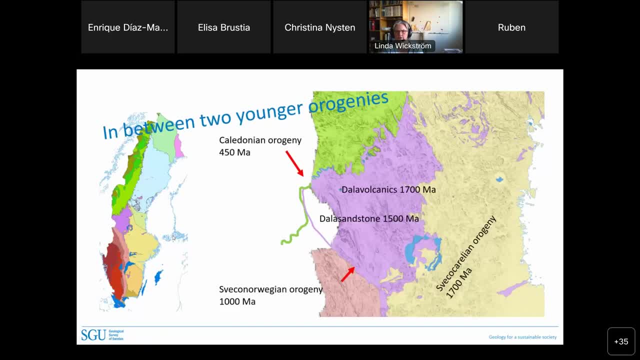 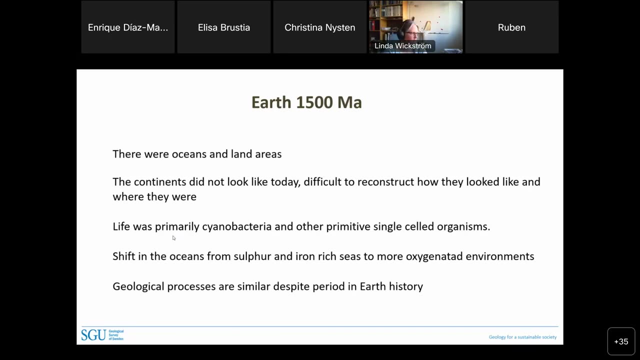 1500Million years old, and it's been squeezed between the Caledonian, So it's also 1 of those places that has actually managed to survive. And what is difficult to explain to people, I think anyway, is that so how? how did? how did earth look like? 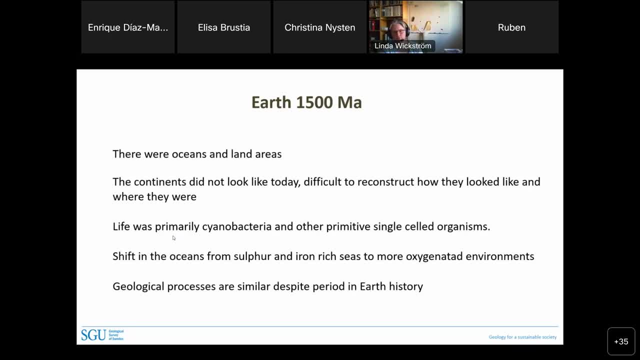 1500Million years ago, then you have to, You have to talk about that. there were lands and there were continents and there were oceans. Um, the continents Didn't look like today. It's difficult to reconstruct how they looked and where they were on it. Um. 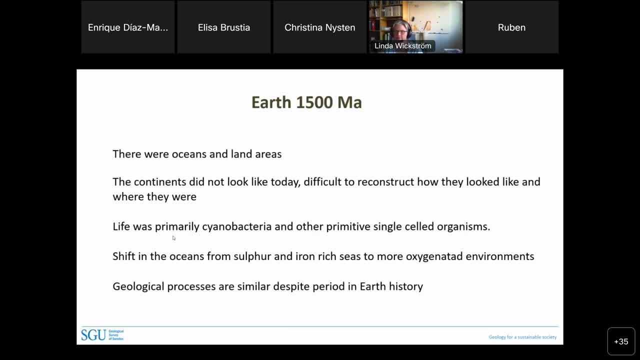 And, uh, yes, there were. there was life on it, um, at this time, but it was primarily science: bacteria and other single celled organisms. Uh, so no bugs, no insects or no dinosaurs anything like, or fish or anything like that. 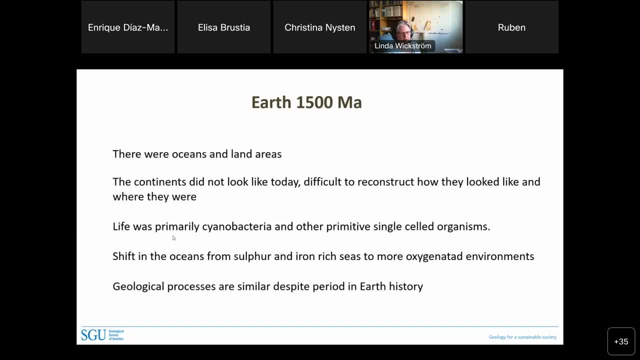 And the oceans, uh, Were also different. there were oceans, but they were sulfur and iron rich, um, and during this period of time, you had to change to more oxygenated environment, environments which favored, uh, of course, then, uh, the evolution of life. 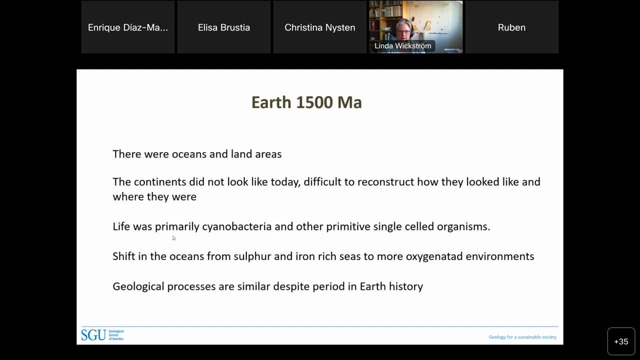 And to, when you talk to to these uh, non geologist, it's always good to to remind them that the geological processes are similar, despite During and when in and in um Uh history, um, they were formed. because that makes it easy to to do modern analogs, which they often can can relate to. 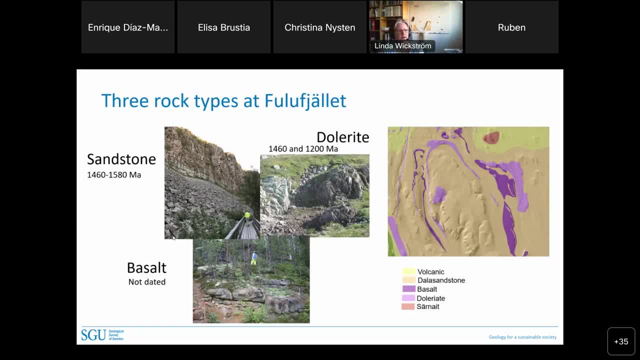 Actually, if you let, the better. geology is quite simple. you have 3 kinds of rocks, you have a sunstone that's very old and you have a dollar right That's slightly younger, and you have a basalt that's surrounding the mountain. That's um. 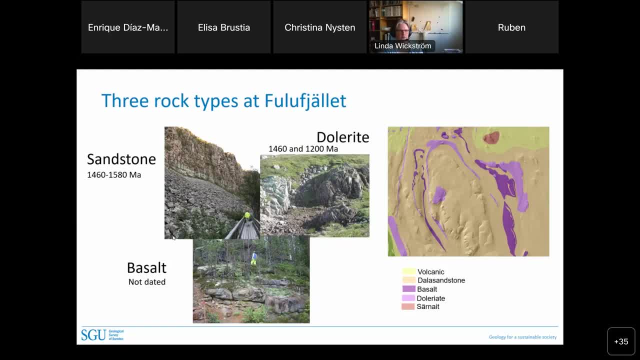 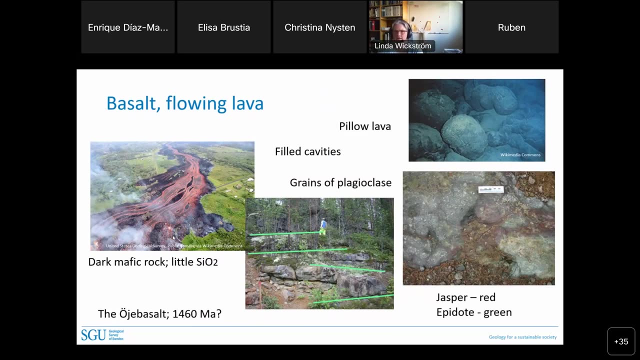 Sorry. so what they see Is actually the sunstone. that's what people see, and they can see the dollar right at some places. So then you, you talk, uh, and try to explain what a basalt is, and when you say that it's a flowing lava and show them pictures from Hawaii or something like that, then it's all very, um, very fascinating. 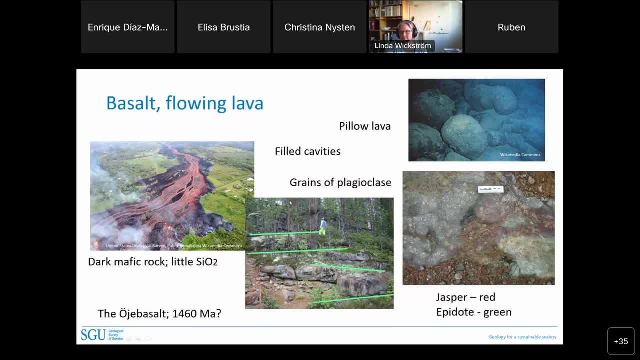 And then they can go to to this place, For instance. This is actually below the mountain, but here you can actually see individual, uh, lava flows that are about 1500Million years of years old, Uh, and that's quite impressive, I think, and you can see a pillow of us and 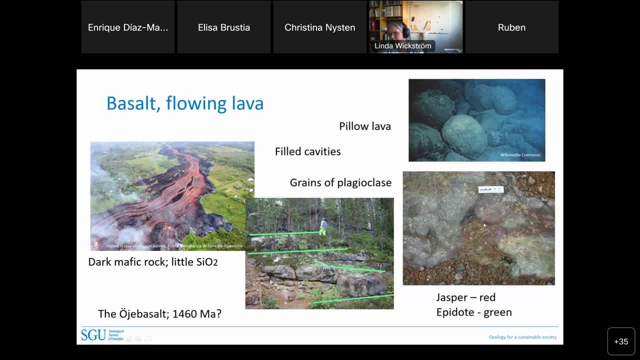 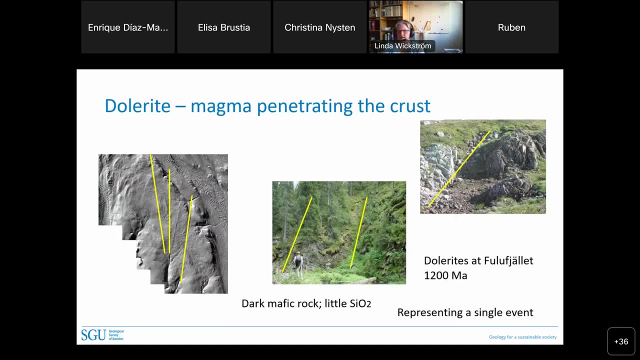 Uh, you have just an epitaph. uh, that's been formed around them, surrounding them. So that's One fascinating thing about this place. When you talk about the dollars, right, I You tell them: that did you have. 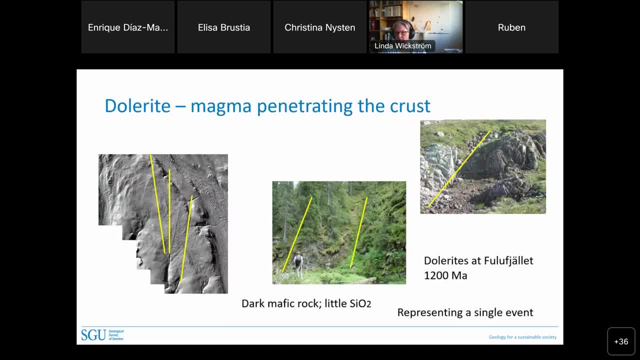 Uh, that's been penetrating the crust instead of instead of sort of flowing out on. On the sunstone You had émie Forming dykes, um, And you can see them later, which is very. I've drawn a yellow line here so you can actually see them better. and you can see them in the field either. 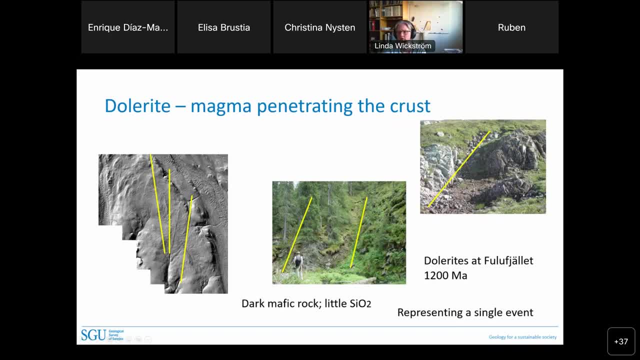 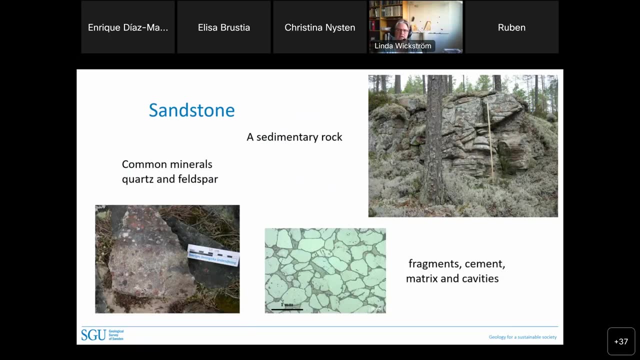 Like to the right, where you have the dollar right in the dark and the Uh Sunstone court site is actually weathering quite bright in some places. And then you talk about the Samsung, which is what they see, more or less That it's a sedimentary rocks and the common minerals, of course, and 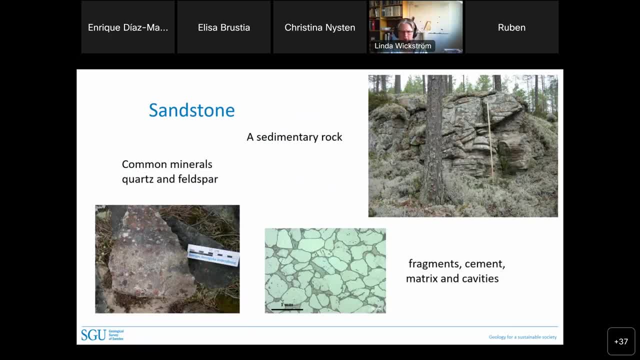 And you can also see a very nice conglomerate in this Sunstone, Um In some places. and then also that the Sunstone Is composed of fragments, seven matrix and cavities, and then you can talk about what these cavities are filled of, for instance, or what they can be filled up. 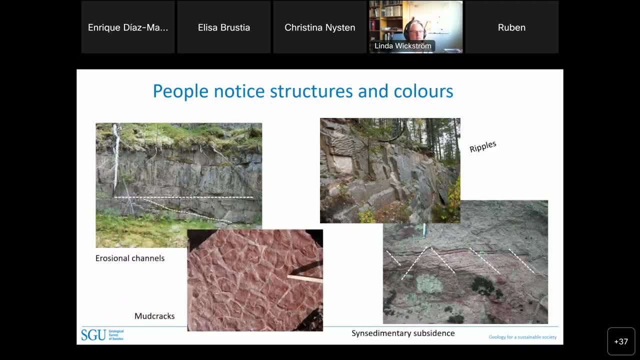 And when people look at these rocks, what do they notice? Well, yes, they, they. they notice structures and colors and they want to know why is the Sunstone red And why is it yellow at some places And why does it look funny, Um, and things like that, Um, 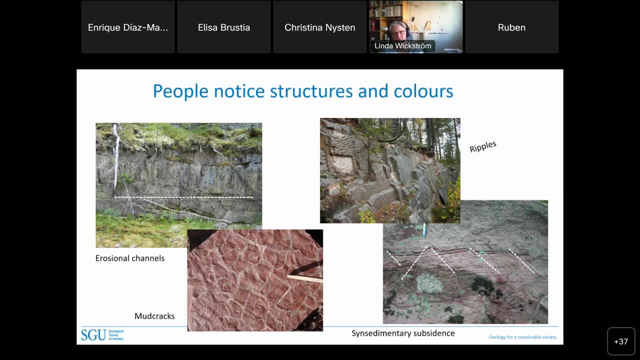 So that's very for it. as a geologist, It's not very Difficult to talk about. you just have to Think that They they don't want the deep story, They just want to know why. Why does it look like? why does the Ripple looks? looks like. 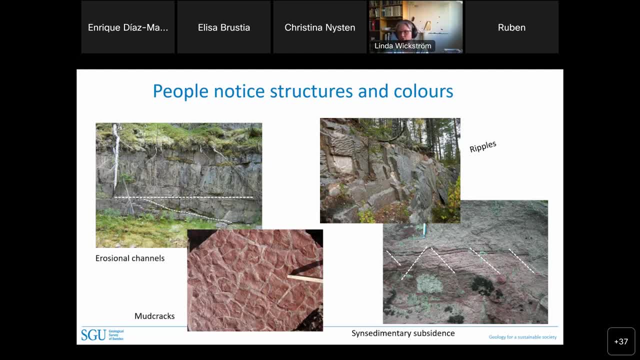 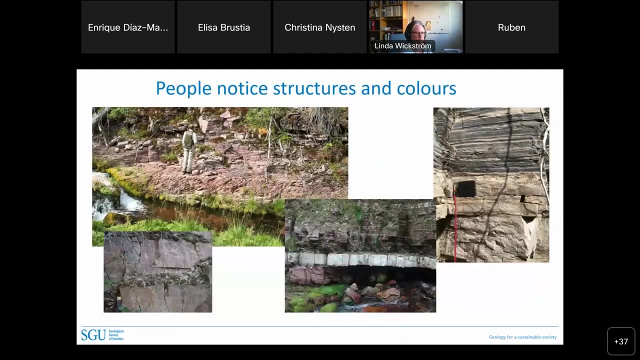 Look like the do, and where can they have been formed? What is more difficult to actually Explain sometimes it's actually the changes in in colors, Where you have the very fine grain, uh, Mud, um, Parts of the sections which are very, quite purple. 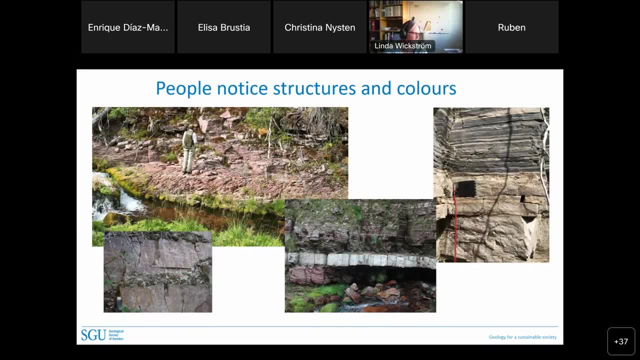 Purple is red, uh where, the more course, uh course, grain layers are quite bright, Actually, white white dish. And then you have other, uh, other processes that can change the color of the rock. You can have weathering, uh which. 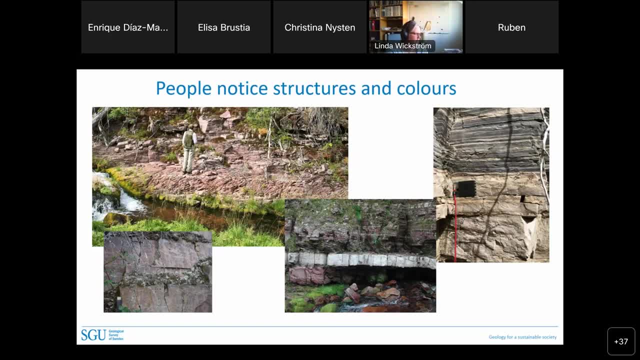 Which is what you have to the, to the uh on the picture, to the, to the right, where it, where the Back, and you can also have a hydrothermal solutions, um, bleaching the, the rock, creating uh Patterns, like, like the patterns to to to the uh. to the left. 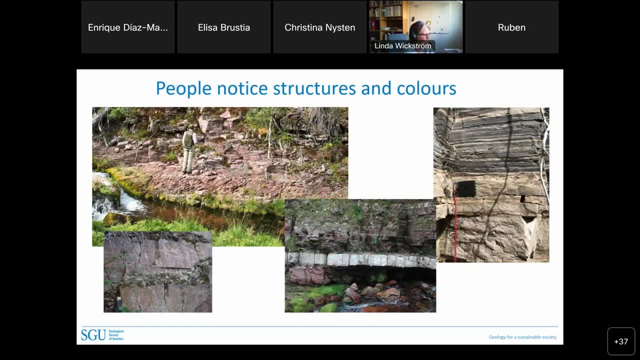 So that is mostly what People in the end wants to to to know. it's the structures and the colors. And then also, if you can tell a fancy story About why, why, why the structures look like they do and why the colors are like they are, then it's: uh, they like it. 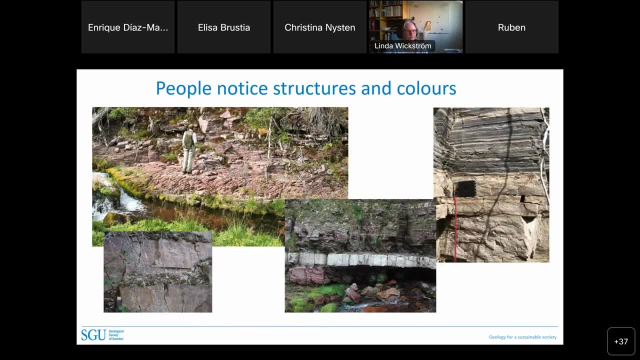 Thank you, that's it Okay. thank you very much. Uh, Linda I I thought you were going to finish with some more conclusions. Oh, that's okay. That's okay, I mean. it's no, no problem. It's a good example to all the things that you have been doing at this national park for for the tourists. 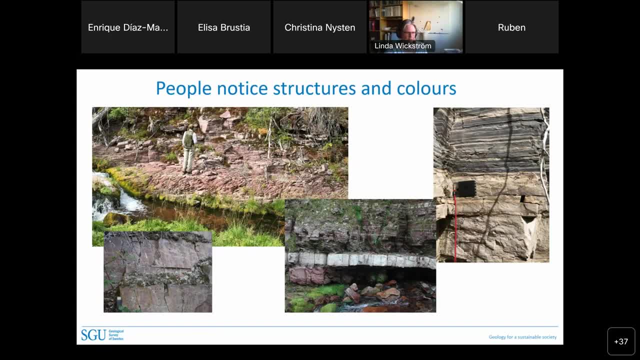 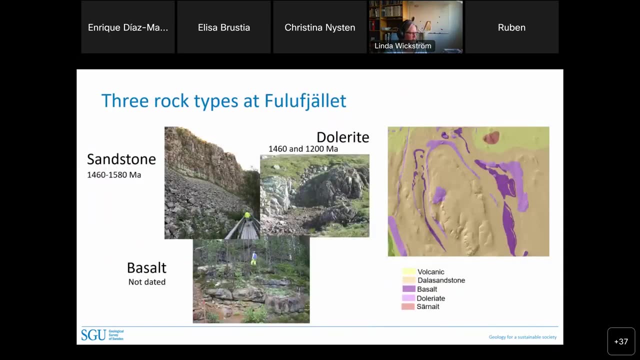 Okay, uh, so we will talk uh. I mean, I'll have some questions later, and now the 3rd and last 1.. That we'll be talking uh will be Kirsten lemon, from the Geological survey of Northern Ireland, of the British geological survey, and she will be talking about the threats and opportunities for geological heritage. 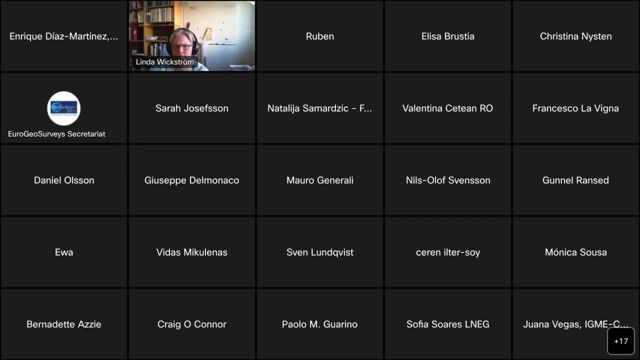 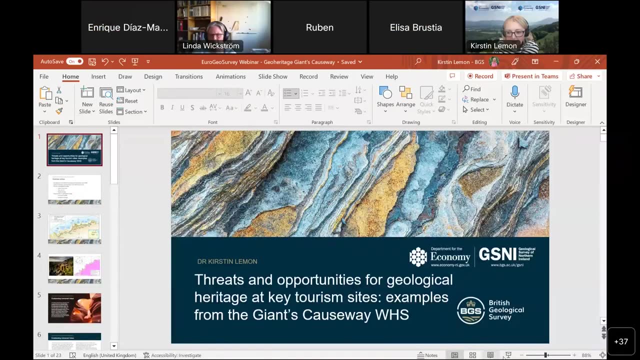 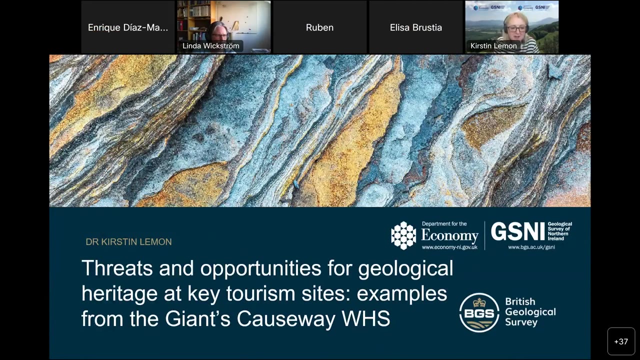 At key tourism sites. examples from the giant cause way world heritage site. Thank you, I'll just share my screen. Hopefully is that working Okay. Yes, we can see it Okay. Go ahead. Thank you very much. So good afternoon Everybody. 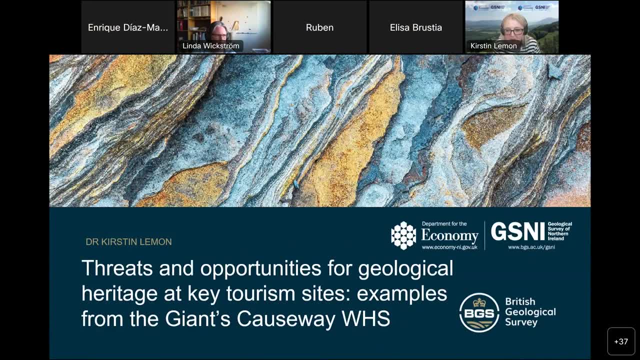 As Enrique says, my name is Kirsten lemon. I'm a senior geologist at the geological survey of Northern Ireland. Just to explain a little bit about what the geological survey of Northern Ireland is- and we are an office of the Northern Ireland government department for the economy. 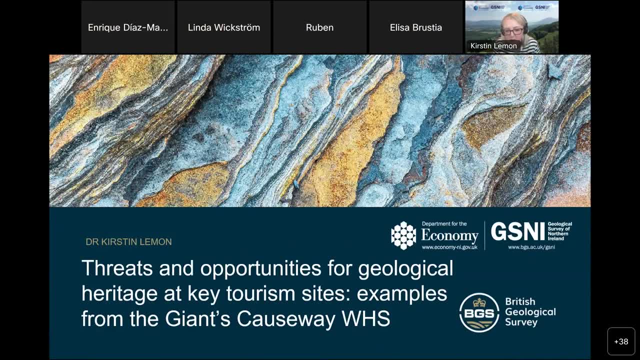 But we are staffed by scientists from the British geological survey, So that's why I've got the 2 logos up there. My role is to look after a number of work programs, and 1 of those is environmental change and geological hazards, But the other 1 is called science. 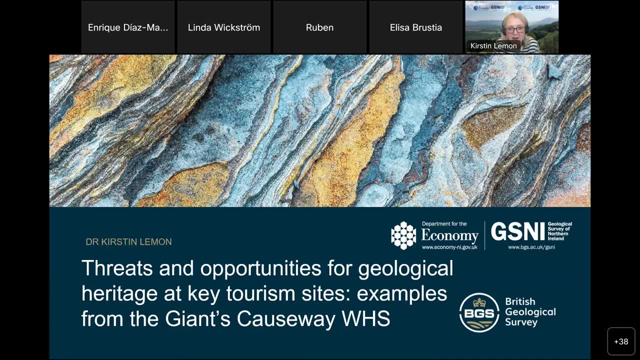 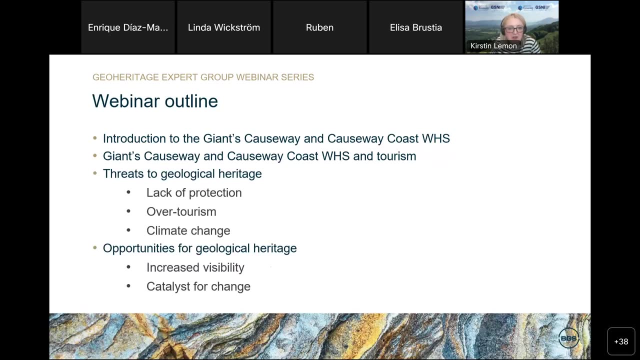 Science for society, where part of my role is to develop geological tourism in Northern Ireland and also to work with those places to understand geological heritage. So it's in that vein that I'm talking this afternoon. So what I would like to do, 1st of all, is to introduce you to the giants causeway and causeway coast world heritage site, to give it its full name. 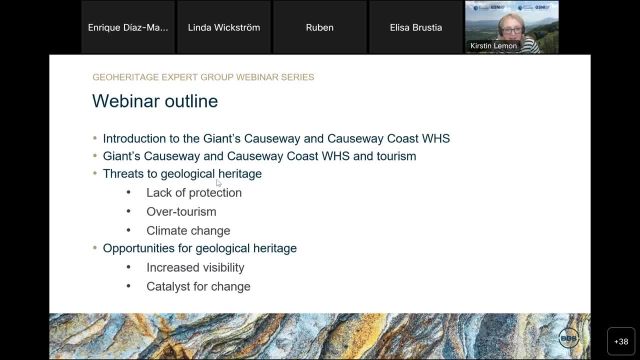 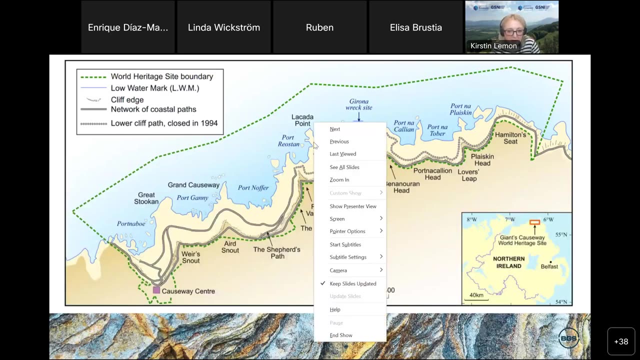 And then explain how tourism works at the world heritage site, And then I want to explain some of the threats To the geological heritage there and also look at some of the opportunities for geological heritage, just to finish up. So, 1st of all, the giants causeway. where exactly is it? 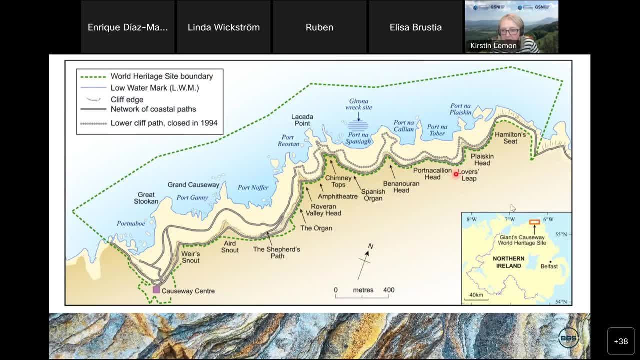 I'm going to try and see if I can find a pointer so I can just give you a little bit of an idea. So in the little map in the corner we've got a map of Northern Ireland. Here is Belfast and the giants causeway is approximately 100 kilometers away from Belfast. 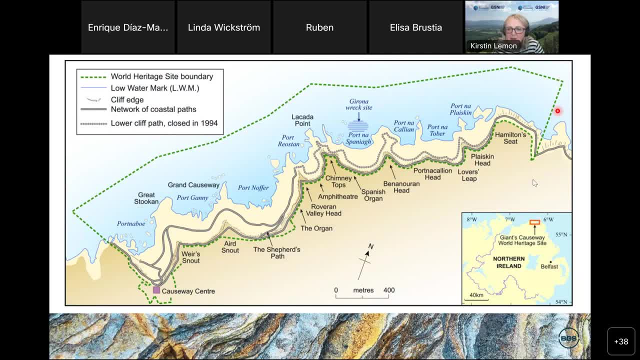 You can see the site is marked with the green dash line. It's around about 5 kilometers in total across and only about half a kilometer wide, So it's not a very big site. It's really served very well. but the giant causeway visitor center that opened up in 2012,. but the majority of the site is made up by paths. They go along the top of the cliff, but they also go along down past the causeway and all the other main sites as well. 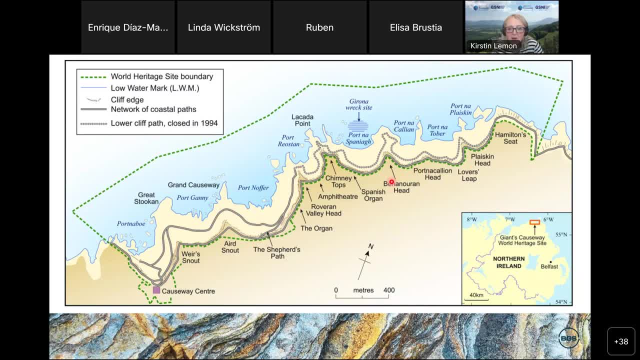 You'll notice that the cliff top, The path extends all the way across the World Heritage site, but the path down here, the dashed one, has been closed since 1994, and I'll talk a little bit about that later on. So it's made up of a predominantly marine environment, but it's also got a terrestrial component too, as you would expect. 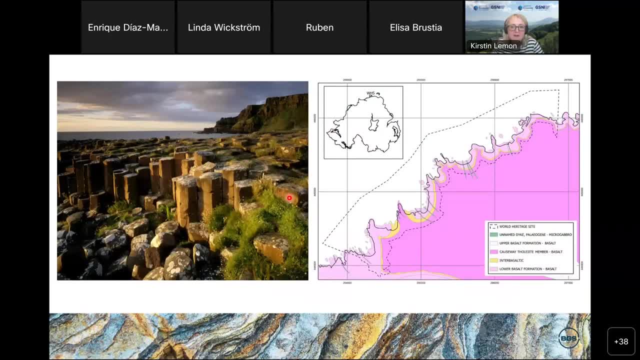 So this is the iconic image of the Giant's Causeway. This is what everybody knows. It's made up of approximately 40,000 basalt columns and that's the image that people associate with the Giant's Causeway. But it's about a whole lot more than that, and I'll go into a little bit more detail in a moment. 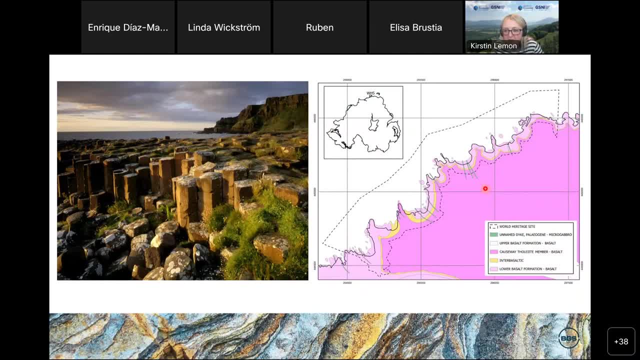 Just to talk a little bit about the geology I've put in a geology map here, And to a geologist this geological map actually does not look very exciting at all, Because the Giant's Causeway is made up really of one main rock type and that's basalt. 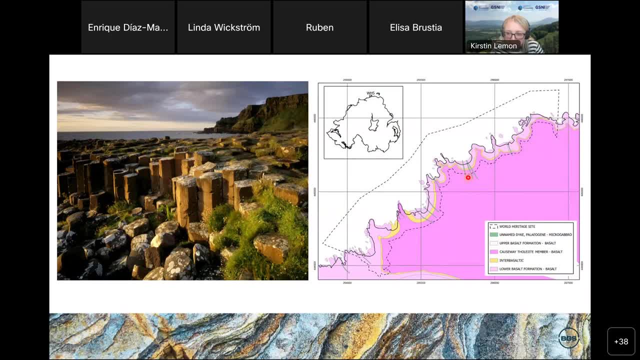 So the basalt formed during the Paleogene period, or the Paleocene to be precise, around about 60 million years ago, And was formed as a result of volcanic activity associated with the opening of the Atlantic Ocean. There are three main layers of basalt. We've got the pale pink, which is what we call the lower basalt formation. 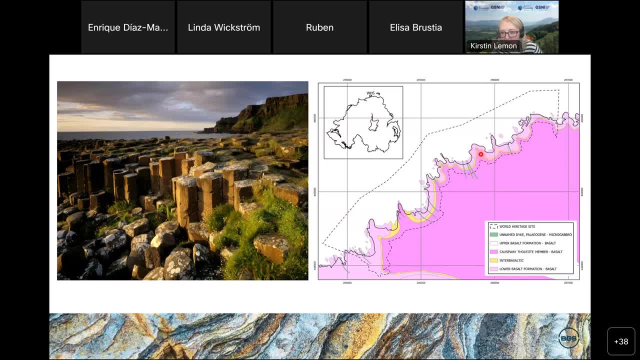 And then, on top of that, we've got this orangey layer. This orangey layer represents the lower basalt formation. and then, on top of that, we've got this orangey layer. This orangey layer represents the lower basalt formation. and then, on top of that, we've got this orangey layer. 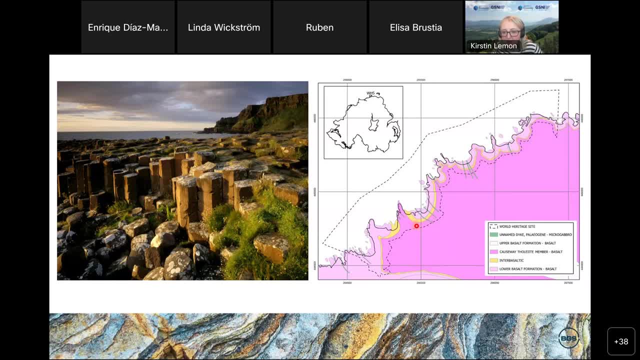 This orangey layer represents the upper weathered surface of the lower basalt formation, and that's what we call the interbasaltic formation. And then the darker pink. this bit here is called the Causeway Thuleite member, And again it's basalt as well. 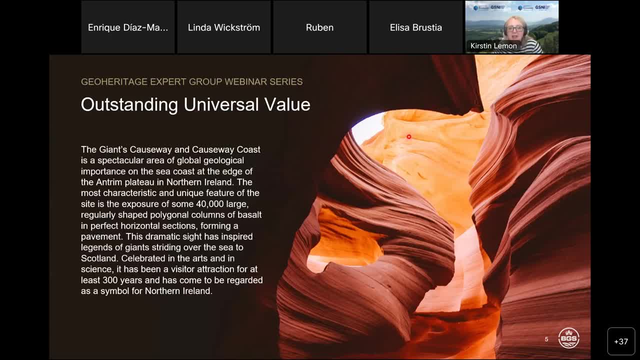 So, being a World Heritage Site, it has to have outstanding universal value. And I'll apologize for this image because it has nothing to do with the Giant's Causeway, It's just the BGS house style. So I've lifted out this section of a description from the ONESCO website and I'm not going to read it out, but I just want to put pick out a few comments. First of all, the outstanding universal value of the Causeway is because of its unique exposure of 40,000ario世 온. 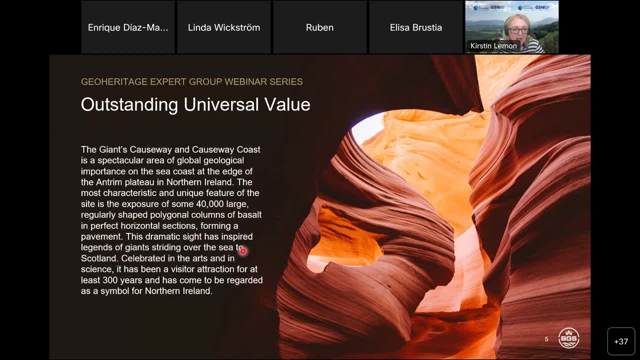 causeway for a reason: because it's associated with an Irish giant who had a fight with a Scottish giant, and it really is celebrated in the arts and in science all the way across the world. It's been a visitor attraction for at least 300 years and this bit at the 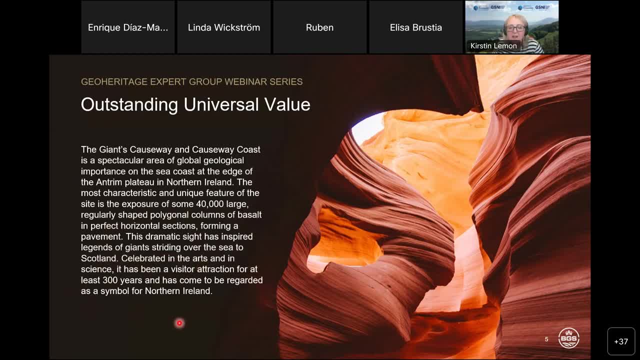 end it's become regarded as a symbol for Northern Ireland. So our geological heritage is very much ingrained in Northern Ireland society as a whole, looking like it's part of Northern Ireland's soul. So just to explore the outstanding universal value a bit more, each World Heritage Site: 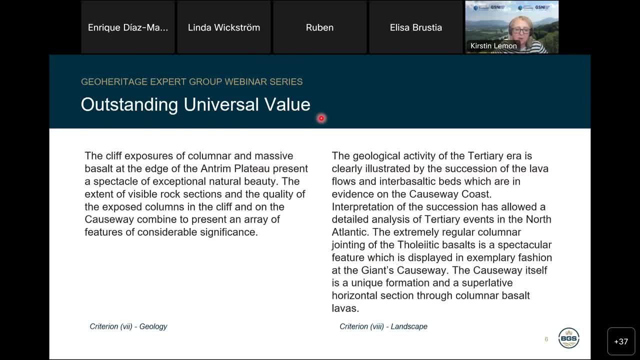 gets inscribed on the World Heritage List depending on what criterion it fulfils. The Giant's Causeway is one of only two percent of World Heritage Sites around the world that have been inscribed because of their geological heritage. It's been inscribed under criterion: 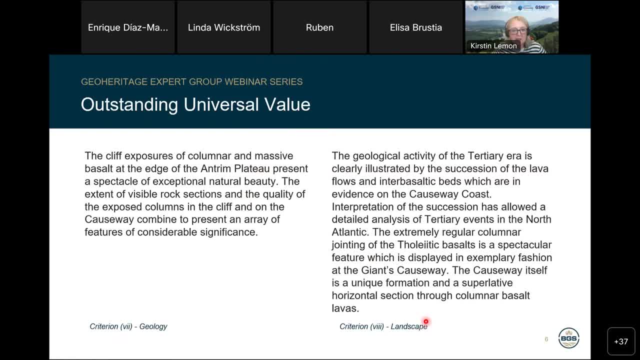 seven, which is geology, and criterion eight, which is landscape Criterion. seven is really talking about the columnar mass of basalts at the cliff edge, so it's talking about the cliff exposures, and then the landscape setting is really to do with the fact that it shows you the sequence of events during the Pelagian period. that 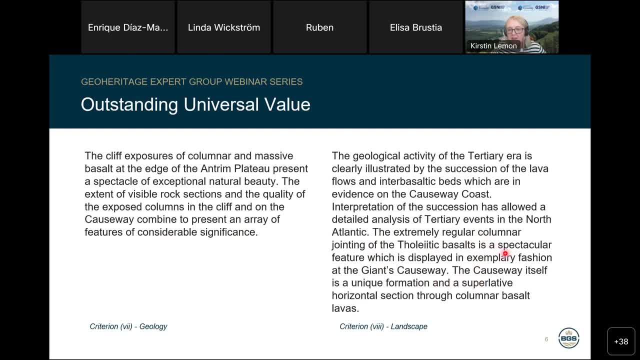 really let us understand better the events in the North Atlantic. Just to explain, I've used the word tertiary here because that's how it's written on the UNESCO website, So it'll give you an idea about why the Giant's Causeway World Heritage Site is so important. So I'm going to show you a little bit more about the Giant's Causeway World Heritage Site. I'm going to show you a little bit more about the Giant's Causeway World Heritage Site. So I'm going to show you a little bit more about the Giant's Causeway World Heritage Site. 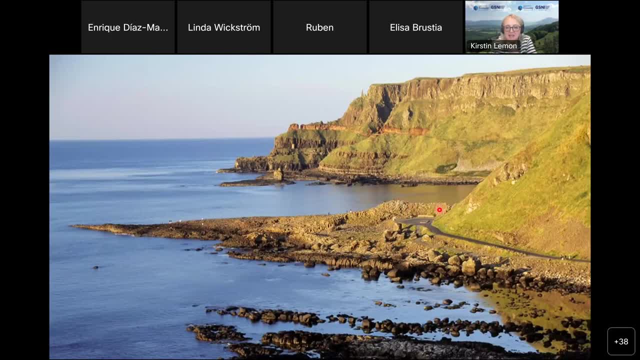 So I'm going to show you a little bit more about the Giant's Causeway World Heritage Site. So this is the characteristic view of the causeway. This is what's called the main causeway or the grand causeway. This is where the predominantly large number of the basalt columns 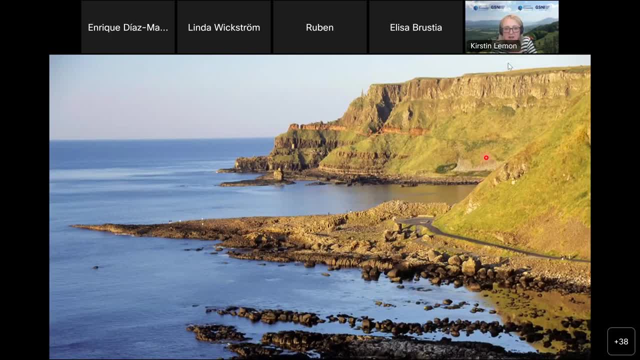 can be found. But, as a description of the geological heritage showed us, it's not just about those columns of basalt, it's also about the cliffs. So we can see some really lovely exposures of the lower basalt formation. We can see the interbasaltic formation, this lovely red layer of laterite. 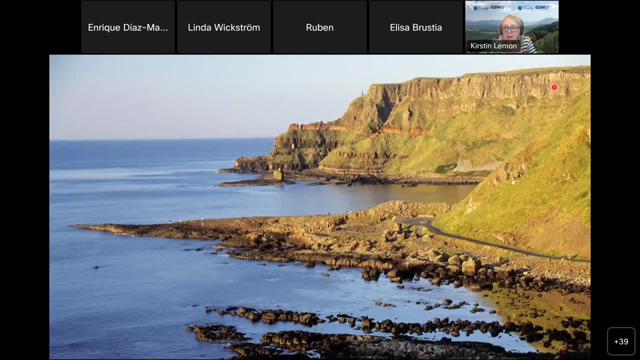 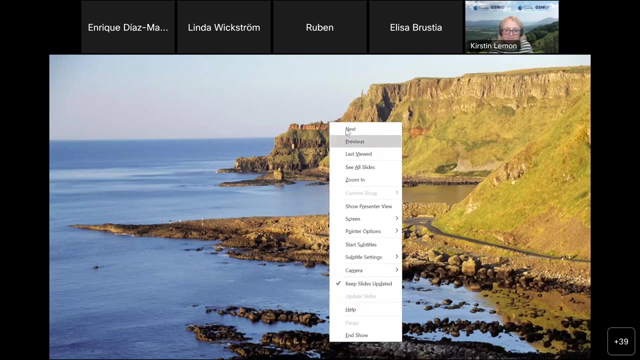 And then you can see the upper causeway tholeite member as well. So the causeway columns are really only a small part of why this place is so special, but it is the reason why most people come to see it. Now I just want to talk a little bit about the site ownership and management, because 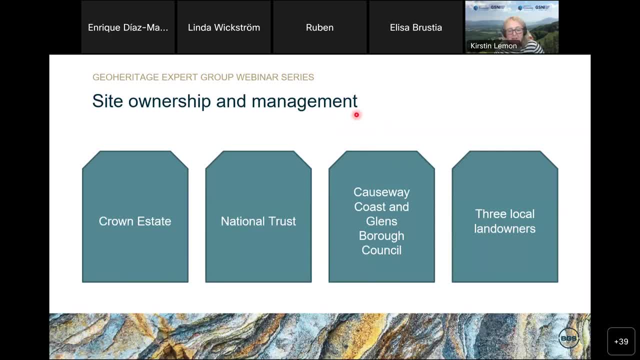 it's really important for how tourism has developed on the site. The Giant's Causeway and the Causeway Coastward Heritage Site are two of the most important sites on the site. The Giant's Causeway and the Causeway Coastward Heritage Site is made up of around about 240 hectares of land. 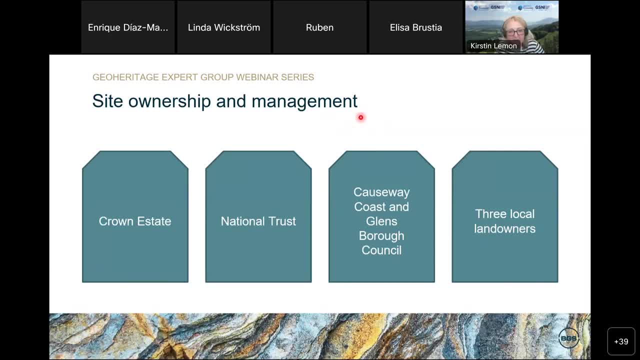 Two-thirds of that is owned by the Crown Estate. So the Crown Estate is essentially sovereign property. It doesn't belong to the monarch, but it does essentially make revenue that they can then use to input into the British government. About a third of it is then owned collectively. 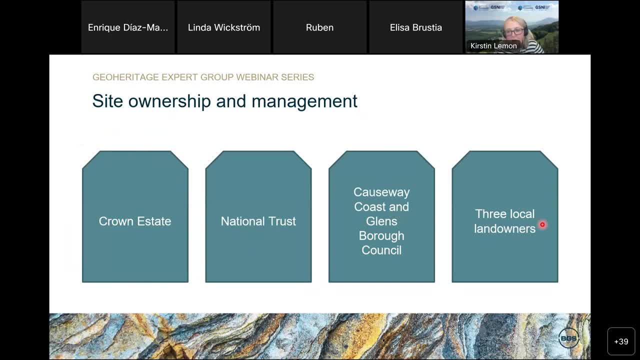 by the National Trust, the local council and three local landowners. However, about 12 of those landowners are owned by the Soil Trust, which are managed by the Soil National Trust. The National Trust is Europe's largest conservation charity. They own huge amounts of coast and 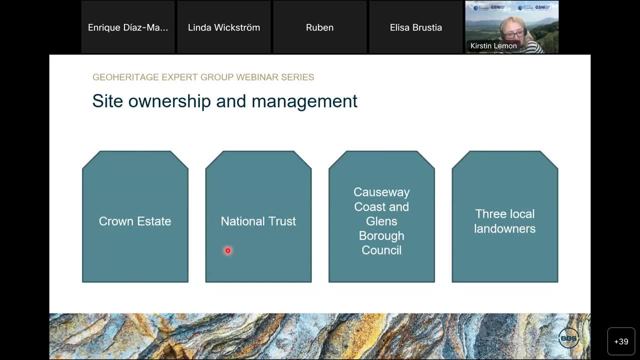 countryside throughout England, Wales and Northern Ireland, and they own a lot of historic properties as well. So they are, if you like, the property managers. They are responsible for the operational management of the site and they also coordinate all activity on a daily basis. 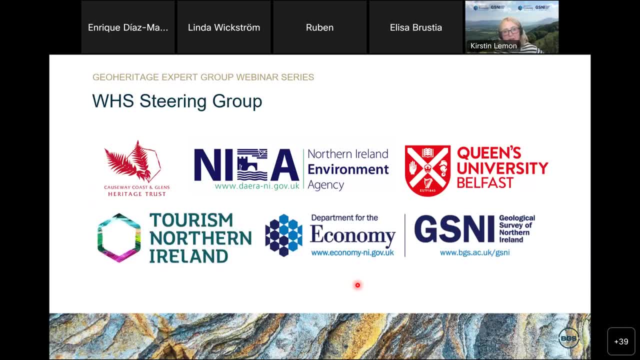 has a steering group. The steering group is there to ensure the implementation of the World Heritage Site Management That takes into consideration conservation, tourism, economic value of the site. It also takes into consideration other aspects, such as community interests. So they are there to ensure that is all implemented. 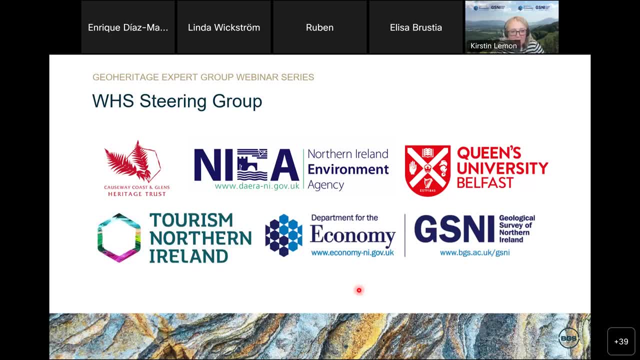 And there's a couple of organizations I want to just highlight here. First of all, the Causeway Coast and Glens Heritage Trust. They are responsible for the secretariat, for the steering group. We've also got the Northern Ireland Environment Agency, who are responsible for geological conservation. 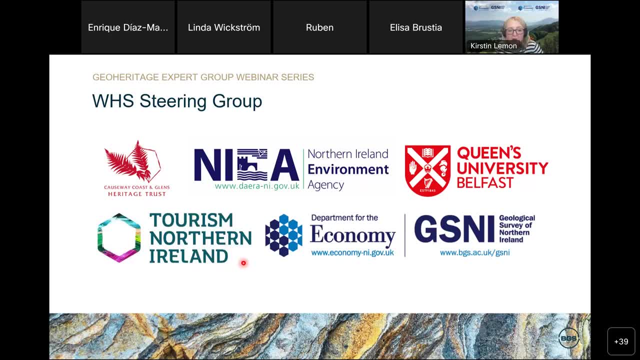 We've also got Tourism Northern Ireland, who are responsible for marketing Northern Ireland, And we've also got my department, the Geological Survey of Northern Ireland, under the auspices of the Department for the Economy. I just want to point out a few things as well here. 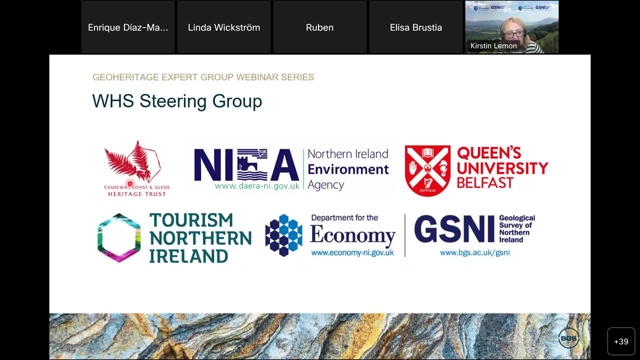 The Causeway Coast and Glens logo, not surprisingly, has got a hexagon representing the Causeway Basalts. But if you'll notice, Tourism Northern Ireland, who are responsible for marketing all of Northern Ireland, use a hexagon as their logo. 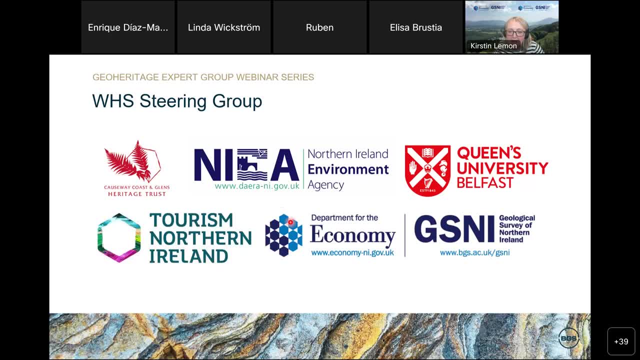 So does my department. This is the same logo used by every government department in Northern Ireland, although each one has got a different color. So to give you an idea of the importance of Northern Ireland's geological heritage and, in particular, importance of the Giant's Causeway. 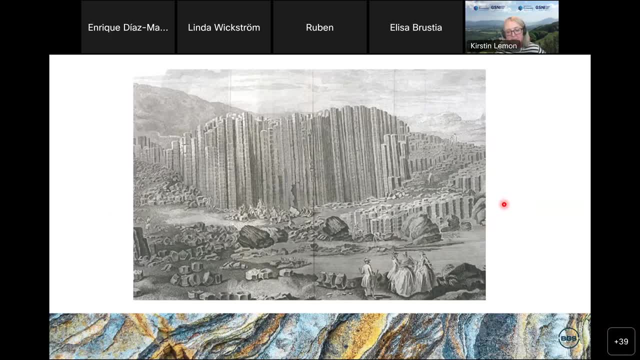 Just a little bit about the history of tourism at the site. The Giant's Causeway first came to the attention of the rest of the world back in the 17th century. It was painted as a watercolor by a Dublin artist named Susanna Drury. 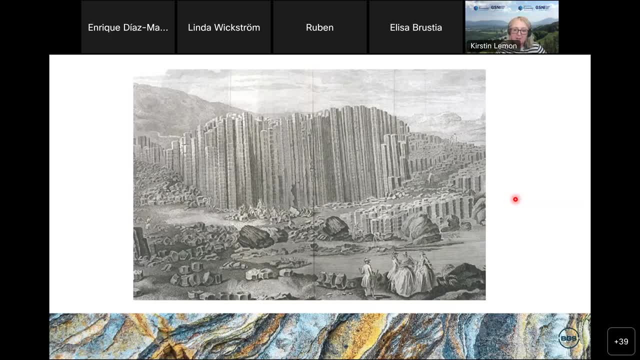 That painting became so popular It was made into. it was an engravement that was then sent all the way around Europe And it then began to attract people to visit. because these rocks were an enigma, Nobody really understood how they formed and their geometric shape. 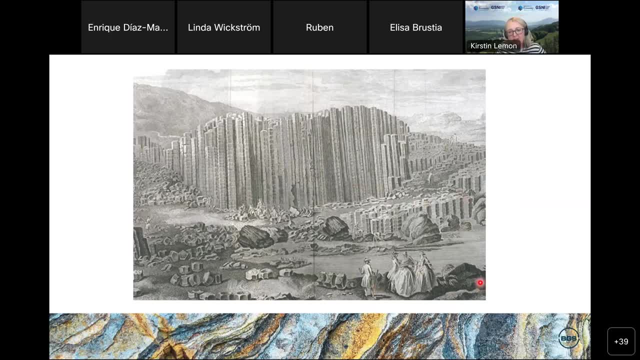 made that they're actually quite unusual. And then tourism to the Giant's Causeway has not stopped. The majority of people that come to Northern Ireland, and indeed the Island of Ireland, want to come and visit the Giant's Causeway. These are just some posters that have been used. 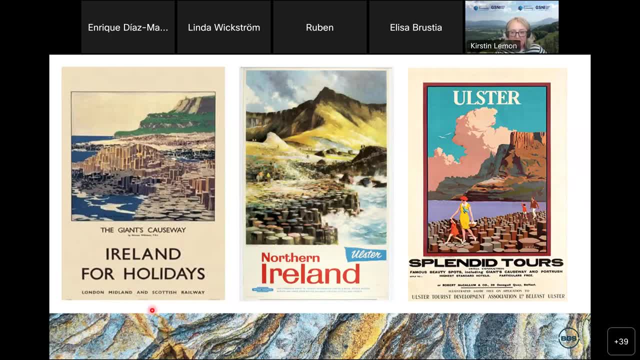 in the early 20th century to promote Northern Ireland and Ireland. each of them has the Giant's Causeway as its iconic image, So you'll see that there's ones that have been advertised to the London, Midland and Scottish Railway. We've also also wanted to be promoted. 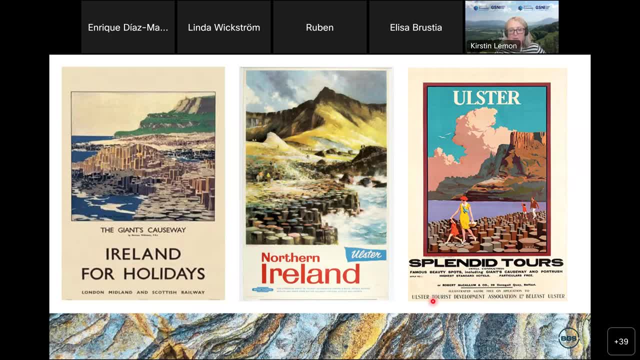 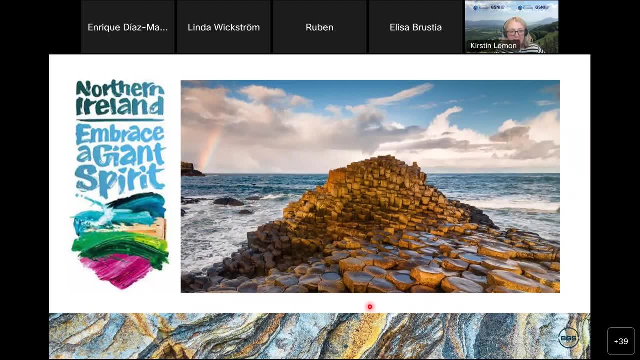 by the Ulster Tourist Development Association, all being used to promote Northern Ireland, with the Giant's Causeway as the key iconic site That continues to this day, because this is actually the slogan that is used by Northern Ireland Tourism: embrace a giant spirit. 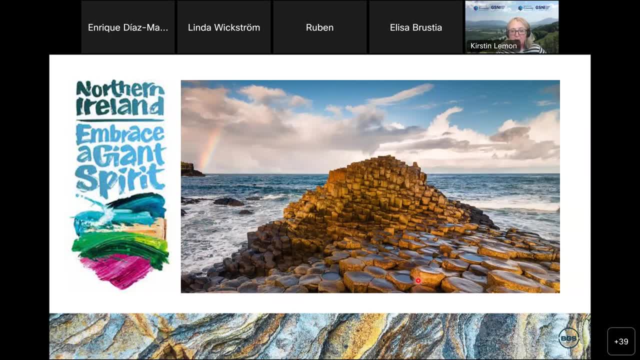 The word giant obviously comes from the Giant's Causeway, and this is one of the iconic images, As I mentioned before. although the geological heritage of the site is about so much more than just the basalt columns, they are what people come to see. 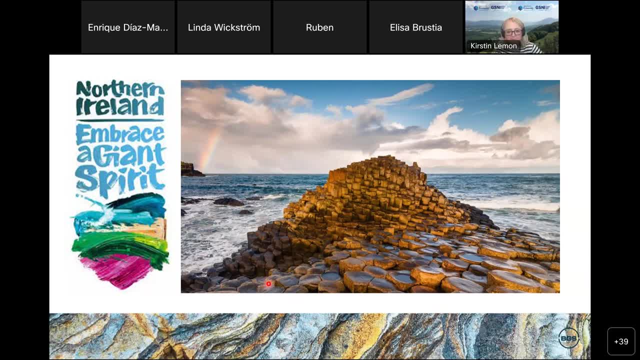 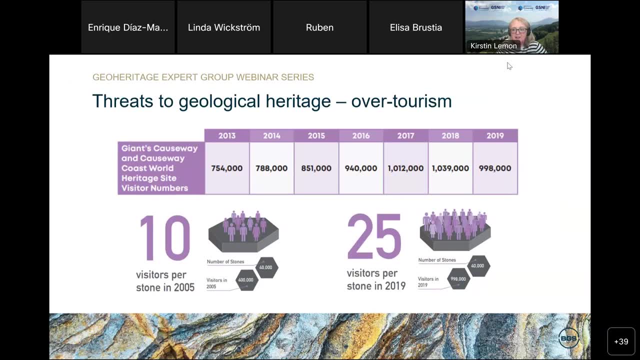 Although whenever they do come, we tell them about the full story. So I'm now gonna move on and talk a little bit about some of the threats to the geological heritage. The Giant's Causeway is undoubtedly Northern Ireland's most popular. I've already mentioned that people come to Northern Ireland. 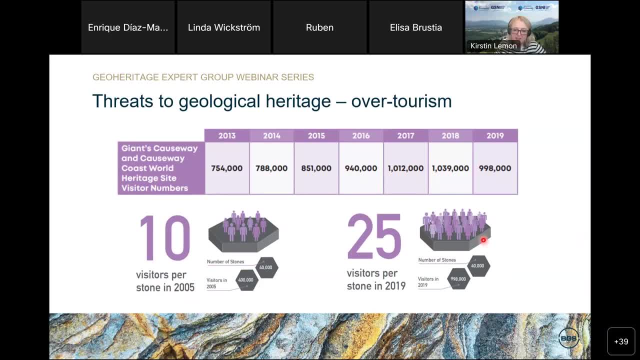 to visit the Giant's Causeway. If they go somewhere else, that's fantastic, but they'll come to the Giant's Causeway first. We've seen a real dramatic increase in the amount of people that come to the site. The new visitor centre opened in 2012,. 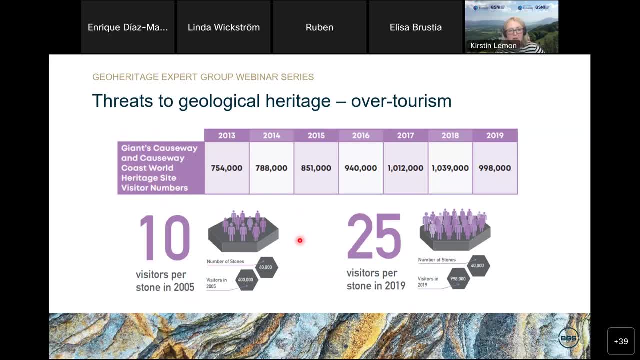 which is obviously somewhere around here, And back then visitor numbers were around about 600,000.. They're now sitting at around 1 million visitors every year. Now for some tourist attractions you might not think that's very much, but if you think about the entire population, 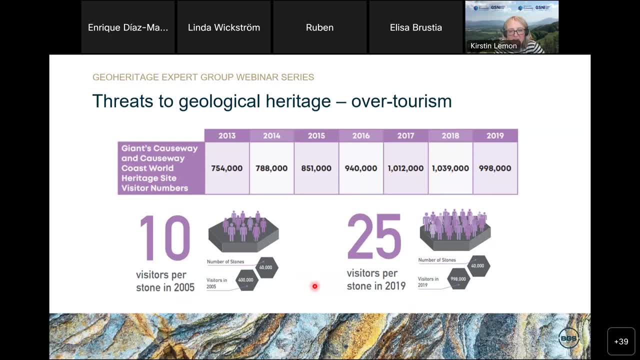 of Northern Ireland, which is only 1.8 million people. that's actually quite a lot, And I've already showed you how small that site is. So again, that will give you an idea of how much of an impact those visitors might have. 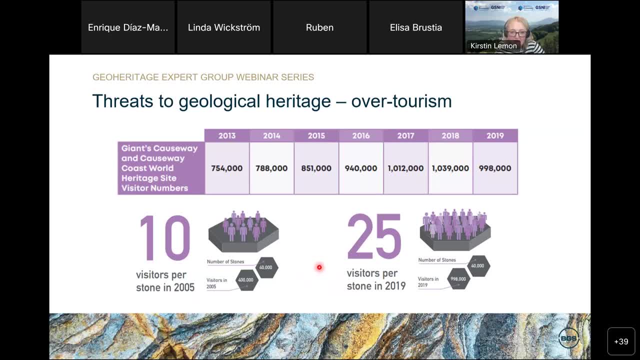 on the site. We've put together a little bit of an infographic. This is actually in the most recent management plan for the site, So back in 2005, we used to get 10 visitors for every stone. Remember, there's 40,000 of these columns. 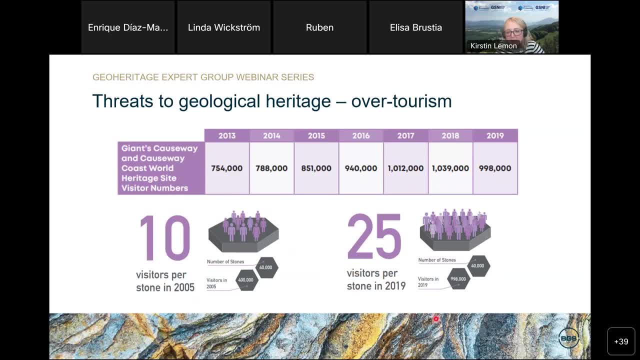 and they call them stones. in the management plan In 2019, there was 25.. So that's a huge increase in the number of people that come to visit the site. By people coming to the site, they put extra pressure on the natural environment. 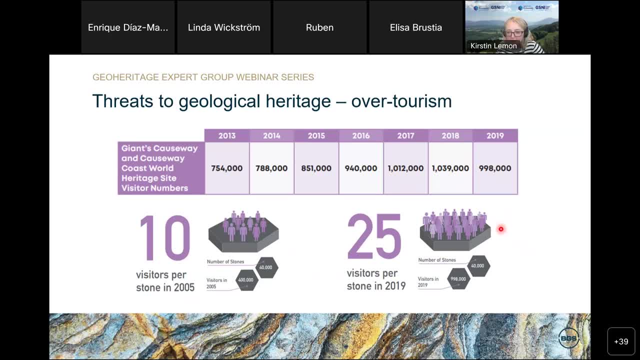 They not only cause weather and then erosion on the columns themselves, but they also bring in bits of pollen, spores and seeds in their shoes, whether they know it or not. So vegetation is also increased on the stones and, more importantly, vegetation that was not normally. 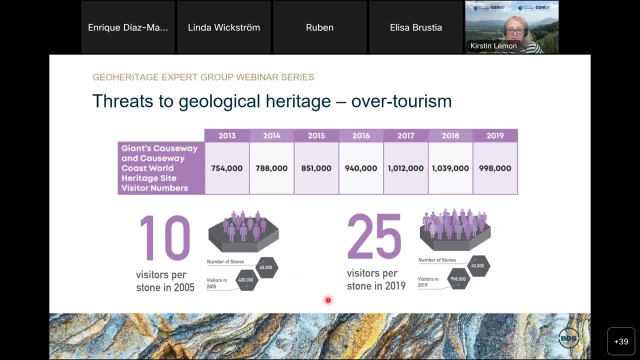 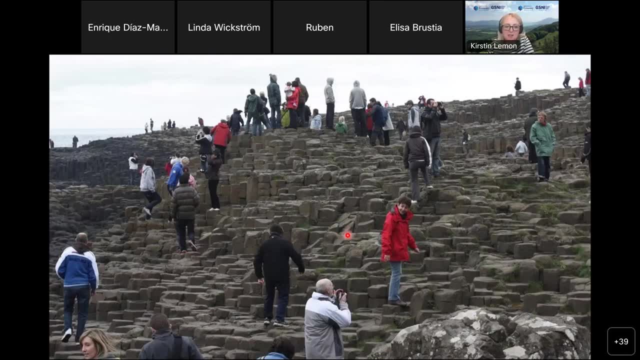 brought into the site. naturally, This is more of a typical image of the Giant's Cause, where the ones I've showed you so far have been the touristic images. They're the photographs that we use to promote the Giant's Causeway, But in actuality, this is what you will see. 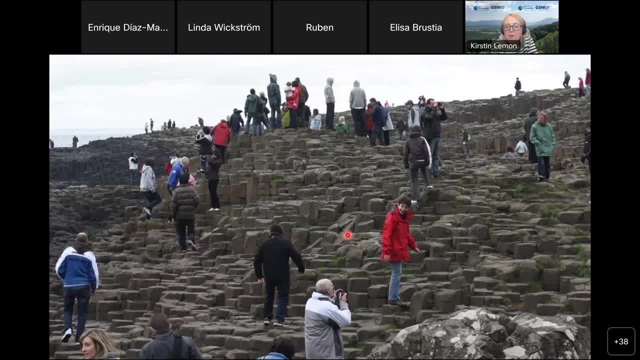 Unless you come to the Giant's Causeway at 6 am in the morning, or if you come late in the evening, you will be joined by lots of other people. So, aside from the fact that there's being damage done to the site, 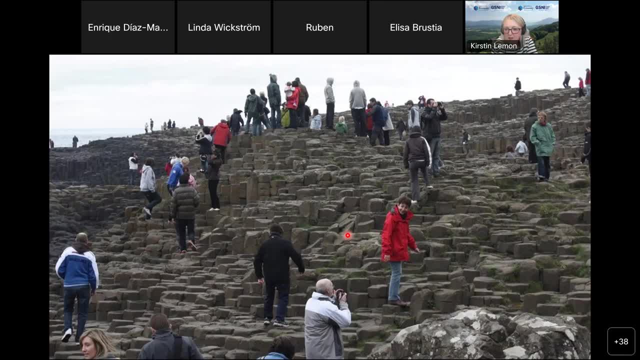 it's also not a particularly enjoyable visitor experience. However, there is a positive to this story. The positive which will come as a surprise, I suppose, to most people is COVID-19.. COVID-19 gave us a chance to you know. 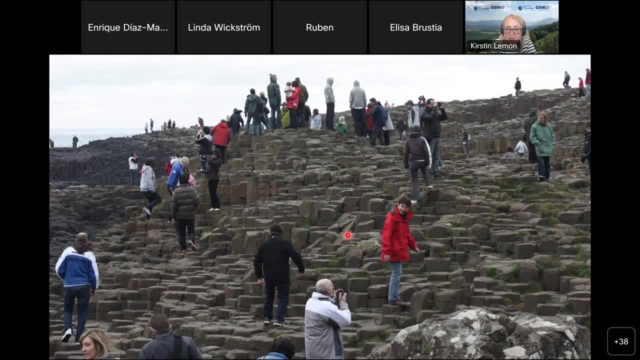 to be able to visit the site. It gave us a chance to really rethink how the Giant's Causeway is looked at when it comes to visitors. I gave you figures there up to 2019, when we were having around about a million visitors. 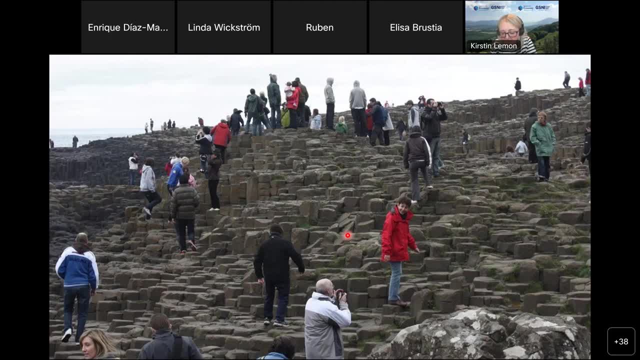 every year That visitor number has obviously plummeted. The one million visitors around. about 60% of them were international visitors, which is quite unique when it comes to Northern Irish tourist attractions. But that number is now much lower and our visitors are much more domestic and much fewer. 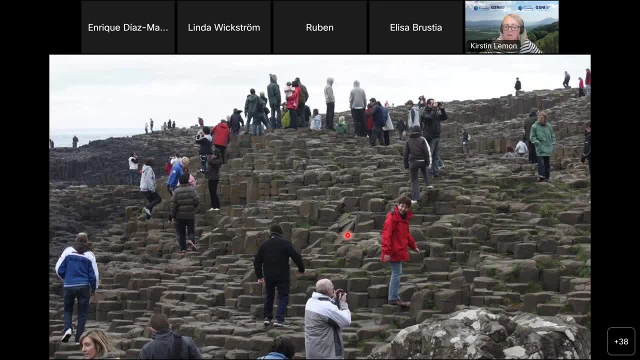 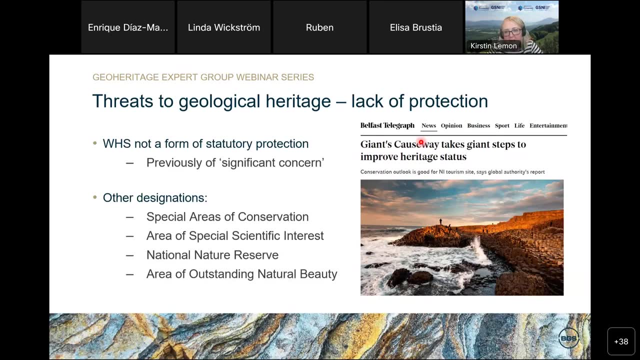 And so the National Trust is now reviewing how it manages the site, And I'll talk a little bit more about that later on. Another threat to the geological heritage at the site is a lack of protection Whenever you tell people you've got a World Heritage Site. 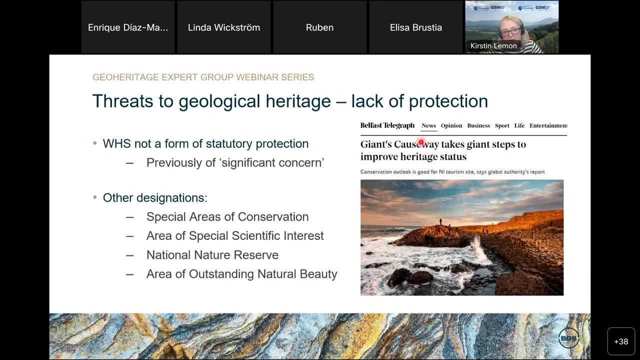 people automatically assume that that brings with it an element of protection. But the World Heritage Site is not a form of statutory protection, So there's no legislation specifically relating to World Heritage Sites. The World Heritage Site itself gets its protection under spatial planning regulations in North Africa and in the United States. 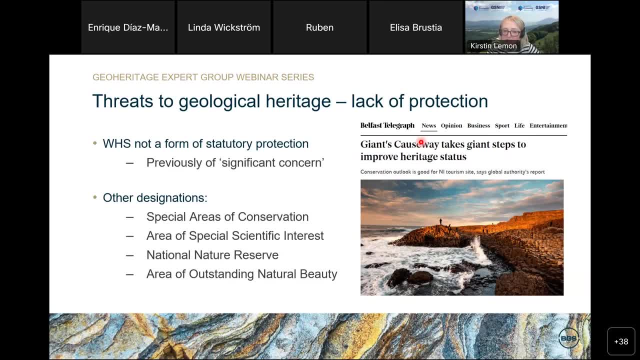 The World Heritage Site itself gets its protection under spatial planning regulations in North Africa and in the United States, And there's a millones and millions of geological archaeological occupations in Northern Ireland And considerations should be given to any development that will affect the Giant's Causeway. 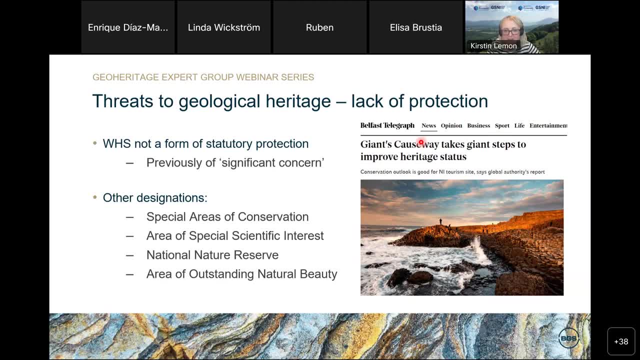 And during the Perspectives, and this actually led to serious concern around about 10 years ago, whenever the Giant's Causeway was actually cleared and really investigated by UNESCO, because there was a planned development that could have a serious impact on the site. It was previously noted as being of significant concern. 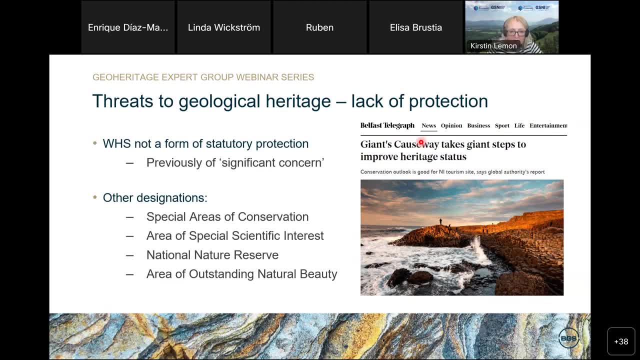 However, the development has been stopped and there's not being planned for the future, So at present we've only had. the site is seen as being of good heritage status, But that is something that will need to be looked at and could potentially happen again. 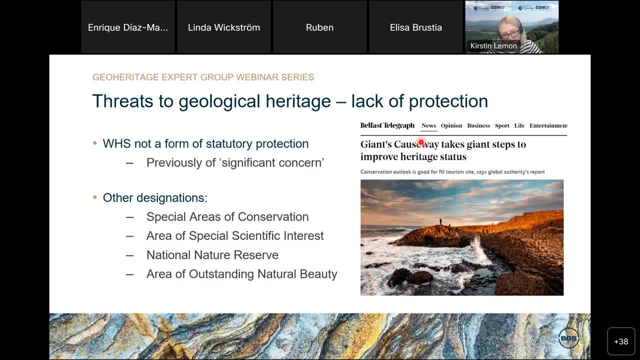 On the plus side, the site enjoys other designations, So it's got international designations in the form of two special areas of conservation: One is marine, one is terrestrial. Of course they are not for geological heritage, They are purely for their biodiversity. It's also protected under national legislation. 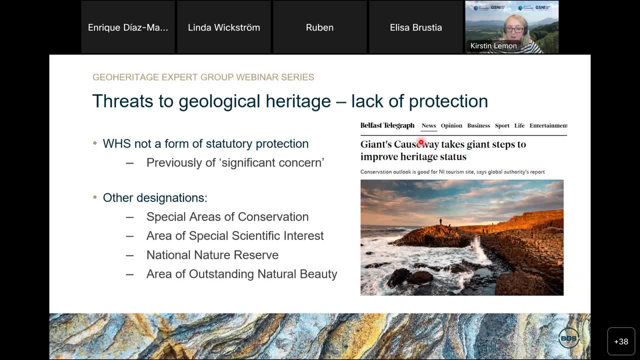 It's an area of special scientific interest, for both earth science interest, but also for its biological science interest. It's also a national nature reserve and an area of outstanding natural beauty, or certainly set within larger ones. But those two, of course, are not because of their geology or their geological heritage. 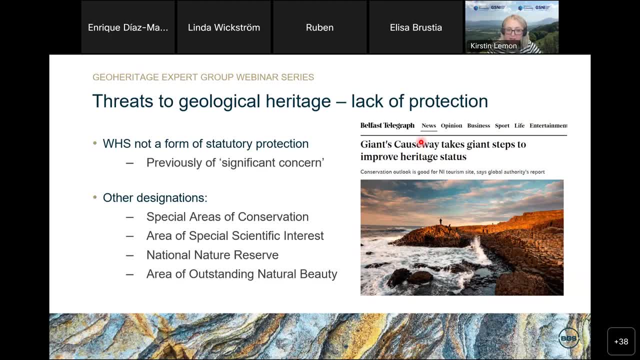 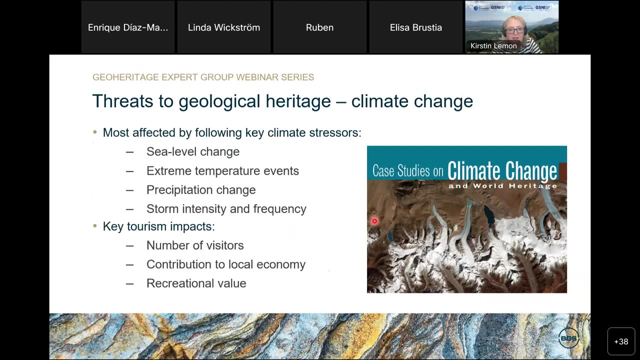 They once again are for their natural environment and for their biodiversity. So, in reality, the geological heritage does not have a huge amount of specific protection. And then another threat, and probably the most significant threat to the geological heritage, is climate change. 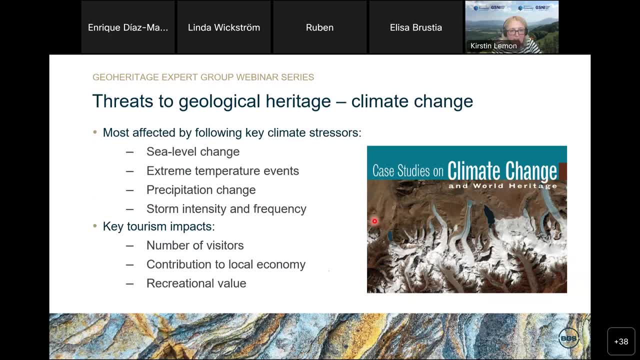 We all know about climate change. I'm sure everyone hears about climate change on a daily basis, But we've been carrying out research at the Giant's Causeway and a number of other UNESCO sites locally that are based on geological heritage, just to try and understand the impact of climate change on those sites. 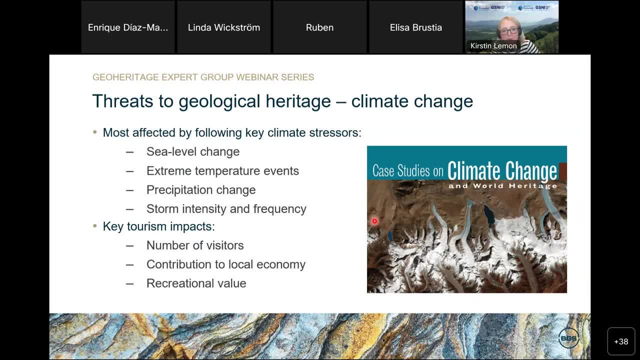 And we've identified that there are a number of key climate stressors that will particularly impact upon the Giant's Causeway. Sea level change, extreme temperature events, precipitation change, storm intensity and frequency will all have an impact specifically on the geological heritage. 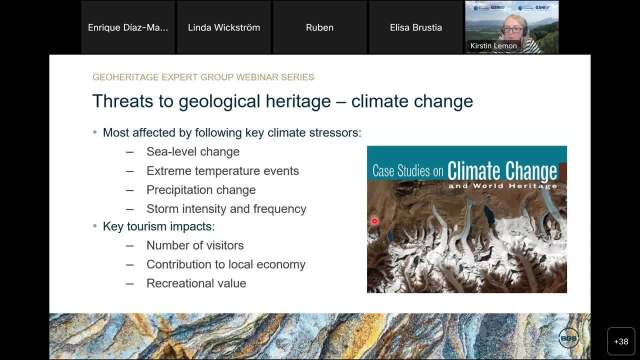 If sea level rises, we won't be able to see the columns that are actually at the shore. Extreme temperature events, precipitation change, storm intensity and frequency all lead to increased slope instability And we've seen that increase around about tenfold in the last ten years. 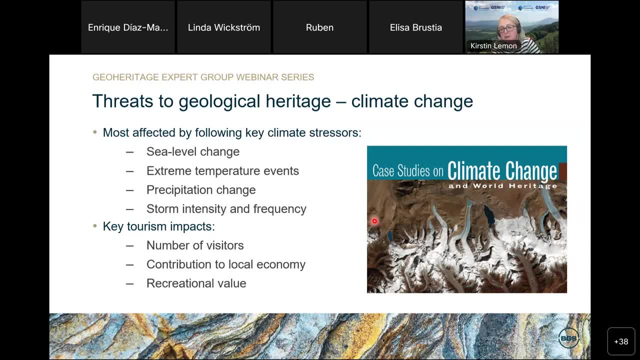 Sometimes, geological heritage is often ignored. when it comes to looking at a geological heritage, Climate change- The study on the right hand side is one that was done for UNESCO on world heritage And it actually goes as far as saying that geological heritage will not be specifically affected by climate change. 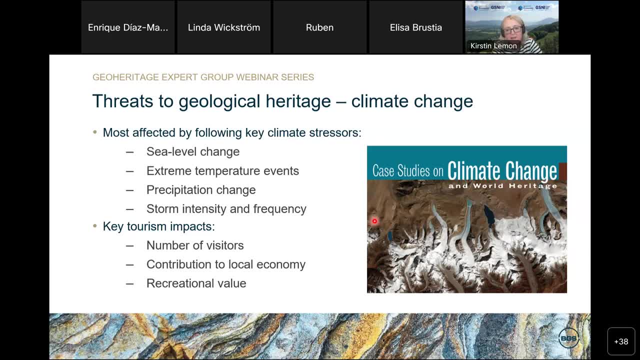 Now I know thoughts are changing on that, thankfully, But it is something that is frequently ignored And, although it will have an impact on the geological heritage, that then will have an impact on the tourism aspects of the site, It will affect the number of visitors that will be able to visit. 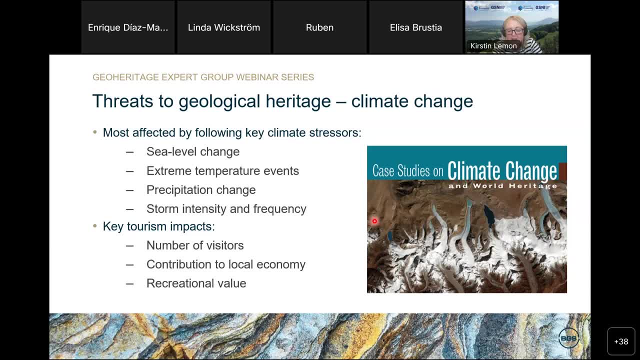 It will also, therefore, affect the contribution to the local economy, And there are lots of visitors that come to that site to enjoy the walks. Some of that slope instability will leave the path being closed, And that will then affect the recreational value of the site too. 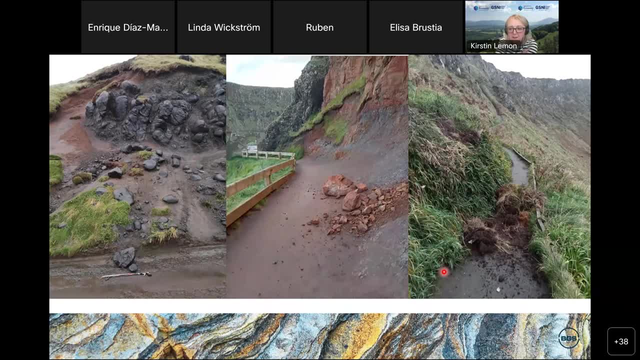 Just to show you an example of some of these slope instability issues that we are currently seeing. We particularly are seeing areas of rockfalls, So the picture on the left hand side is an area of spheroidal weathering. This is the main access path down to the causeway. 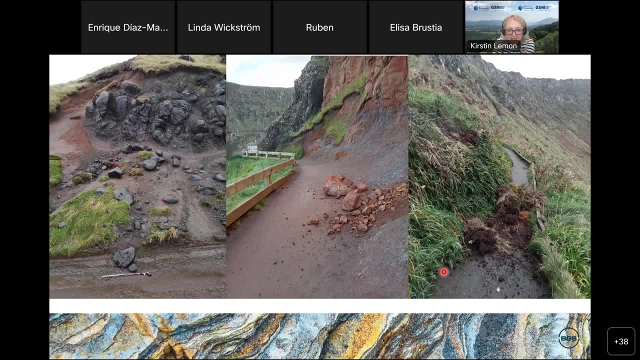 And we are seeing regular rockfalls And you'll see in the middle there. That is one of the paths around the cliff. We are seeing regular rockfalls there as well, And I don't know if you can see the gate here. This gate is actually a closed section of the path. 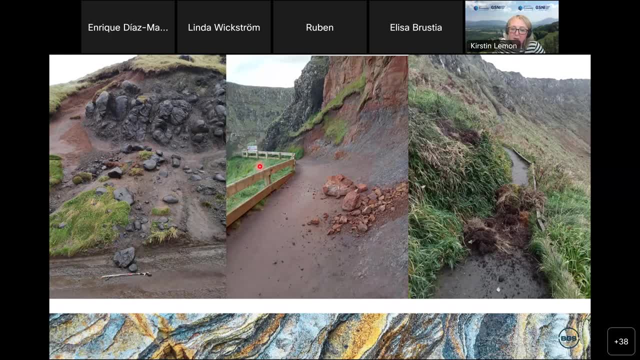 And, if you remember, I said that the path along the middle of the slope was closed in 1994.. This is because of a significant landslide, So there is a debris flow just around the corner that has closed that middle path altogether And it has never been reopened. 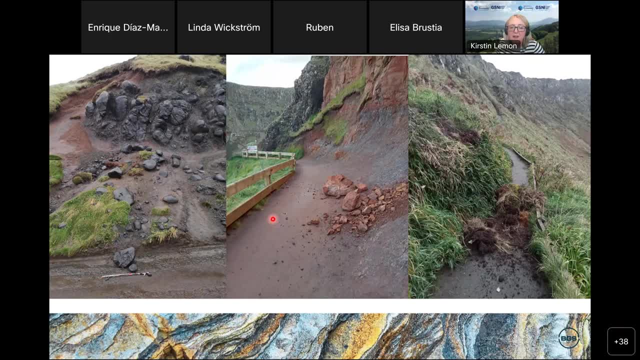 And that is going to increase and will potentially impact upon the rest of the site. This path in particular is a path called the Shepherd Steps That takes you down from the sea level right up to the top of the cliff. It is probably closed once every two months. 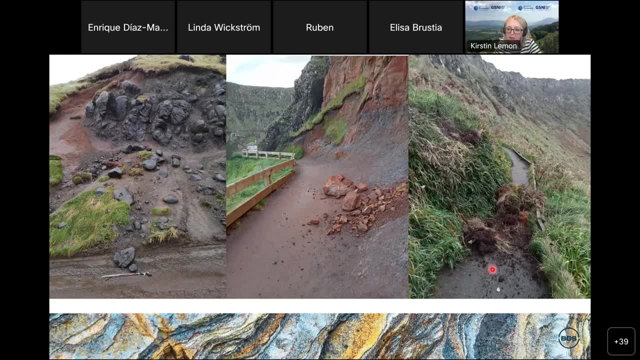 That is how frequent these events are taking place. So it is having a real impact on not only the geological heritage of the site, As it is certainly being well- I'm not going to say destroyed- Because it is a natural process- But it is certainly having an impact on the tourism side of the site too. 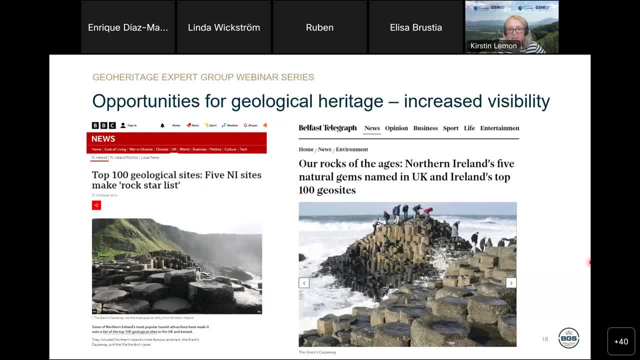 However, these are all the negative aspects. There are certainly opportunities for geological heritage through geological tourism at the Giant's Causeway. The Giant's Causeway is undoubtedly our most iconic geological heritage site. I would go as far to say as it is known all the way around the world. 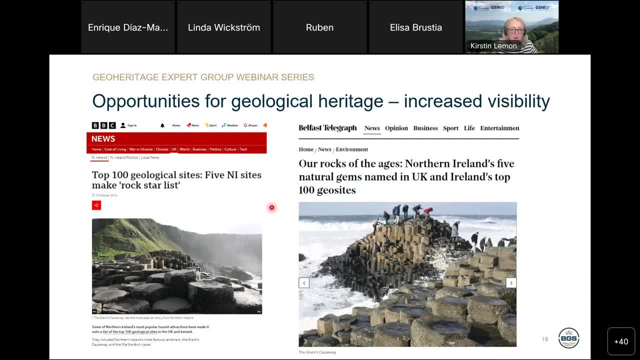 That means that we have a really good opportunity to promote geological heritage in Northern Ireland, But all the way across the UK and Ireland as well, Through the Giant's Causeway, And we have done that. So the pictures on the screen there are from a project that was done by the Geological Society of London. 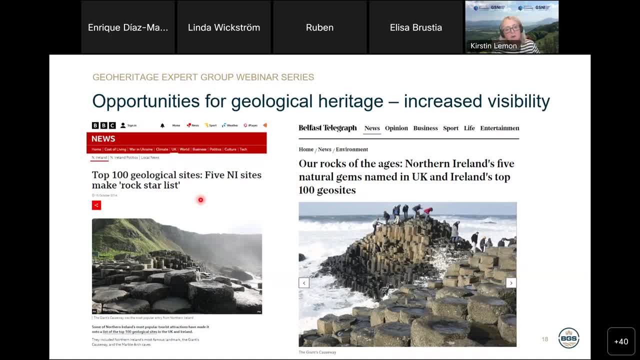 Back in 2014.. The idea was to identify the top 100 geological sites across the UK and Ireland And, not surprisingly, the Giant's Causeway came out as one of the top sites. However, there were five sites in total in Northern Ireland identified. 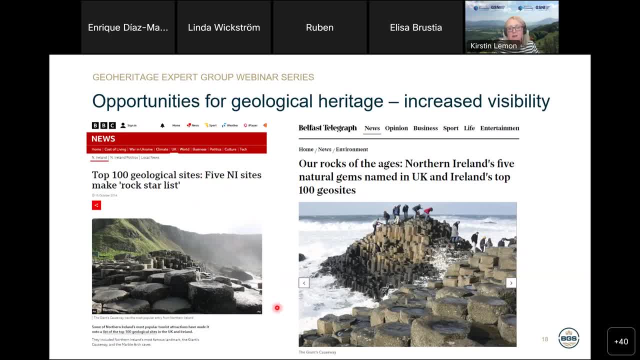 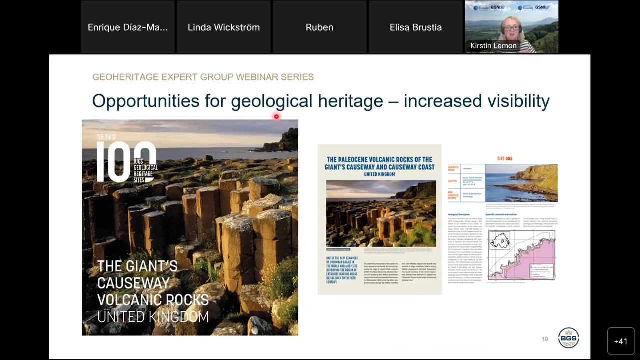 And by using the Giant's Causeway images, it meant that we were able to promote all those other geosites as well, And not only the five in Northern Ireland, But all of those across the UK and the rest of Ireland too. We've also seen this in the most recent IUGS top 100 geosites project. 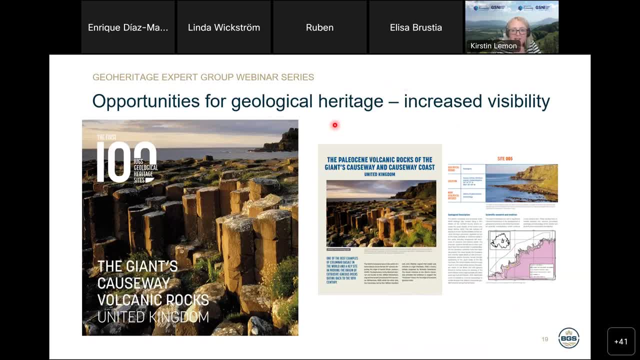 Because the Giant's Causeway was number five in the sites in the book. Not surprisingly, because it is an iconic site for geological heritage. It was in the section under the importance of geological heritage for geological science Because it was one of the sites that helped to prove the origin of igneous rocks. 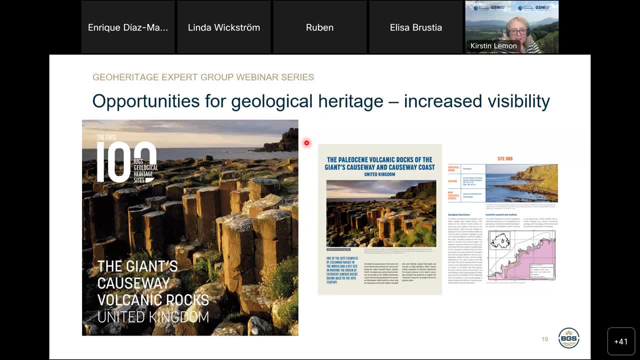 But the fact that we were able to get it in there as number five. It is one of only four in the UK And the only one on the island of Ireland that made it into that book And it actually got a lot of attention locally. 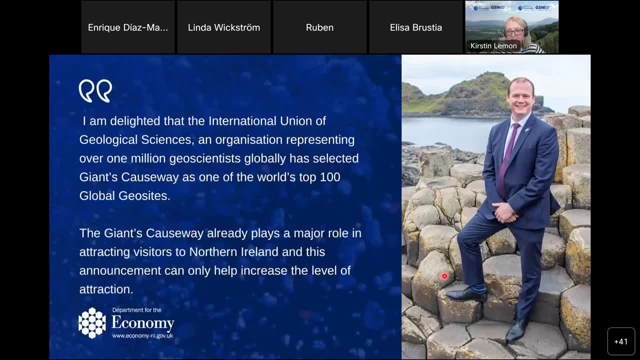 Particularly amongst Northern Ireland government officials. So this is a picture from the Minister for the Department for the Economy, Who really put out a statement, And this was put around all social media and all the news around Northern Ireland And we thought this was really particularly good for us. 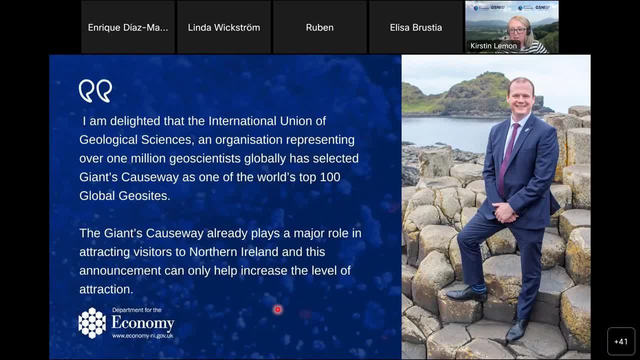 Because sometimes when you're sitting within the Department for the Economy As a geological survey, you sometimes get ignored. But whenever you can get your geological heritage to have an impact on the economy And actually make ministers see how important that is, That's really good for us. 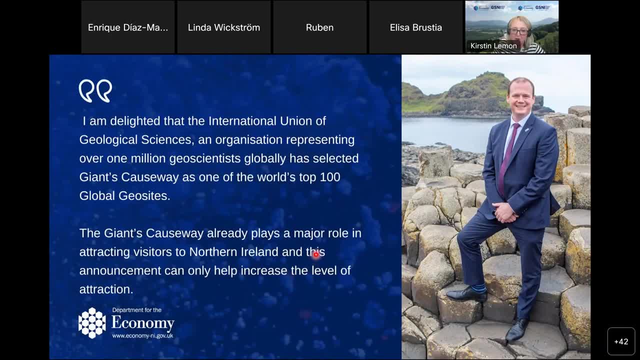 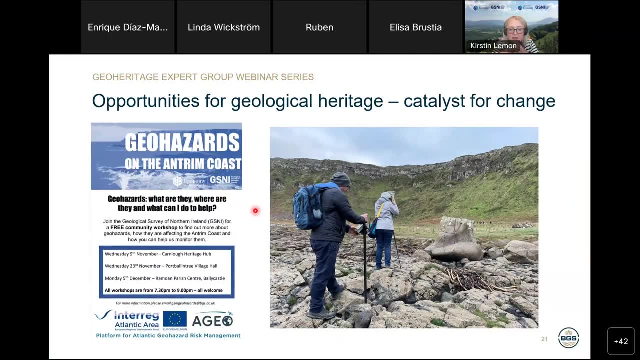 And helps people to understand geological heritage and its impact on the economy as well. And then my final section is to talk about how we can use sites like the Giant's Causeway as catalysts for change. I've already mentioned that it is a fantastic tourist site. 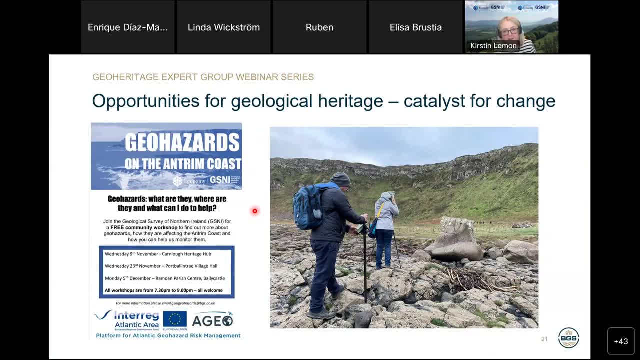 But what I haven't told you is really the amount of impact that this site has for the Northern Ireland economy. So I'm just going to read you out a number of figures. So the Giant's Causeway in 2019 contributed, or certainly helped to generate, £484 million for the local economy. 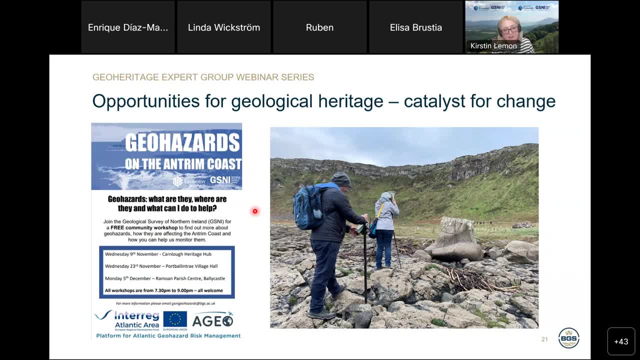 It paid £1.5 million in wages to local people And at the visitor centre, the shop that they have, 80% of the crafts on sale were from the local area, So it will give you an idea of the significance of that site. 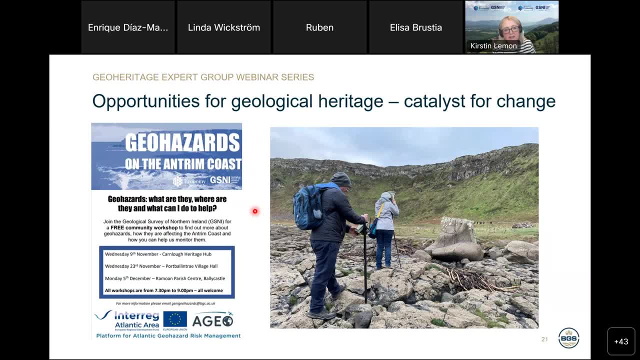 So whenever we see issues at that site such as geological hazards And we can tell people that they're going to have a real impact on the economy, It does make people sit up and listen. So it really allows us to have, if you like, a platform to carry out work that we might not otherwise be able to do. 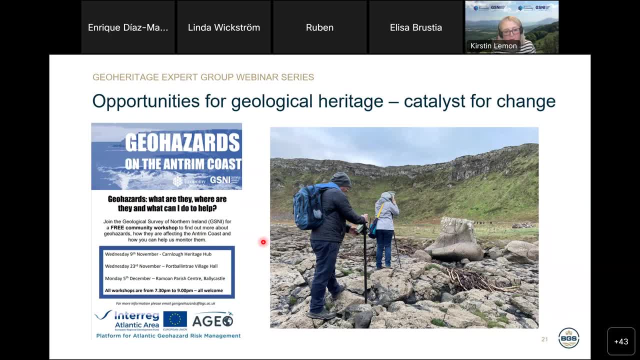 One of the examples I put on the screen is a project that we are involved in called AGEO, Which is a look at geo-hazard risk management. So we are working with a national organisation, A national trust, to monitor the site, To help to understand the geological hazards. 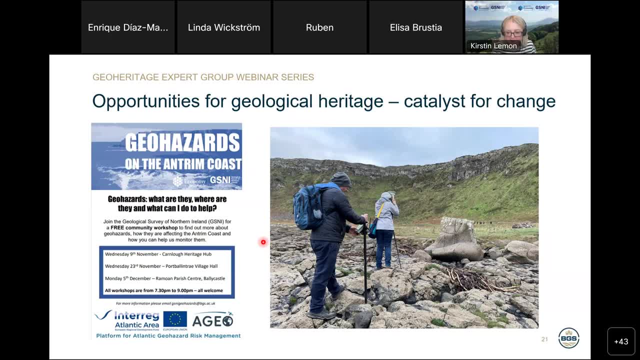 What their triggers are, How we can contribute to risk management, And in doing so, it's helped us to better understand not just the Giant's Causeway, But the wider area of the Antrim coast. It's also given us that, if you like that visibility. 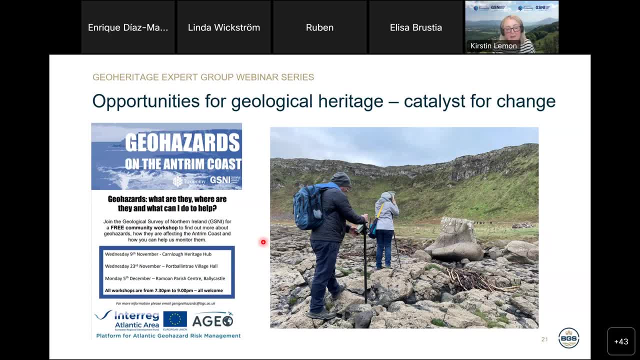 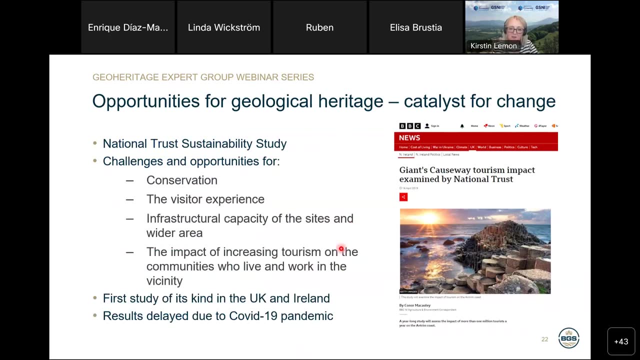 If people see the causeway, they're automatically interested, And this in turn then helps us to better control the impact on tourism as well. And then, finally, my final slide is just to mention The work of the National Trust. So I've already mentioned the fact that the National Trust are rethinking the way they operate. 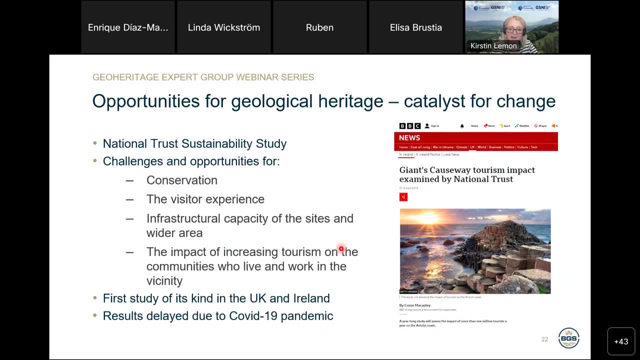 By looking at geological heritage And by looking at the impact that lots of visitors have. It gives us a real opportunity to really think about how those two work together And how we can better manage those sites, Because we do still want people to visit. 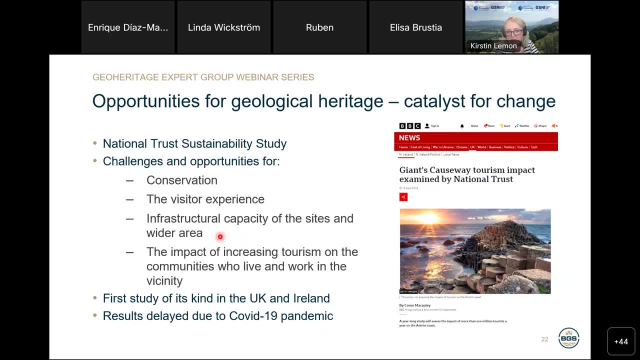 We want people to appreciate and enjoy our geological heritage, But we want them to do it and not have an impact- Or certainly not have a negative impact- on the site. So the National Trust have commissioned a sustainability study. It's the first study of its kind in the UK and Ireland. 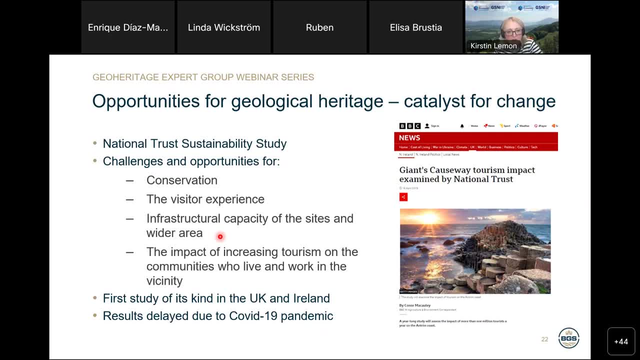 And the idea of it is to identify all of the challenges and opportunities For conservation, For the visitor experience, For looking at the infrastructure capacity And look at the impact of tourism on the community And also on those who live and work nearby. 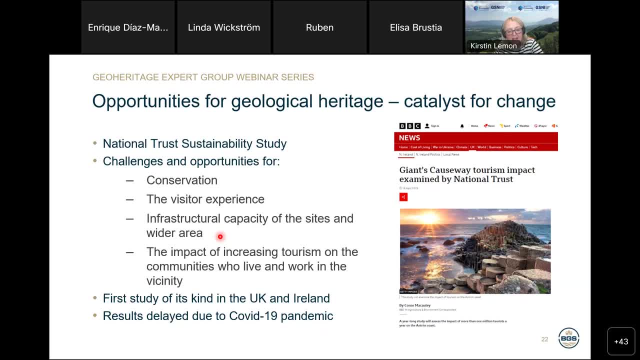 Now, this work started in 2019.. And the results have been delayed Due to COVID-19., But we are really hopeful that the Giant's Causeway in particular, And the National Trust can really act as, if you like, A pilot site for other sites. 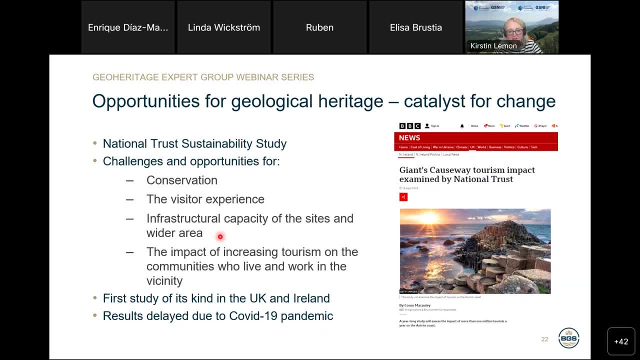 Of geological heritage in particular, But also natural heritage, So we can understand how to better manage them. Looking at the geological heritage And understanding how it is impacted by visitors And how we can make sure that people can still visit in a responsible way. 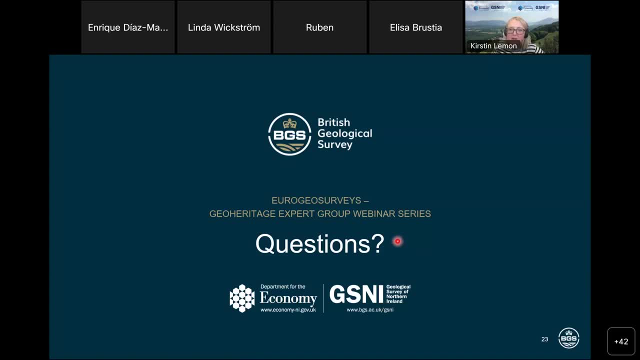 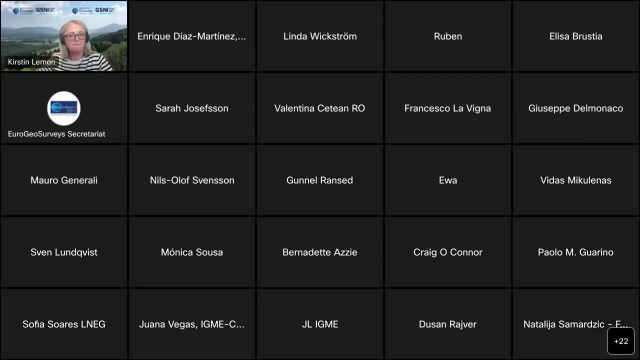 Well into the future, And I'm going to finish up there, So thank you very much for listening, Thank you. Thank you very much, Kirsten. That has been really nice And I think all three are very good examples Of how us from the geological surveys. 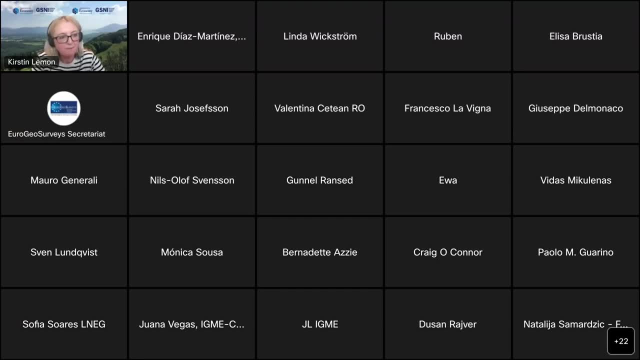 Can contribute really with all the different aspects For the management of the geological heritage And how we can contribute to society, Which is the main objective of this webinar series. I'm sure there must be questions. I have not looked in the chat. 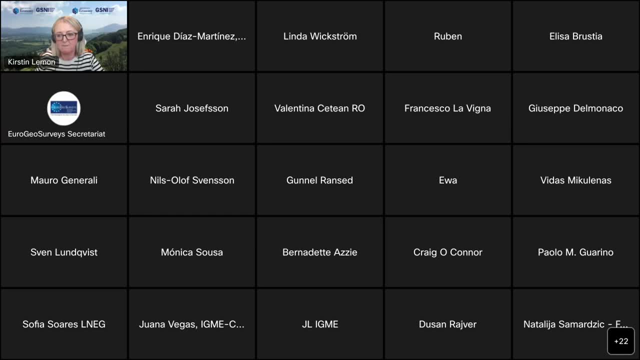 And we will open also for the folks who are watching. We already have, let's see, 47 persons here And I don't know if you can do make your questions written in the chat, Or I suppose there will be no problem to open the microphones. 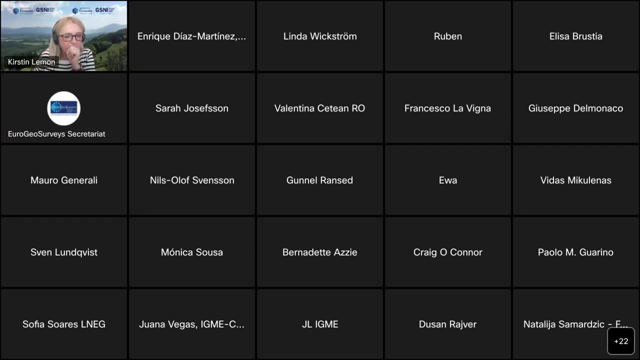 Always with due respect to all the audience And to the speakers. I already have some questions, But I think it's better if we open for the participants from the public. If you want to, If anybody raises their hands, And if not, I will go ahead with some of the questions that I have noted. 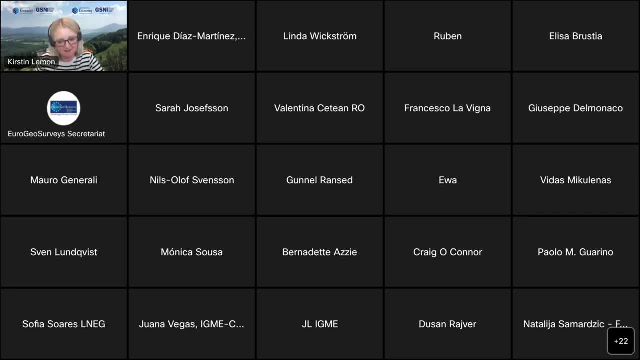 For example, one question I have to begin with- This is for Elisa In the first. If you can open your cameras, Linda and Elisa. Elisa, I would like to ask you For the future of these trails and panels that you have designed. 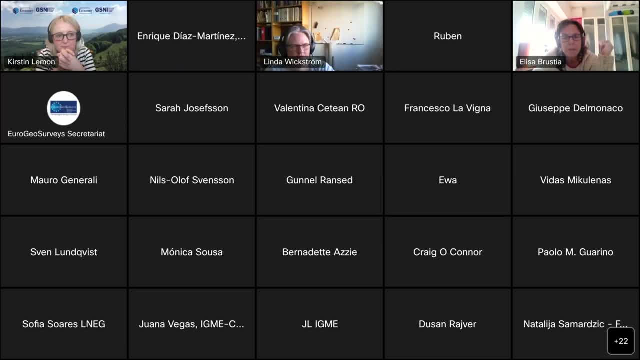 This was previous to the pandemic, as I understood. no, Yes Because, for example, the marks- Let me turn on my camera. Sorry, I didn't, I thought it was. I'm curious because you have used the space that is clearly white with no, no lichens. 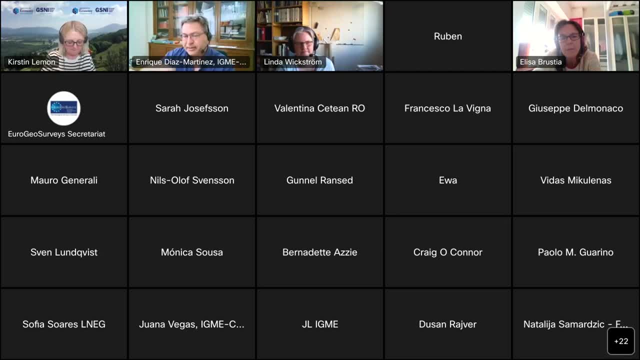 No most know any vegetation that has resulted from this latest earthquake, And this will also, with time, be recovered by the vegetation, by the most, by the lichen, And so now it is very clear, because it is very recent, Just a few. 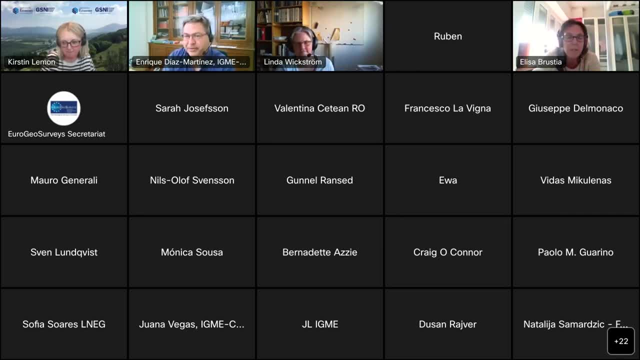 Yes, it's very it's very recent, but it will evolve. So my, my question in particular is: What are you planning? Are you planning to clean the surfaces? Are you planning to Mark with a line, or or what will you do in with time? 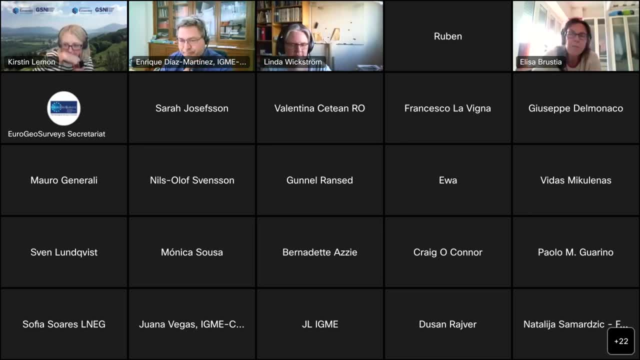 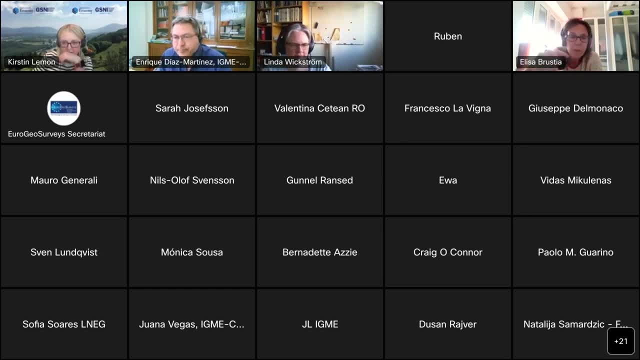 One, one um plate where not not we but but the the park was to pluck first and late in, later the earthquake they played. there was a photo and another another. another activity is to put a special, a special resins that is possible to use also for the monuments to preserve from the 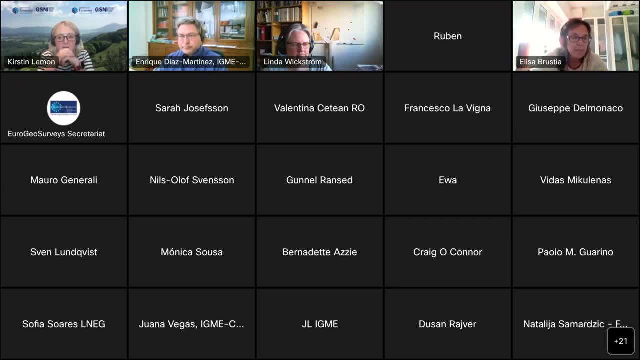 from the pollution and and the lichens and others, only for for a little, a little space, one meter for example, to put on the on the surface faulting, and it could preserve the, the white. okay, so you are planning for the future to how to manage this, because i suppose that for the 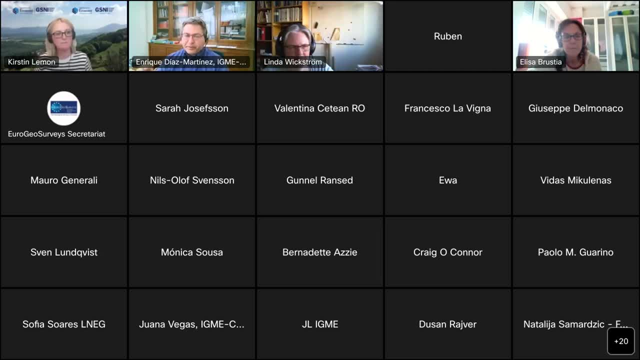 visitors. that is the most clear evidence that when you look from the distance and what you get closer and it is important to to manage when the process, when the geological process takes place in between periods, and that, yes, because now is- is so clear, so wide as is possible. 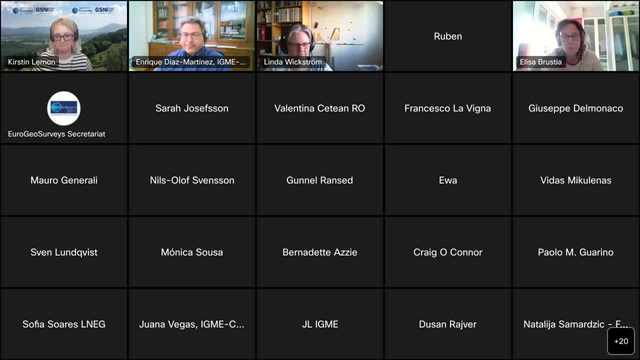 to to observe also too far, but in i don't know, 10, 20 years surely became the same. the rest of this, yes, okay, so that's also important if the cities are closed because you have something like that we are dying to find for a member of a large number of pages. we, we sugarcoated the context. 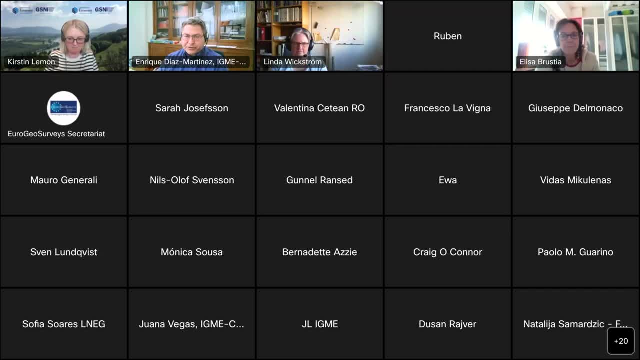 and we also need data which we can use by by saying: check the time we can we see. so just also to soft to decide we, i would guess from. i'm happy to do that. so i have a question that asks if, if i have done any special studies to 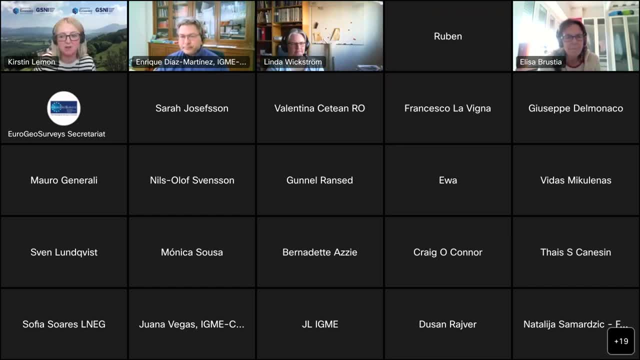 estimate the impact of projected sea level rise over the next hundred years, so the figures that i've been using are based sorry. so the figures i i've used have been based on those that are projected by the meteorological office or the met office in the uk and those that are being produced as part of the uk climate. 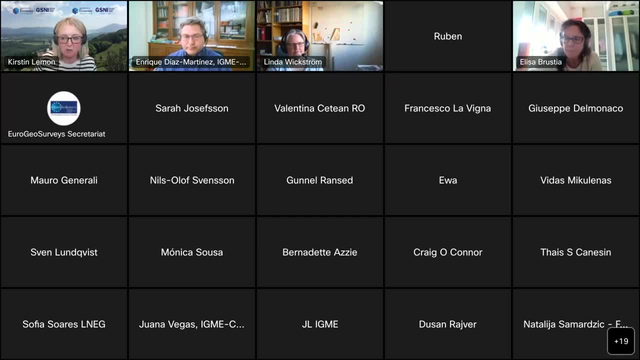 projections, and so they're the estimates that we have used. and then there's another question is: um, are you planning any special management action in this way? so there's no specific action. however, we are working with the national trust to develop climate change adaptation plans, so this: 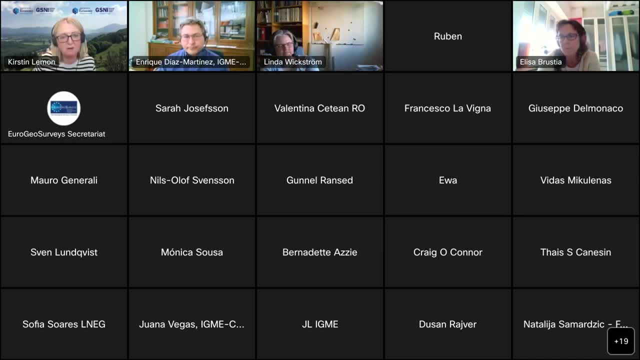 and was based on a research project that was carried out to fully assess the impact of climate change on geological heritage sites and also to assess their ability to adapt to climate change. so there are recommendations produced as part of that and we are working through those recommendations. if anybody would like to see that project- um, i can- i'm happy to send that home. 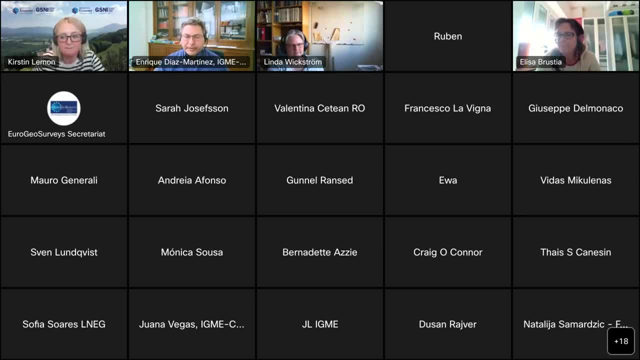 i. i suppose that every everybody will be interested also. i mean, apart from, uh, the reports that you are doing or that you would like to do, the the special interest would be also: what would you suggest in in case you would have money or in case you would have sufficient time? what do you think would be proper to do in this type? 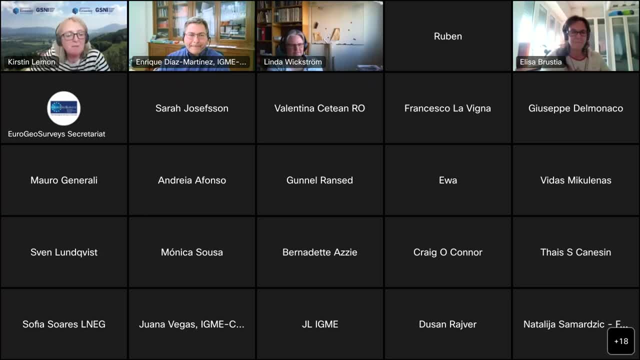 in these cases. so that's a really good question, because the national trust is a conservation charity, so they are not very keen on, i suppose, putting any hard engineering solutions into the coastline. they see the coastline as being dynamic and i think that is a very good attitude to take because, as we all know, we're not going to be able to stop climate change. we 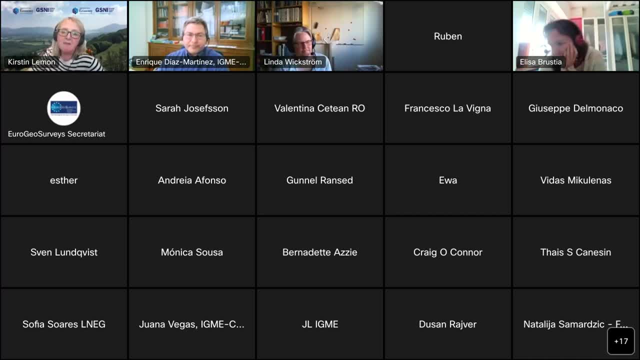 just need to be able to better live with it. so i think i can't really answer that at the moment and, ricky, i think we just need to sit down with the national trust and work out how they're going to deal with climate change adaptation. i suspect it will be dealt with through looking at um. 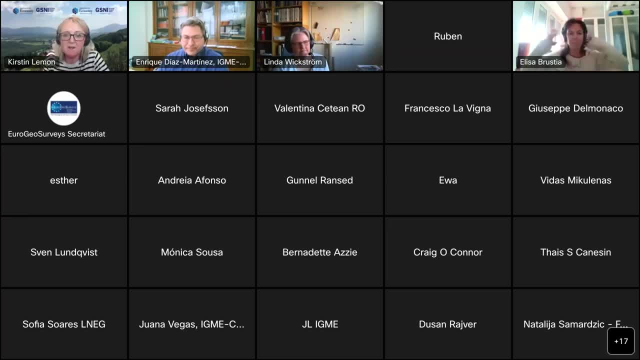 better site management, maybe redirecting paths. it'll also be done through education locally, and it'll probably also be done by maybe looking at some nature-based solutions, but i need to talk to them more first. i will maybe get back to you in about a year's time. 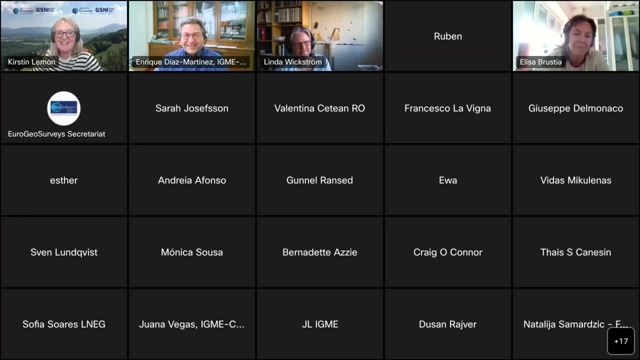 okay, we will have more webinars in the future, exactly updated, and i also have i. i don't see any more questions in the chat, so i i would go for for linda one question, because, uh, you were saying that i mean there's these three main the, the waterfall, this all this very old tree. 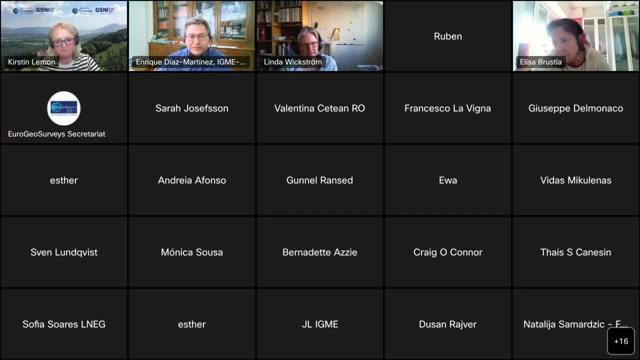 and the rain disaster that are the the most of the biggest interest for the tourists that are going there. and then they ask these questions about the rocks that you are trying to to support the, the guides there at the national park so they can respond properly, and i i suppose this. 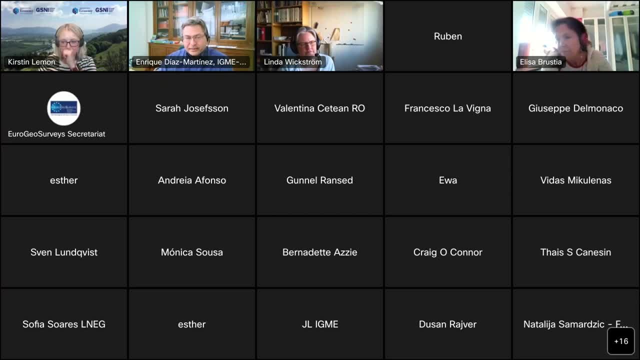 is: uh, this is only- i suppose it is not only- this national park. so i would like to know how the geological survey is supporting in general the the needs that come in similar respects in the protected areas in sweden, and if this is working or helping at all. 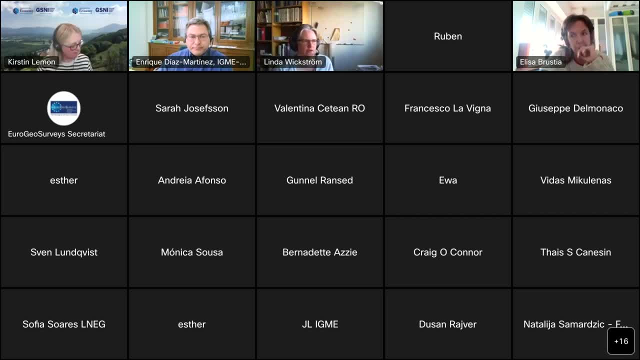 we, we don't do it automatically. uh, we just work with these questions when we have external funded uh projects today, unfortunately, uh, it would be very nice to have um a budget within the survey that we, so we could work better with the, the environmental agency, for instance, which is the, the. 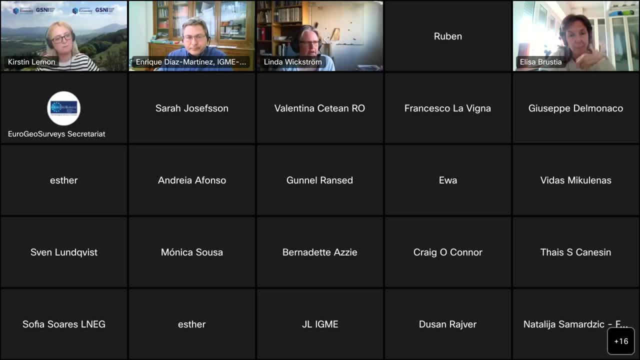 the organization responsible for all the national parks. um, the good thing with these, these projects projects have been that we have had a very, very good con contact with the county administrative board, which is the local organization working with the protected areas and the national parks within their region. so we have learned a lot about how they, how their work is done. 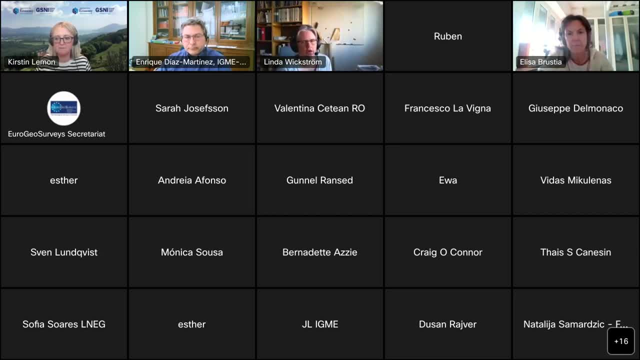 and under what conditions they have to, to, to work, and quite often when we talk about geology with them, they become quite happy because the the I mean to to protect or not to protect, but to preserve a, a geosite. in some cases it's actually easier than than. 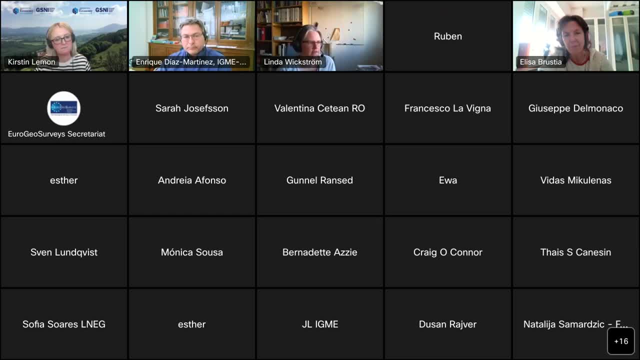 than conservation and preservation of a biological site. so when, when you tell them that, well, you can actually go quite hard on this rock site with a brush, then they are happy and they can take away trees, they are happy as well. so I think we have taught them quite. 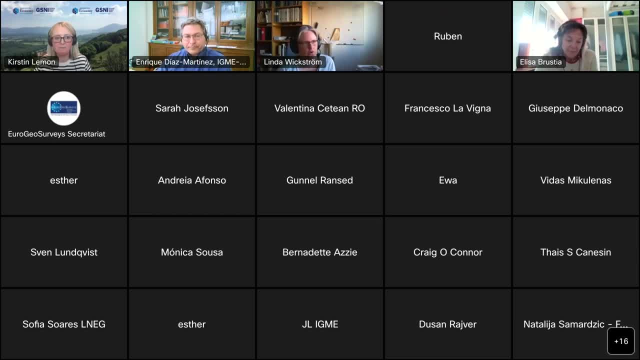 a lot about how geology works in these projects and we hope that they can actually take that further on to to their colleagues. okay, and one one more question for for you, Linda, because at least in Spain, we have had many examples of problems with the management of protected 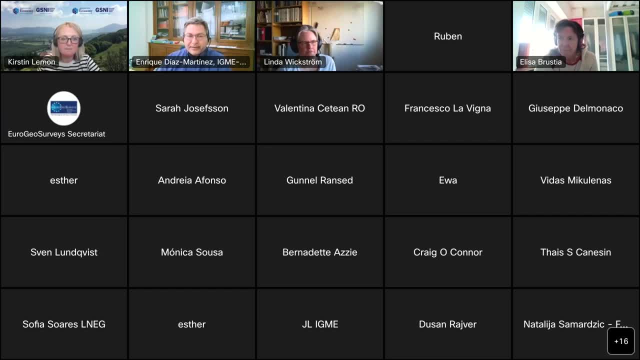 areas when you have a viewpoint. the vegetation grows, the trees grow and there is. you don't see any more the landscape. I don't know if you have had this case. I think in the giant's causeway there's not so much, not so many trees, but I I noticed that in your national park, and probably also Elisa. 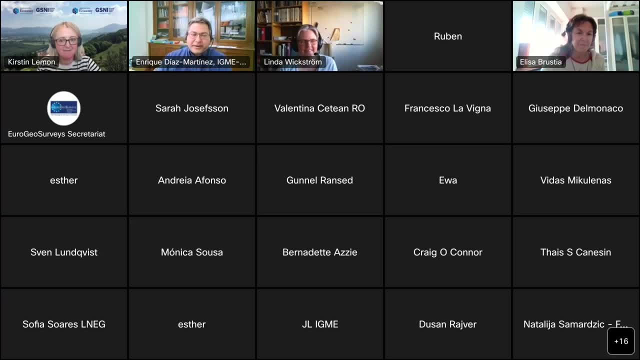 may have a similar issue with the vegetation growing and then you have to tell the park to cut trees. yes, growing vegetation is is a problem for for landscape views. yes, we have some examples of nature reserves in the Dalarna region where we were talking about- because that's it was a- a- a canyon, a quite small canyon in limestone, so there's a lot of vegetation. 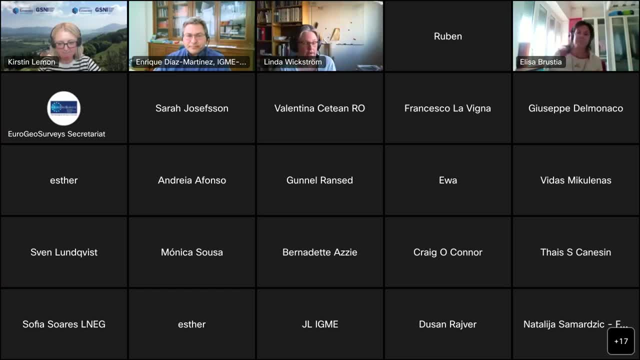 and today quite large spruces, for instance. but the good thing in that case was that the, the management, also wanted to take away what it supposed to this particular landscape. certainly strength with you can actually cover stuff a lot more. okay, thank you and your work. youization was great. 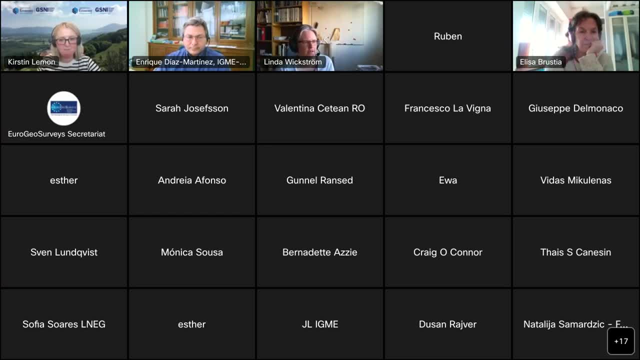 thank you, muy bien, thank you, and so just a little bit really special questions for you花 now. all right, do you have there some? do you have uh, like fairly great questions and a few examples? uh, so, are you interested in to take away the spruces, because they weren't really supposed to be there, So we could sort of 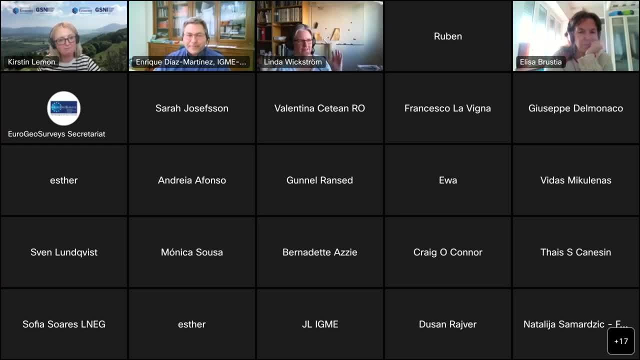 take that spruce and that spruce and that spruce, and then you can actually get the shape of the canyon. So we were quite happy and they were also happy. So then the conclusion is that it is possible, always under agreement and with having a common objective. I suppose, Yeah, I think. 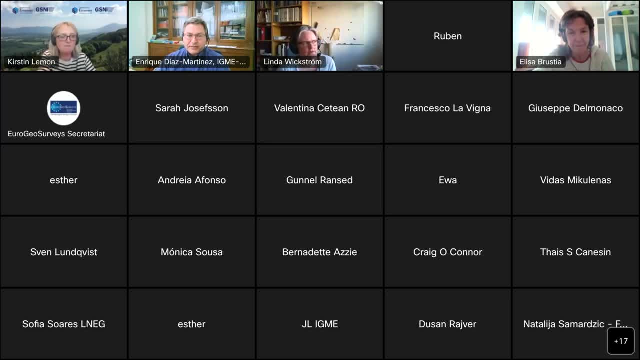 in many cases, it's all about trying to explain to them why. because they just don't have sufficient knowledge about geology and what's hidden. Elisa, do you have any comment regarding this management for the viewpoints, because I noticed you have some panels but I didn't see. 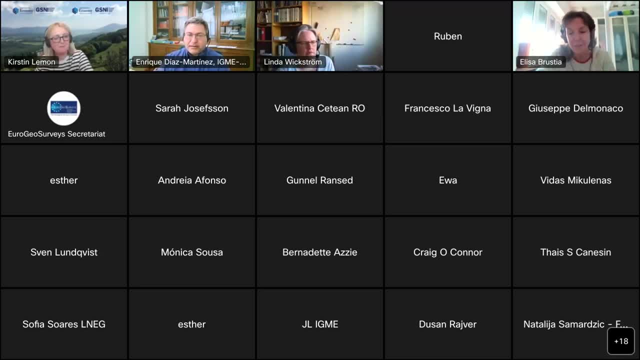 many trees in this. Fortunately, in this area there aren't. Is the vegetation very, very little, Only rocks and there aren't trees. Is that zone very, very clear, very clean from vegetation? Well, the vegetation is not dirty, but it's, I suppose, a problem with. 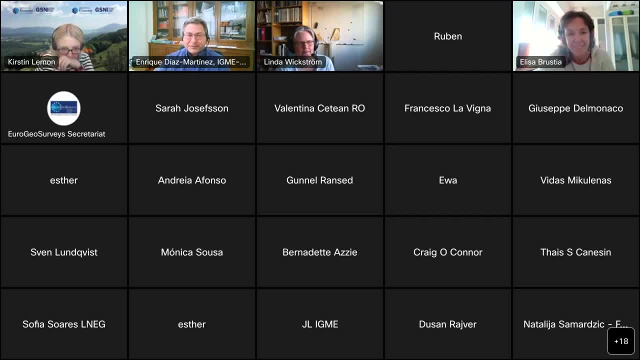 the priority It is in the management, because there are examples when you have lost the purpose of the viewpoint. Yes, yeah, clear. Maybe. Kirsten, do you want to add anything regarding this problem with the viewpoints and the management? We don't really have any problems with viewpoints, certainly not. 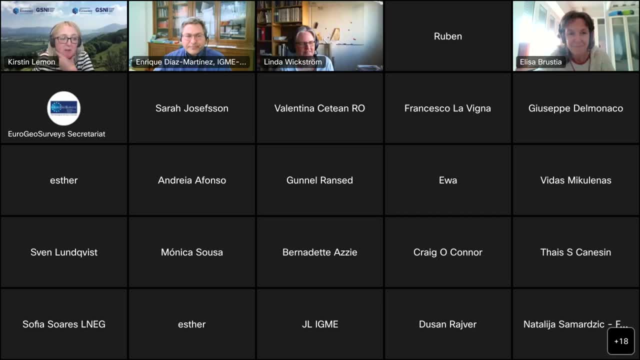 from vegetation. The only problem with viewpoints we would have would be too many people, not plants, Too many people. So what are you doing in that case? How do you control? do you limit the number of people? Do they have to make reservations? So they do now. So prior to COVID. 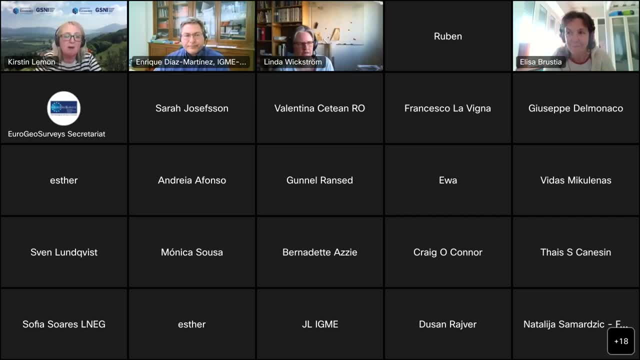 there was no reservations needed at all, but now you do have to book and the National Trust are struggling, I think, financially, as a result, because they did depend on on the money from visitors, not just to fund the Giant's Causeway, but actually the money that came to the Giant's Causeway helps. 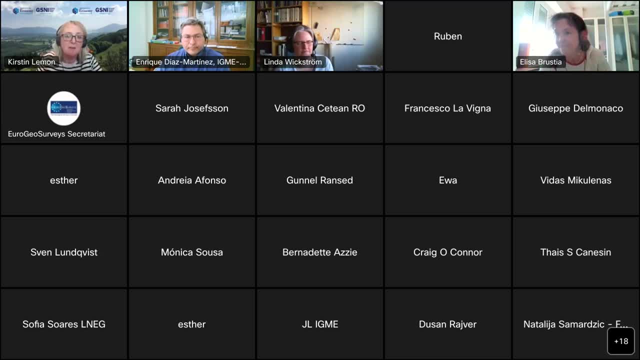 other National Trust properties across Northern Ireland. So it is something there they're. they're going to get a balance as to whether we have more visitors or more money. So yeah, it is. it is a bit of an issue, but no problems with vegetation, except a little bit, a little bit on the stones and that. 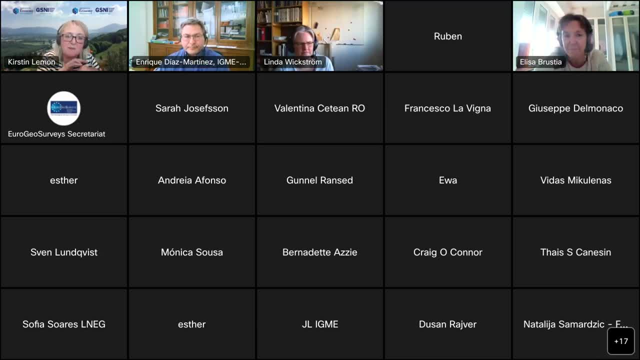 they mentioned were brought in on people's shoes. You get seeds brought in sometimes, and but that's that's really it. Actually, there is a question from from Thijs Canessing regarding this. Yes, so with regards to the carrying capacity, that is something that's being looked at as part of the 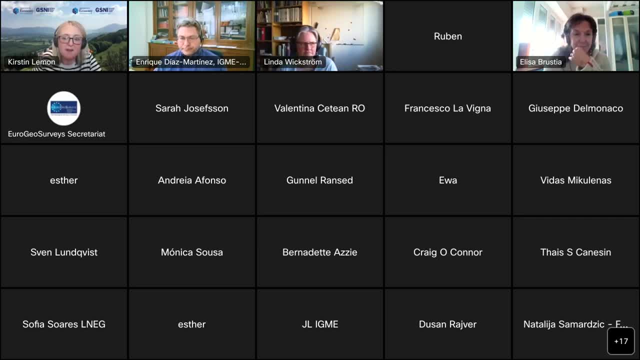 sustainability study. that's being done at the moment. So that is being looked at, very much so for the Giant's Causeway and the adjacent site of Cargaread, which is another geological heritage site. So they're looking at what the carrying capacity is, what the optimum visitor number. 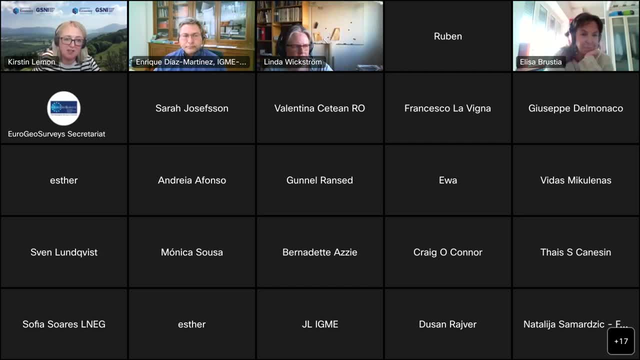 is, and then they're going to produce recommendations, but that is not completed yet. It's been delayed because of COVID. so but it should be out soon. And I suppose something that you mentioned, which is with the climate change in the. in the last decade there has been a lot of 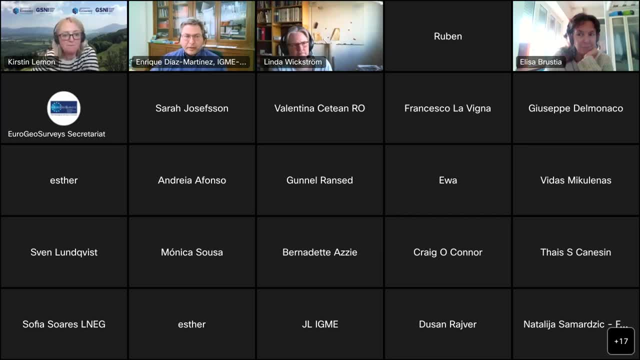 discussion about how to replicate all this increase of the slope processes and the rock falls and all this that generates problems for the accessing the or to, for the itineraries, and all these things for the management of the public use. I suppose, Yeah, that's having a really quite. 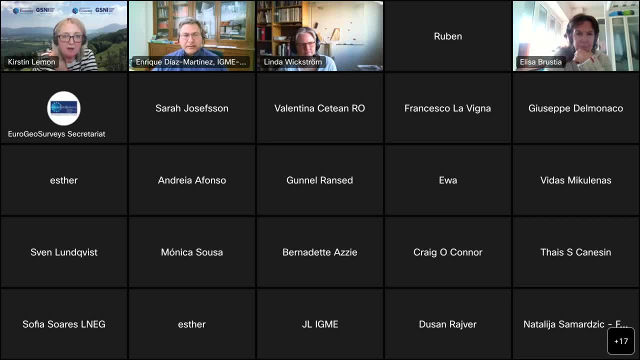 a big impact and the project I mentioned there, the RGO project. whenever GS&I originally got involved in that project, we actually had another site in mind We had which is out to the west and it was looking at peat slides instead. but before the project started, 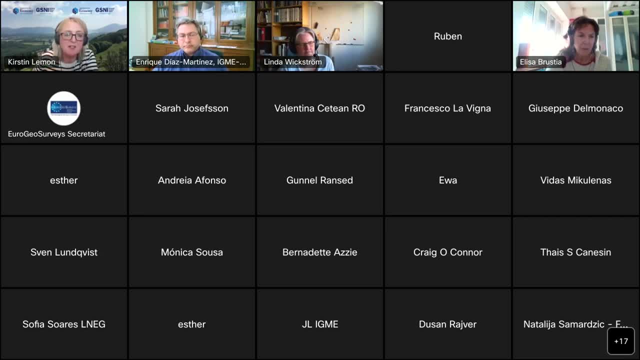 we were getting calls from the Giant's Causeway and the National Trust basically on a monthly basis because of landslide events. They wanted us to come and look at them and tell us what, tell them what to do. So we actually changed the pilot site from Quilker Mountain in the 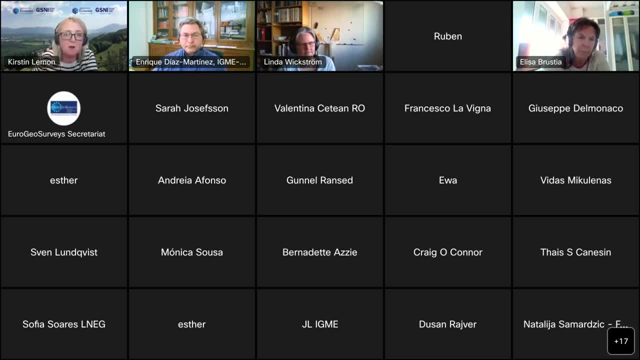 west to the Giant's Causeway- because we reckoned that it was number one- have a higher impact because it was going to help us to understand what's happening in the key tourist site, but also it would help people to listen to us. so certainly the tourist tourism and 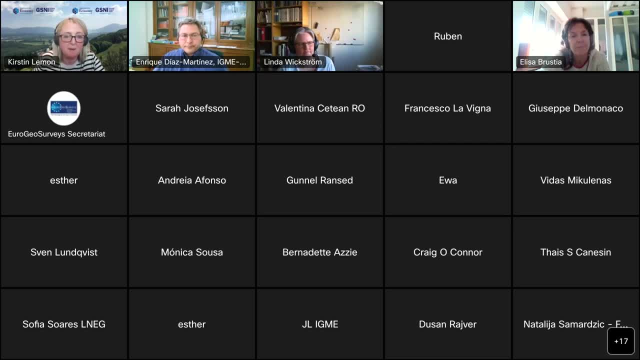 I, you know, if we're doing work at the Giant's Causeway, they will perhaps listen to us now. So yeah, it is. it is quite, a quite a big issue and it's increasing. We've seen it increase even in the time of the project. Yeah, one of the things that we are hoping through this, through our 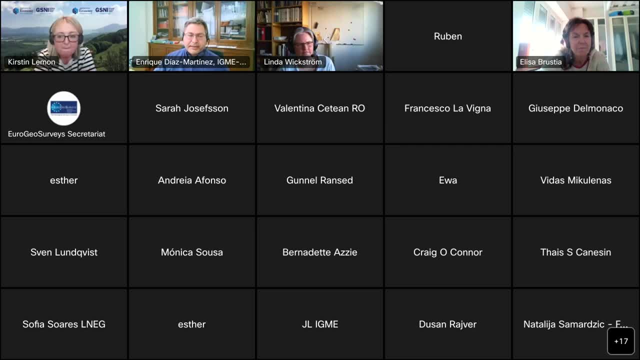 geoharitage expert group of the Euro-use surveys is to be able to include in the map that is available in our web also our all the geosites so that the tourism companies, agencies and the proper the national governments are or the local authorities can see what geological heritage they have around that they 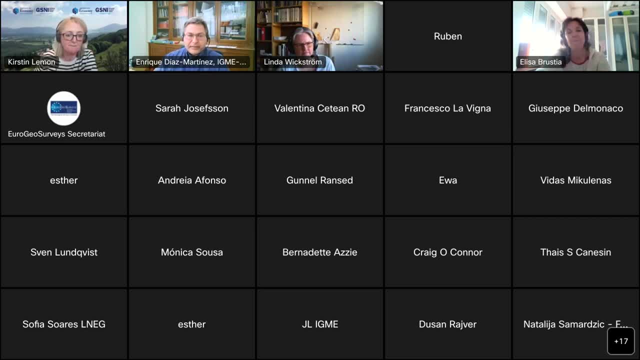 can use for the, for the tourism, And so in this respect I would like- I don't know if any of you three would have any comments regarding- in particular, when you propose sites, do you specify also if a site is more presentable or if it's not presentable? If it's not presentable or if it's more. 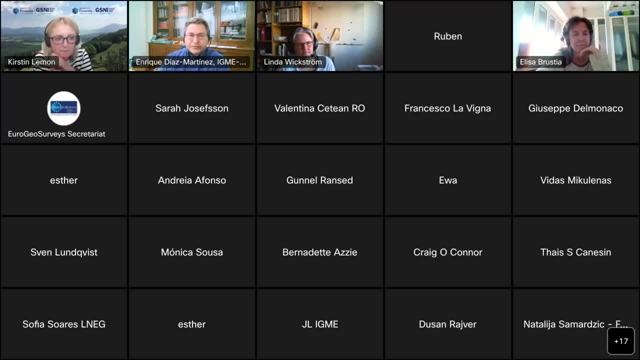 proper for education, for tourism, for science, for any of those. So normally I would suppose. but is this? has this helped with the tourism development? I don't know if any of you wants to respond in in your particular case. So, Enrique, do you mean in your communication with the tourist? 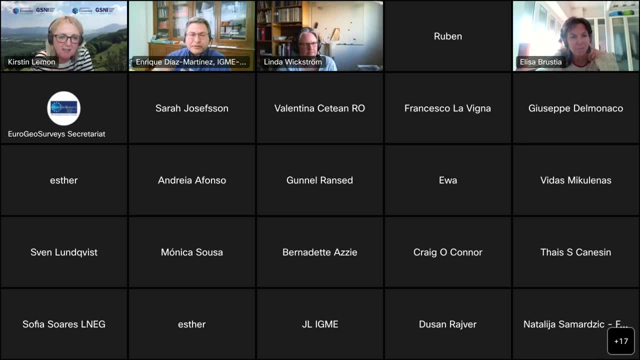 bodies? Do you specify whether they're useful for a certain aspect? More than towards the tourists, they just will adapt to whatever is. you know what they need. I mean particularly with what you provide to the administrations, to the government. 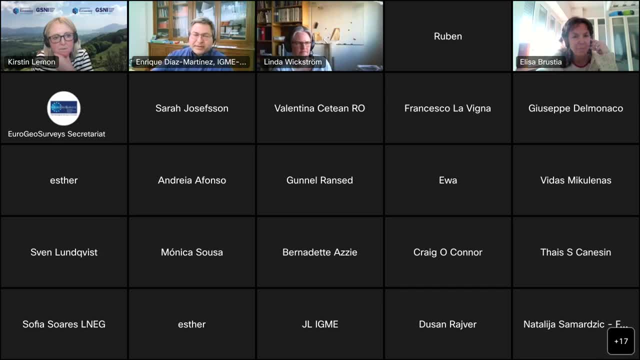 to the local authorities. do they know about the sites which are better to be promoted for for the tourism Just, I suppose, on our behalf. if I was ever speaking to local councils in particular about tourist sites, I would generally only talk about ones that are with public access, so are suitable for. 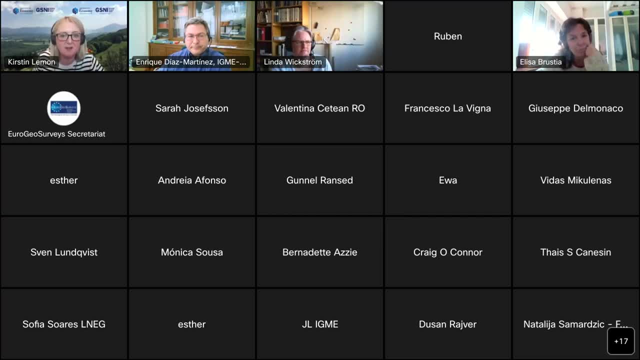 tourists. therefore they've got amenities, car park trails etc. And I generally would not promote any other sites. but that's more to do with the issues that we have here in Northern Ireland with landowners and access to land. I'm not entirely sure what it's like in the rest of Europe. 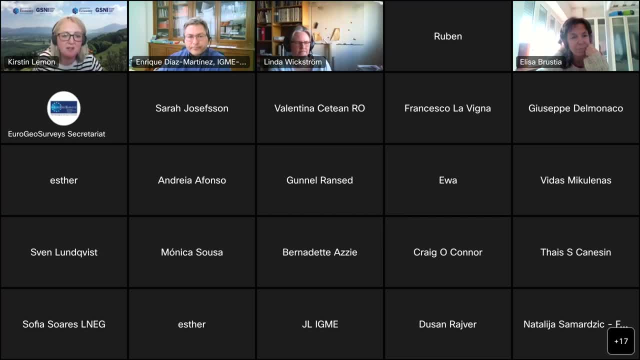 but we are not allowed to walk in anybody's land without permission. I know other parts of the UK are different, but in Northern Ireland we're not allowed to, and that's why I do that. Okay, How about you, Linda, In our new 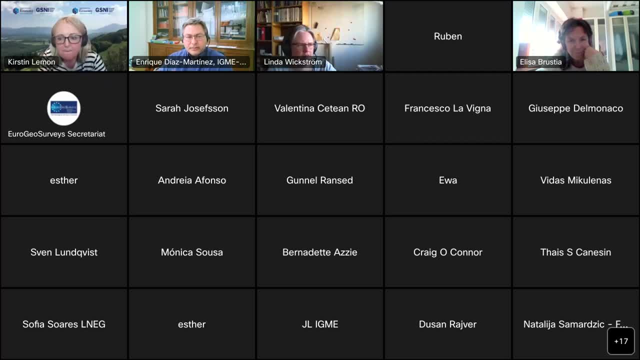 database we can actually mark out if a site is appropriate for education or for tourism or if it's just a pure scientific site- And we hope to, if we get money for a new project, that we can actually do some kind of automatic valuation of these aspects. So if you change, 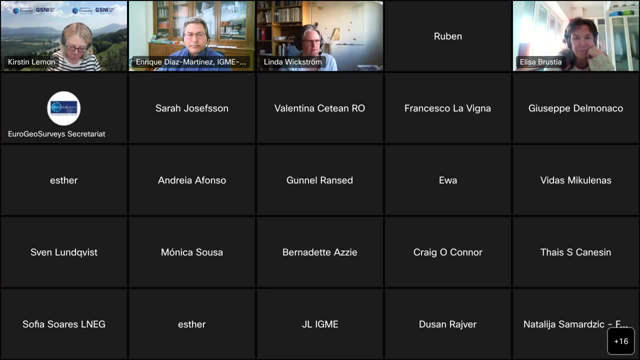 one attribute, for instance, it sort of recalculates Itself. Yes, So you don't have to do that evaluation again, sort of so to speak. But we'll see. Do you want to say something, Elisa? In your inventory, did you apply any of this, for example? 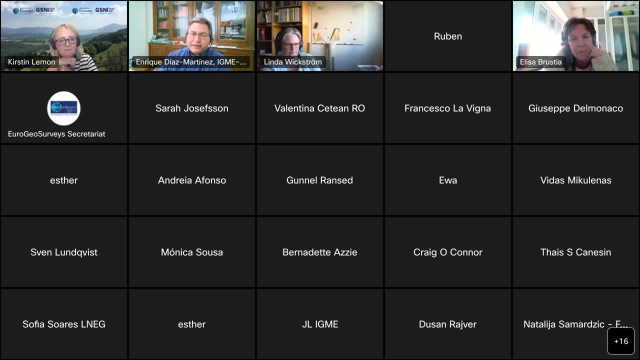 when you chose the areas that were going to be affected by the pandemic, areas that were going to be used for in mount vetore. uh, for the itineraries, or for the viewpoints, the, i suppose you, you get enough now. at this moment we we organized only um a course for a. 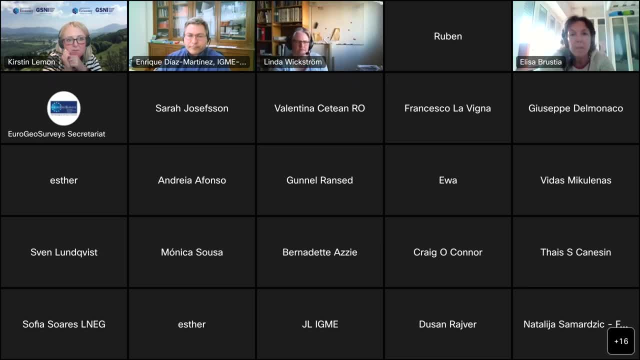 guide, for park guides, but for for people or for school or education. now still not in future is possible. we hope, okay, okay, well, i was also referring, maybe in the beginning, before you. you designed the, the areas where you would bring the tourists. i suppose you also um previously had to talk with the local authorities, for example, guides, the. 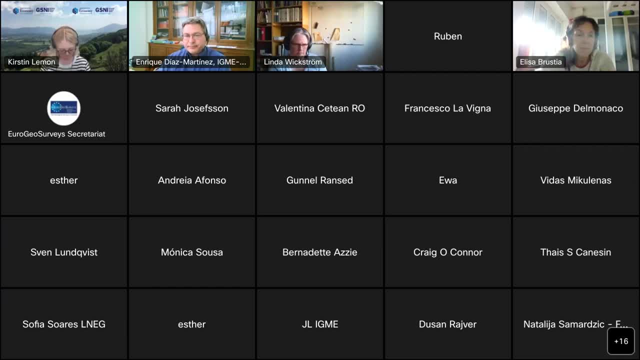 the guy the park guides must, must be something, something. okay, i don't know if. no, we don't have any more questions here. okay, so one. uh, i don't know if we are supposed to stop in four minutes. so, if any of you wants to make some statement or some recommendations for in conclusion, and then i will just finish up the 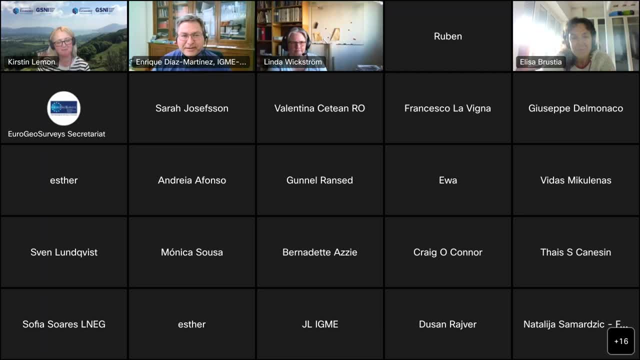 with some of conclusions. also, do you want to say anything else? okay, well then, thank you very much to all three. i think it was a great opportunity to hear directly from, uh, the persons that are working on site with the geotourism, with the help with the specialist. 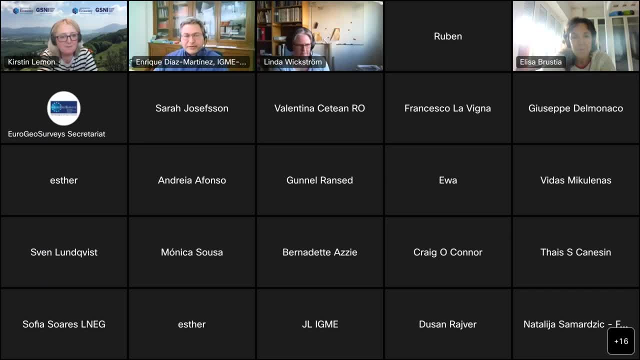 from people that work in geoconservation and geoharitors at the geological surveys. i think that it has been very obvious from the, from the conclusions of all three of the talks, that your heritage can contribute to local socioeconomic development. it is important for tourism. it is important also for the to be considered for the preservation of the sites.